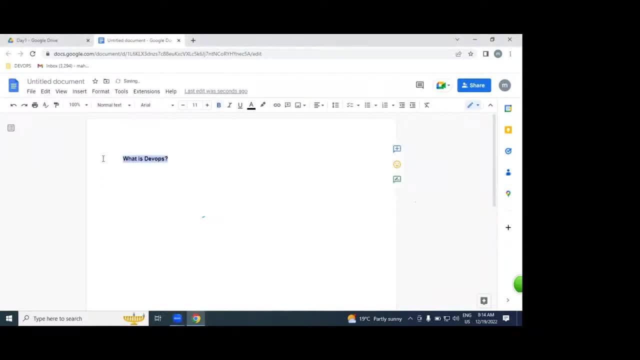 our focus is only for what? DevOps? What is DevOps we are going to discuss for today. In tomorrow, we are going to be discussing about what is AWS, What is AWS and DevOps versus AWS. So today we are focused on DevOps, Tomorrow, AWS and AWS versus. 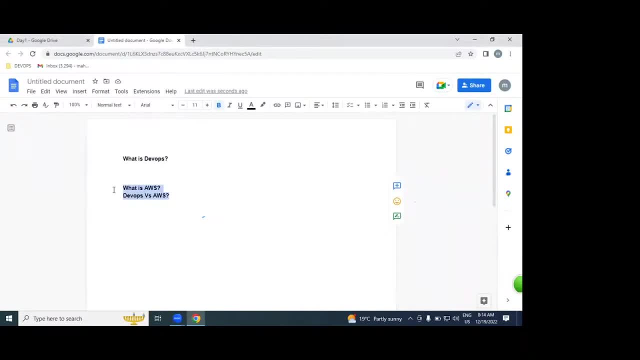 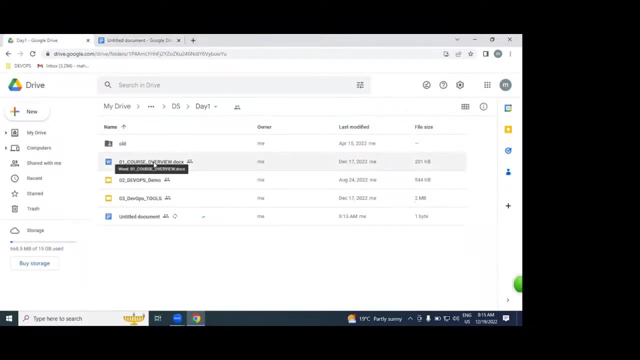 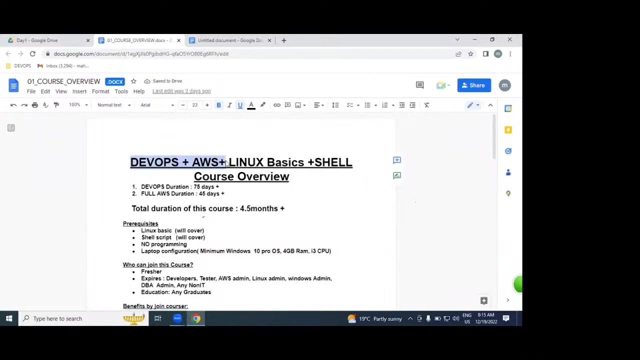 DevOps. That is in exactly tomorrow day. So, before starting the session, and let us course you, What is this course, What exactly we are going to do? Let us course you. So this course is designed with complete DevOps, complete AWS, Linux basics and Shelf. 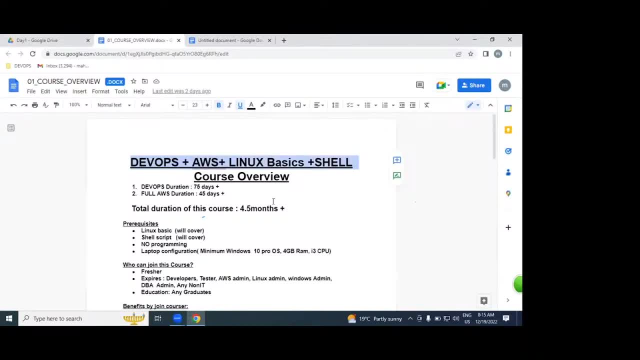 Security. So this four will be covered in this course. The total duration of this course is four and a half months plus, not as minus. It is less One week or two weeks plus or minus. It will take. total duration of this courses. what exactly? Four and a half months. 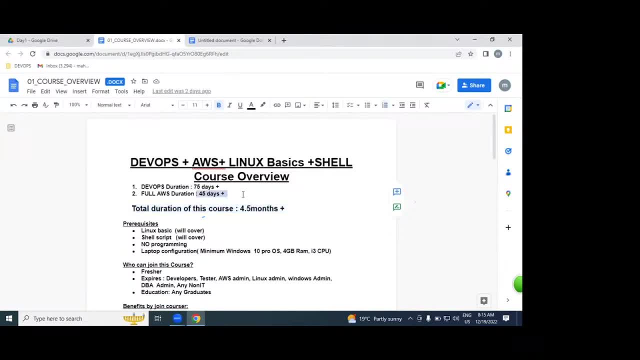 In that 44 days, More than forty-four days, are good for you. You just have to pay these more than 45 days we are going to be discussing ada place. more than 75 days, we're going to be discussing devops. it is a combo we can't separate. so if you want to join in this course, which are 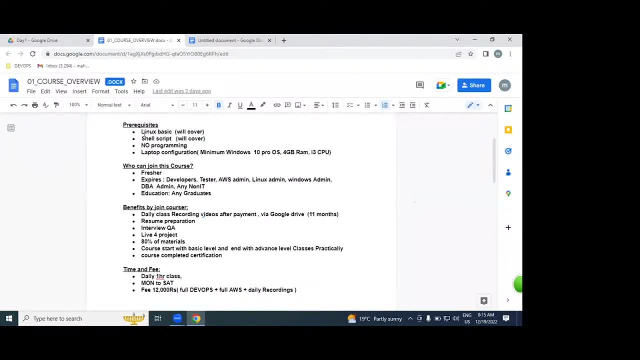 all the prerequisitions. so linux basics is required. if you want to join in this course, linux basics is required. that i will be covered, don't worry. linux basics, i'm going to be covered, don't worry. and shell script also. i'm going to become. don't no, programming like java dot net. 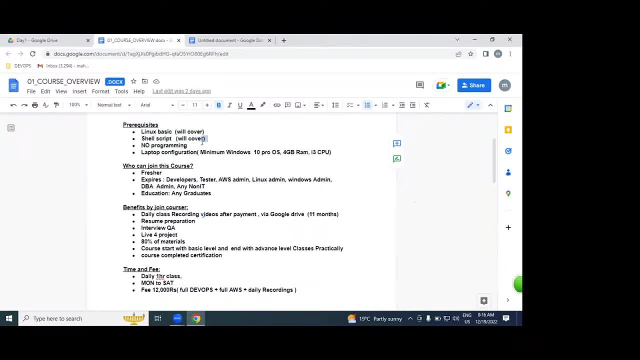 python, no programming is required. if you understand my language, english- it is more than enough. it is more than enough, please. laptop is required to practice every day, so minimum. so 10 pro windows, 10 pro 4 gb ram is minimum, but i'm recommend 6 gb. 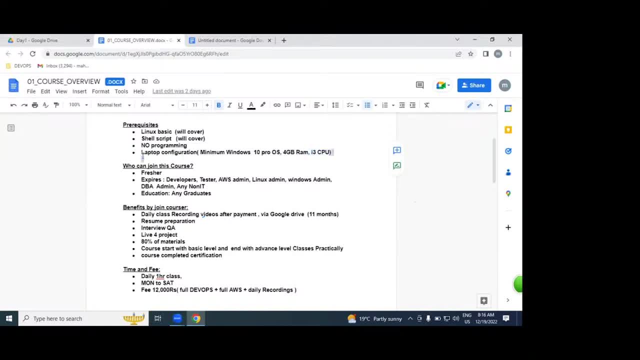 i 3 is minimum, so this is an exactly or laptop configuration. so who can join in this course? yes, freshers can join in this course. yes, freshers can join in this course. experienced students also can join in this course, like developers, testers, aws admins, linux admins, windows admins. 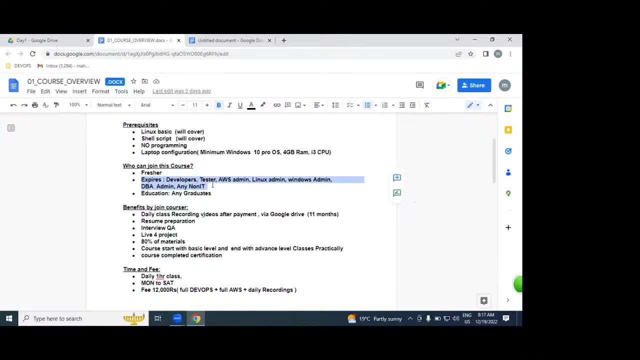 db administrators, any non-it like a chemical background, mechanical background, any degree possible. still, any non-uzu students also can join in this course. graduate any graduation. graduation is must ensure any graduate like btec công ty MBA or a basic computers any degree, any degrees. minimum qualification: 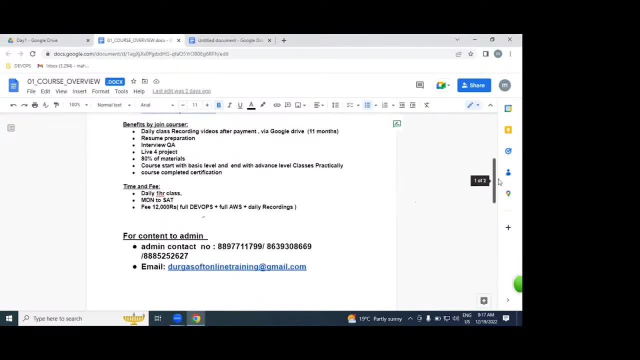 so if you join in this course, which are all the benefits. if you join in this course, which are all the benefits. guys, please just join in. you would be great, for weren't you? we could be Tiny Schulz Morehi's to help you with big time. 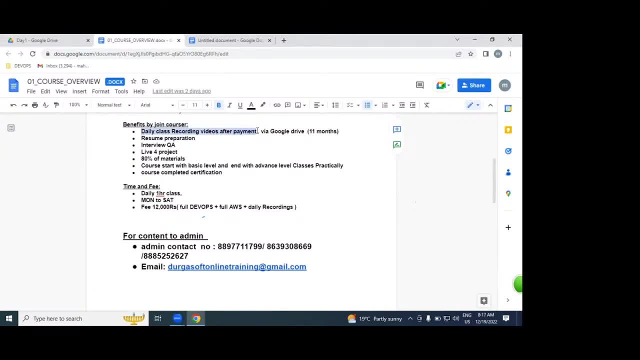 be provided once. if you payment done, you will. daily recordings will be received after this class. after this class, some students may remember, some students may not be remember. you got it very clearly- but after this class, by seeing this recording, you can able to practice. my intention is providing recording for practice only, not for saving somewhere else, for not. 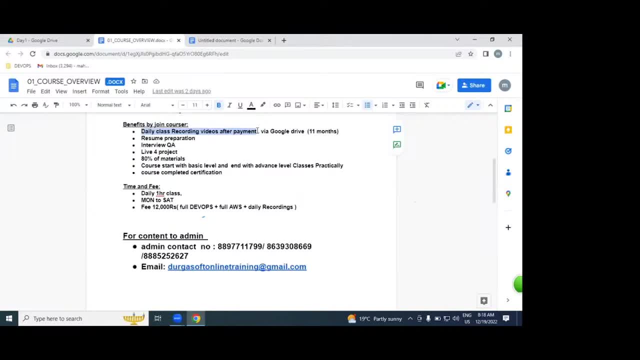 sharing. it is student helping only then, after reading, after attending classes, after watching video, after completion of practice. still, if you have any doubts and clarification, i can clarify in the next class. our motto is not attending classes and practicing. okay, that is very, very important point. resume preparation after completion of this course. resume preparation: 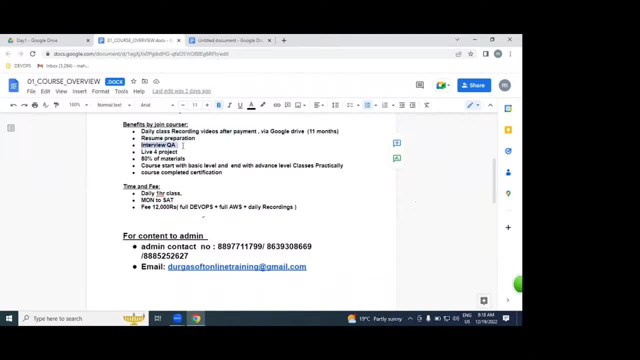 i'm going to be helping you. you entry, question and answers i'm going to be provided. okay, for live projects will be covered, including in this. in this duration, four and a half months. it is not a separate- don't expect any separate projects course, itself inbuilt. i'm going to be covering four live projects. 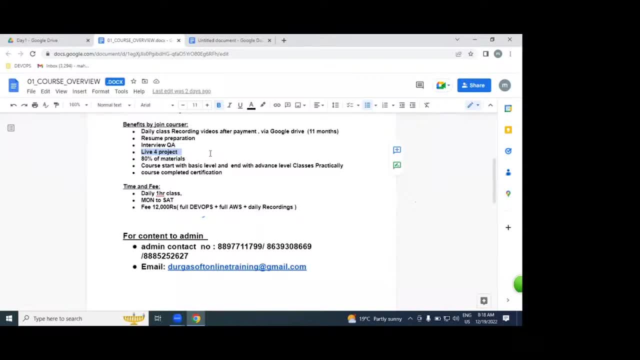 for example, ansible model, any model. so we're going to start with what exactly? basics, understanding to advanced, then end of the model. we'll do one project that is a model of our classes. okay, fine, eighty percent of soft material and provide not hard copy, soft copy. so our close, our classes are. start from where exactly? very basically each. 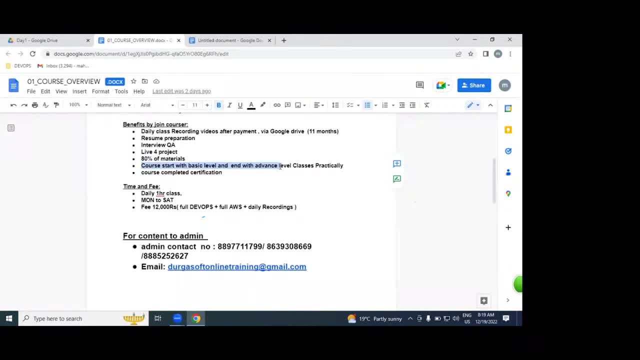 and every student can able to understand very easily, even non non-technical students also, and it's going to finish with an advanced advanced level. so each and every class gonna be explained theoretically and then it's going to be finished with an advanced advanced level. understand the concept. the same thing will be reflected in a practical on the same class. 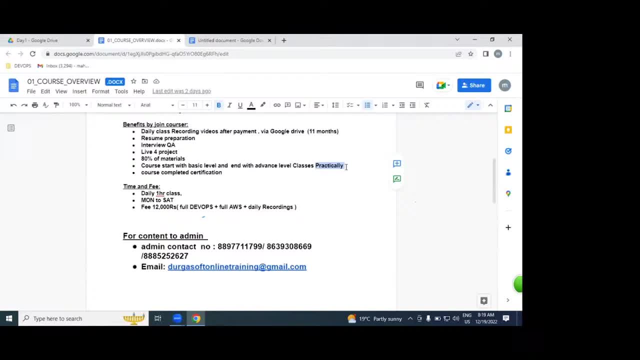 itself every day that you need to practice. you have to promise yourself: practice one hour for a class, minimum two hours. to practice three hours per day. you need to promise yourself before joining in this course and after completion of this course you will receive a course completed certificate for only freshers experience only. get it, but don't forget this certificate if you need another certificate. you will get a certificate for only freshers. experience also get it, but don't give up on the beginning of this course and when you get that certificate right, that will be there, so you will get a certificate as well. it is the same thing you. 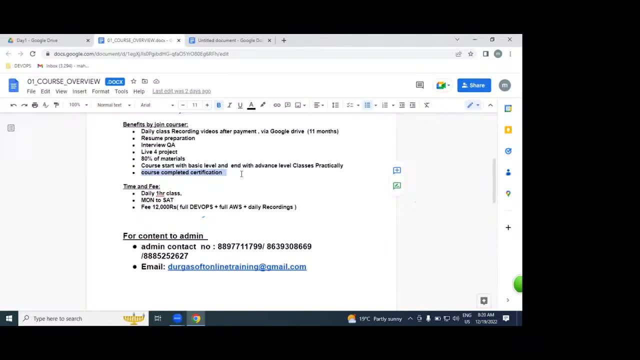 mention anywhere. you know very well what is that. got it very clearly. so, after completion of this course, you will feel 1.5 years of experience, a real experience. you can feel inside that you can manage, in your regime, that you can manage and after getting a job, up to three years or 3.5 to. 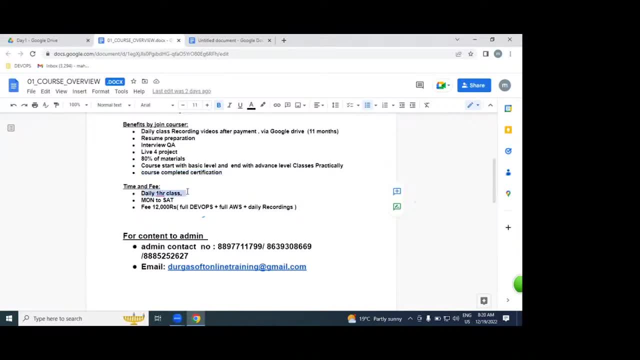 four years also? okay, fine, so daily you need to attend one hour class, it's enough, only one hour. after the class i will clarify questions and doubts. also, one hour is more than enough. one hour is equal to five hours per day. if it is increased 15 minutes, you're going to increase. 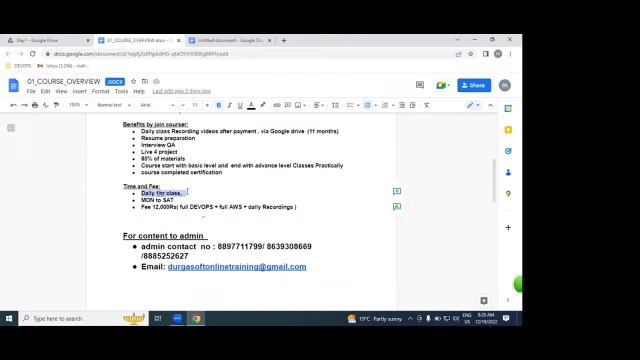 one more two hours, okay. so completion of classes doesn't matter. we can complete within one month also, but we need to practice. that is what one hour it will take, four and a half months duration. so our classes are monday to saturday. our classes are monday to: 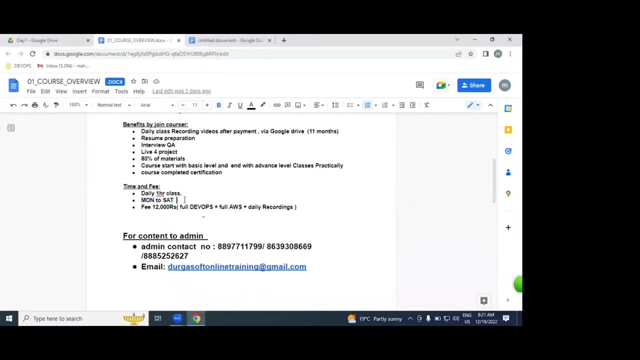 monday to saturday- sunday also sometime. we have baby monthly once sunday also, we have a session monthly once prior to one day. i'll inform you prior to one day if it is sunday, saturday or friday. i'll inform you whether we have a class this sunday. okay, so you are going to be paying 12 000 rupees fee. 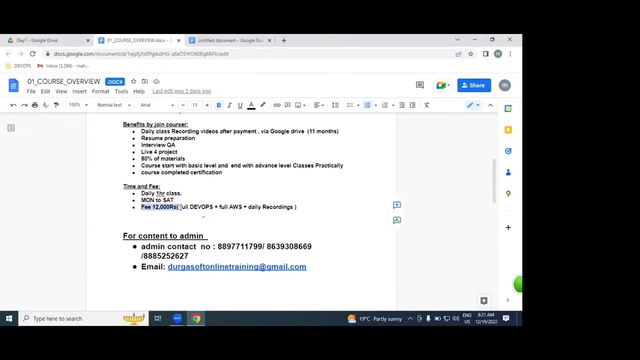 you're going to be paying 12 000 rupees fee: full devops course, full aws, not for introductorial way, full aws, full completed course and daily recording sessions also. you're going to be paying for what? daily recording sessions also. daily recording sessions also. 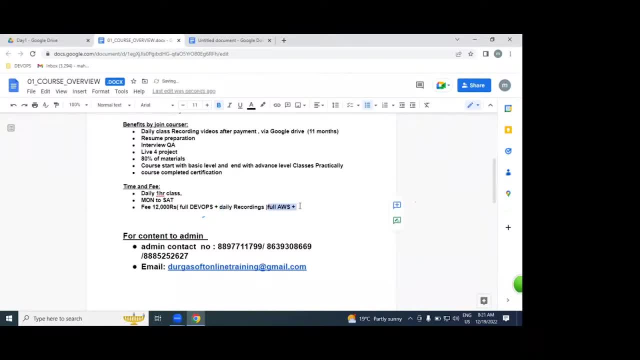 daily recording sessions. also, and if you want to contact with the redmond, please use this information. please use this contact or admin contact information. i'm going to be sending this information directly to the redmond. contact says: okay, going to be shared in the chat box online students. please be get it and make it somewhere else save. 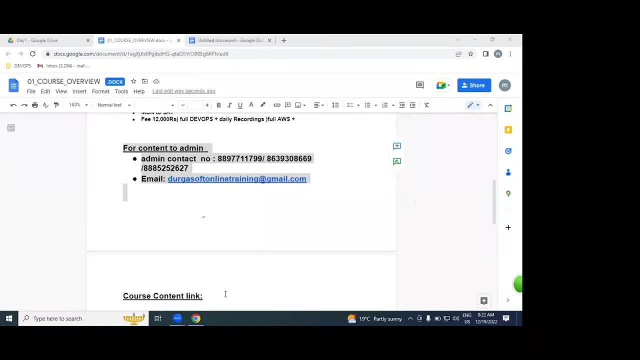 and what exactly. we won't be discussing for enough months what we are going. what exactly, guys, please course content link. we need to required or not? so i'm going to be shared this link: course content in the chat box. please be used there if you copy paste in any browser. if you copy paste any browser, that link 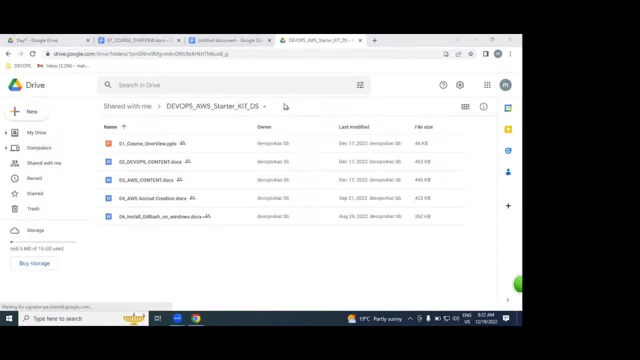 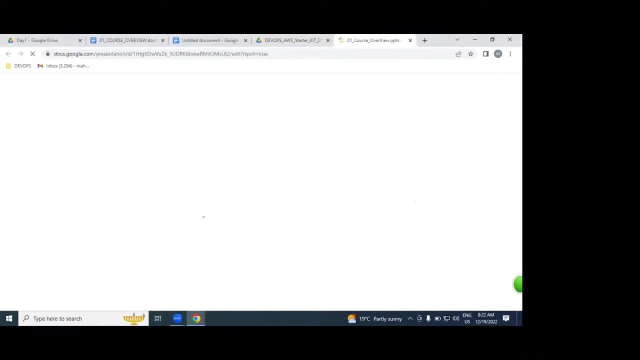 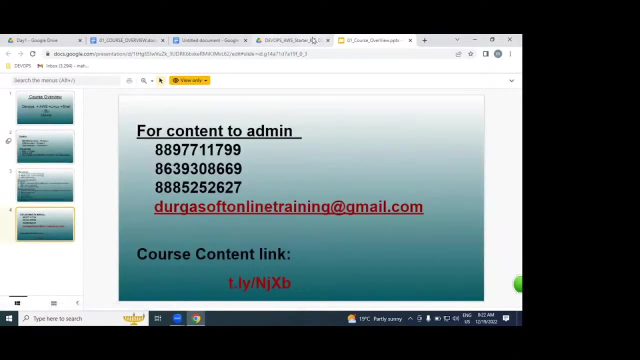 you can able to see the course content. okay, first one is: what first document is exactly? what is the course? how are you? what exactly? which you have discussed right now? same thing only, but after the class you know you can revise once again. okay, fine, the next document is the works content. 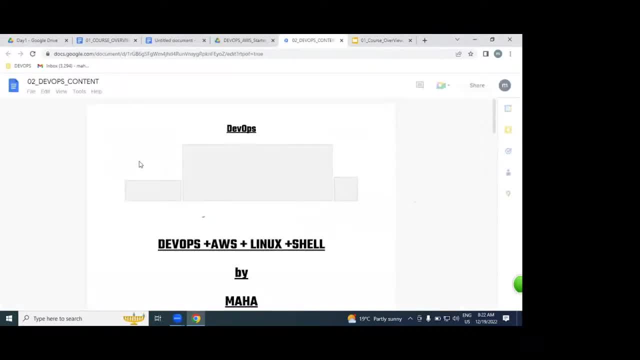 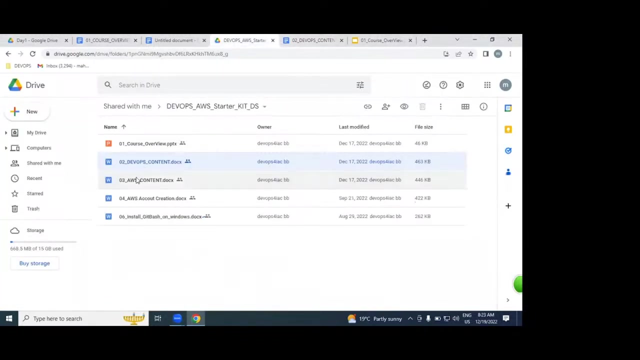 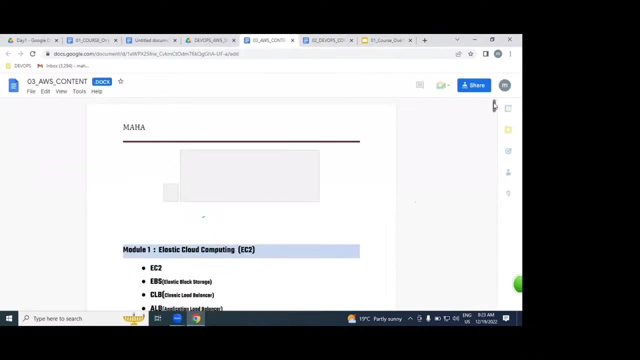 what exactly we are going to be discussing in devops. please look at once. it is totally around. maybe 20 pages of devops content, please. 20 pages of devops contents, guys, please, 20 pages of devops content, the same way. okay, we have a aws content also. we have a aws a content also. it is around, maybe. 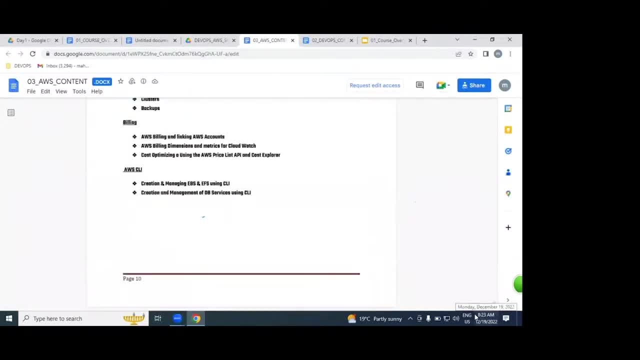 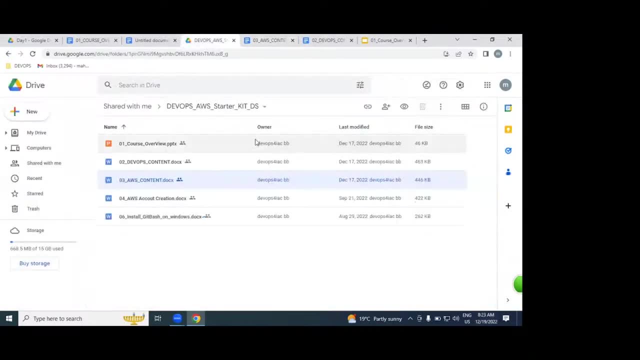 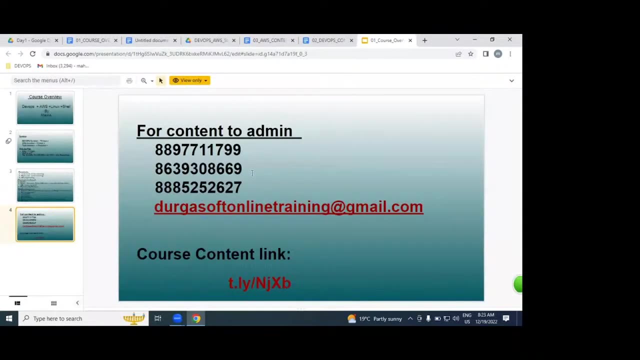 9 pages or 10 pages of content. please look at once after the session, please revise once these two documents what we are going to be discussing in the four and of months. so offline students, by end of the session you can able to take it and please ask me i will share it, okay. 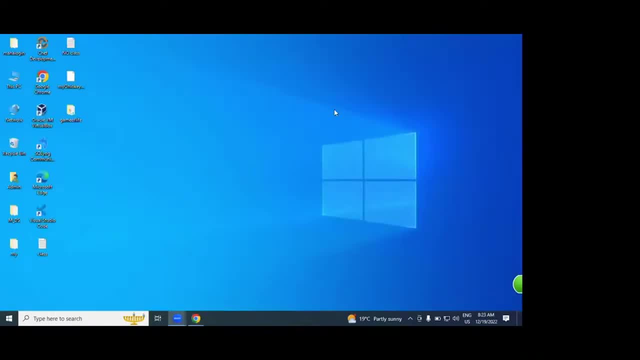 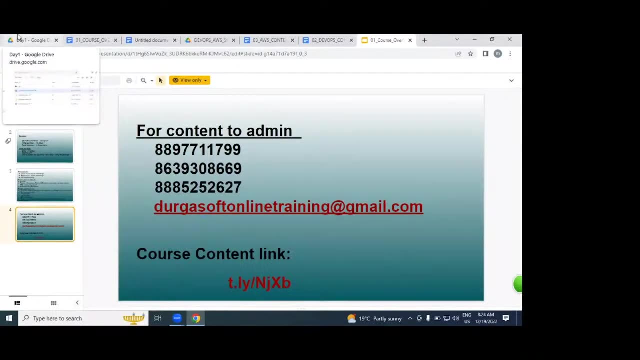 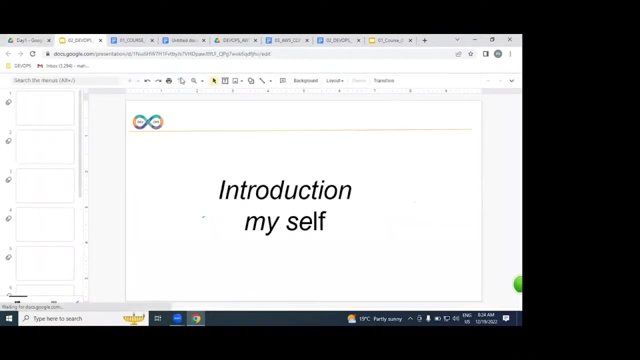 okay, okay, okay. So this is an exactly course. who are you? course, who are you? shall we start a demonstration? please? shall we start right now? so first let me introduce myself. my name is Maha. my name is Maha. I have totally 15 years of experience in MTA. my career starts as a Java. 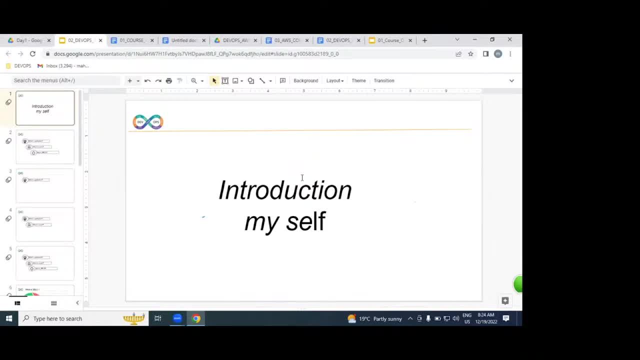 developer, Java developer. then I turn as a DevOps engineer, as well as with AWS and Azure. from last five years onwards, last five years onwards, I'm working as a DevOps engineer, senior DevOps engineer. that is in exactly my profile before starting this. so I have three. 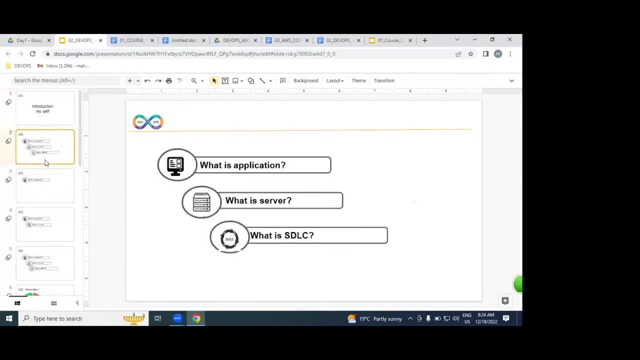 questions I'm going to be asking. please answer to me. what is an application? first question. the second question: what is a server? the third question is: what is SDLs? please answer to me what is the first question. please at least read out. please reply what is the first question. 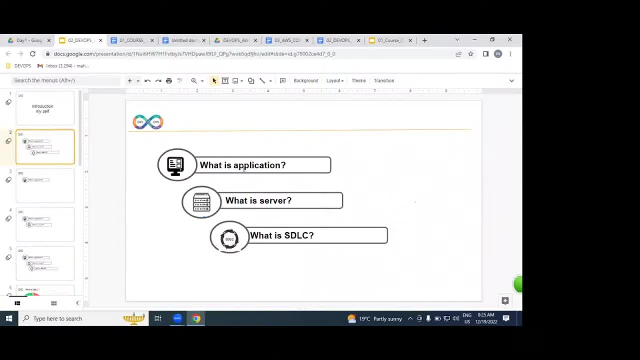 please just type in the as it is. what is the question, please? what is application? just type it in the chat box, guys, please, all of you. what is an application, please? application is nothing but a website. 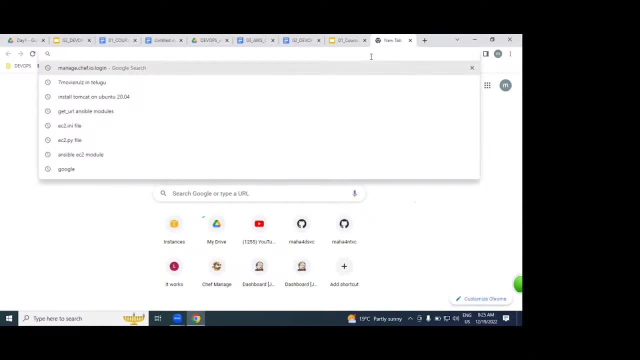 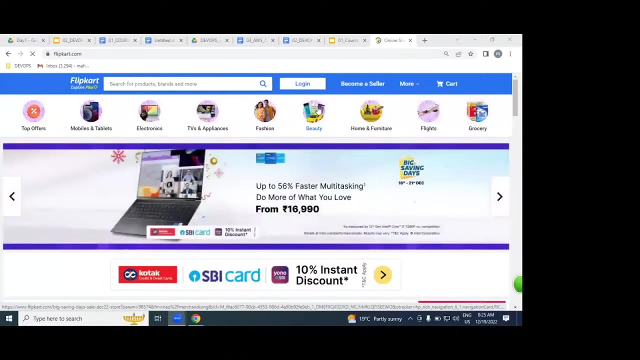 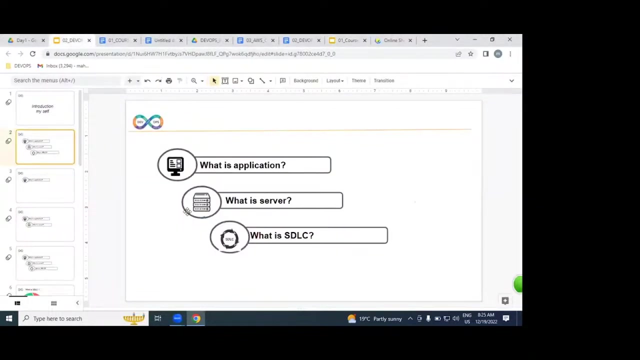 application is nothing but a website like a Flipkart website, like a Flipkart, like a BookMyShow IRCTC. these are all we are calling as what application? so, if you ask me definition point of view, if you ask me what is an application, 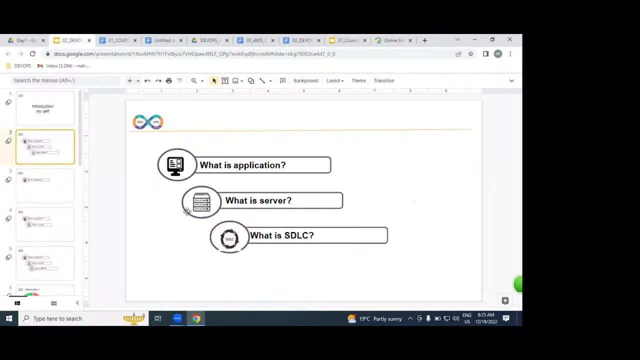 if it is, ask me, definition: the working software, the working software which is written, any programming like Java, NET, Python, any programming, any programming we call as what application? so let me repeat one more time: what is an application, please? 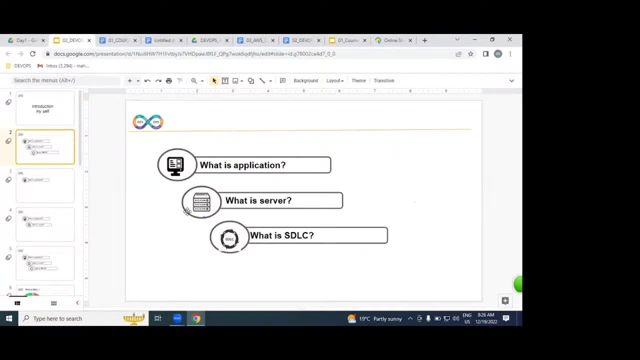 the working software which is written, any programming language we call as what applications? am I right or wrong? so, after we have a developers or not, have you heard about Java developers, NET developers or not? after writing the lines of code which you are calling a software, the software we are going to, 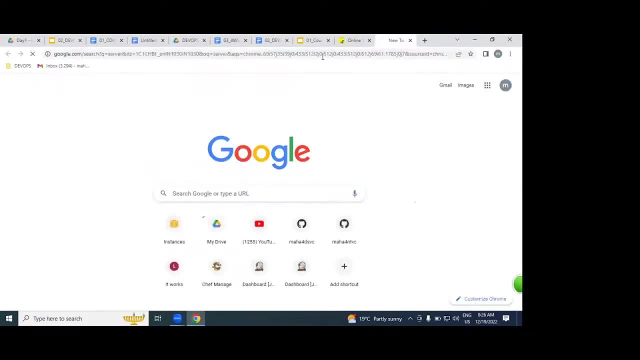 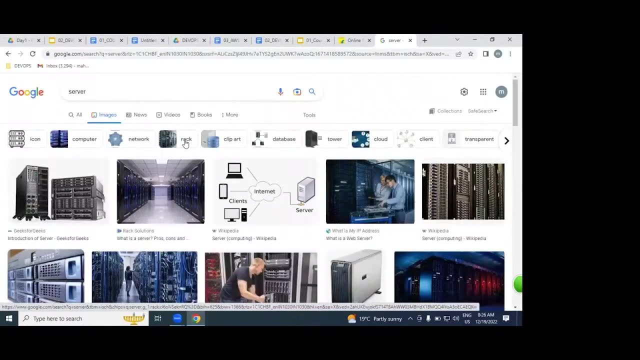 be placed on server side. we are going to be placed on server side once. if it is placed on server side after writing software, the software is going to be placed on where- server side. then, there itself, we are going to be accessing what exactly as a website. 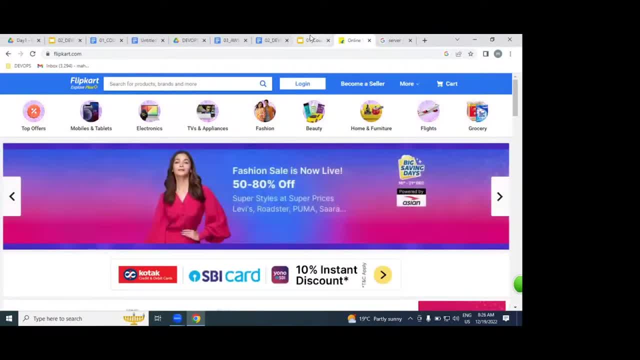 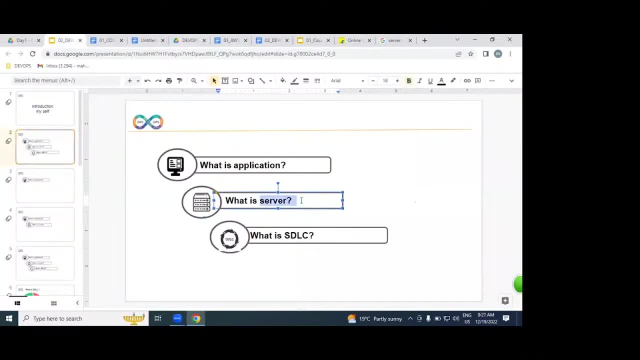 got it very clearly. so what is an application, the working software which is written, any programming language, that application we are going to be placed on where exactly? on hundreds of servers, once, if it is placed, once if it is placed, a Java application on server side. 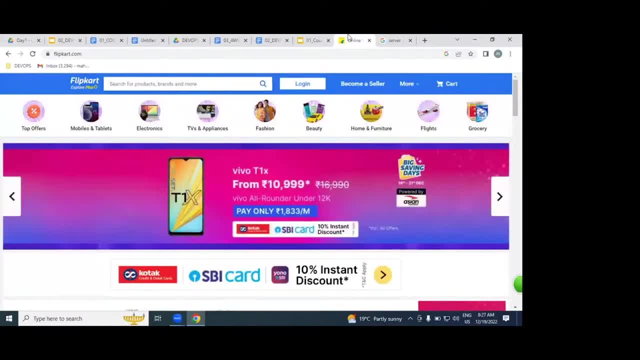 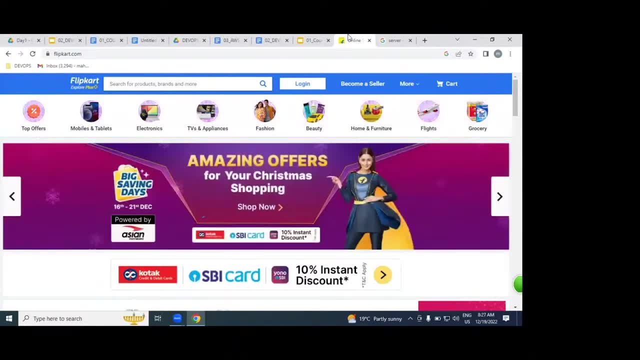 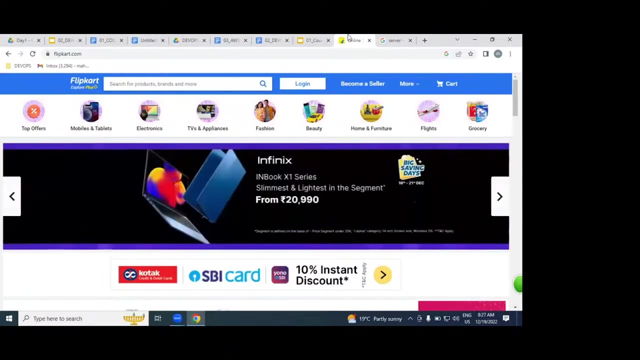 then there itself, we are going to be accessing over internet as a website. as a website. got it very clearly. what is an application? do you understand? what is a server? also, server for what? for maintaining our applications, for deploying our applications. but what about? next question is pending guys, please tell me. 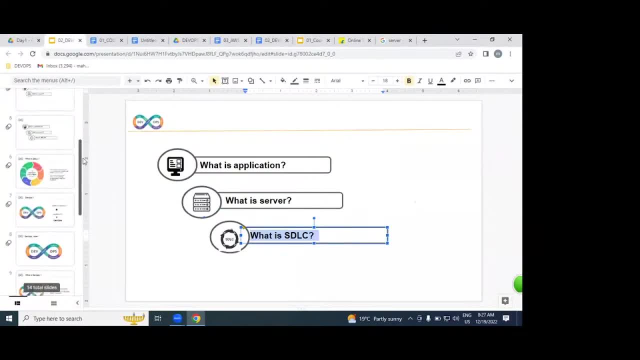 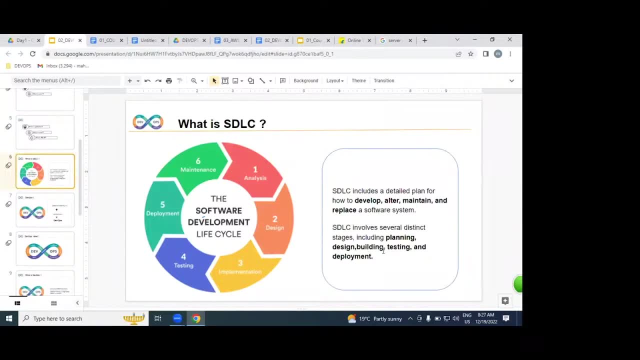 what is SDLC? so, what is SDLC, please? how many people aware of this? how many people know about this? online students can able reply. how many of you know about this? how many of you know? how many of you don't know? 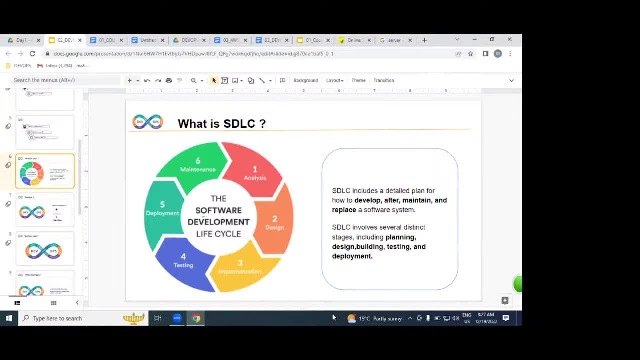 can you reply please? if you know, say yes, sir, I know it. if you don't know, so no, I don't know. can you reply in the chat box? all of you. can you reply, guys? please, all of you. what is SDLC? 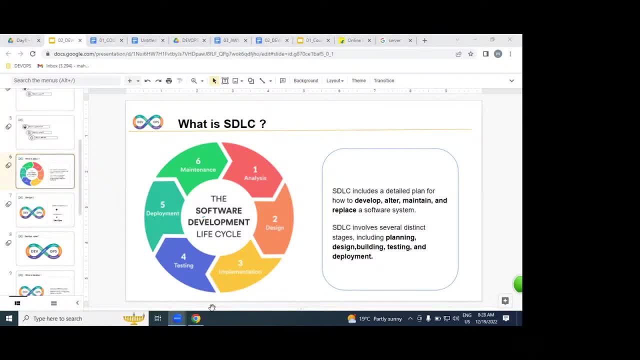 who knows, who don't know, because if you reply, I can explain more about this. everybody knows it, we can move forward. that's it. that is the reason I think somebody knows, somebody don't know. but let us discuss about it. what is SDLC? guys, please? 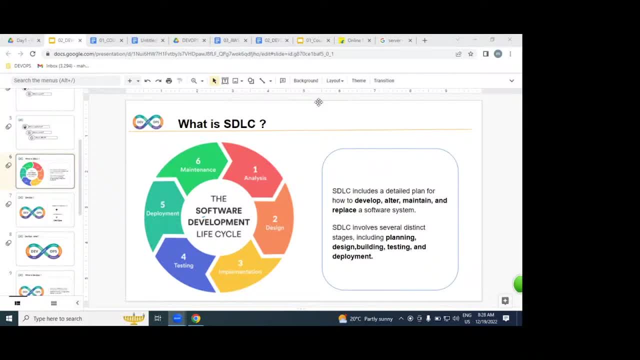 SDLC in the sense of what software development life cycle? SDLC is nothing but what software development life cycle? by using SDLC, by following SDLC process, by following SDLC process, we are going to be produce a software by end of this SDLC. 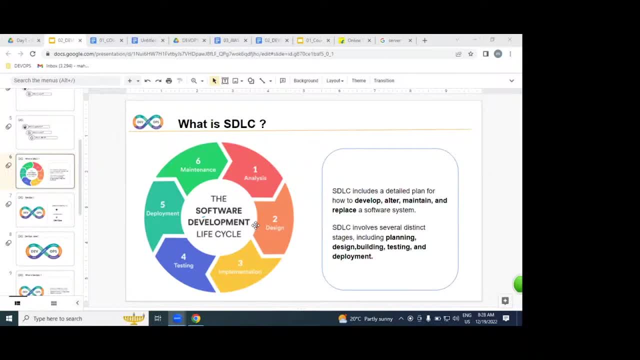 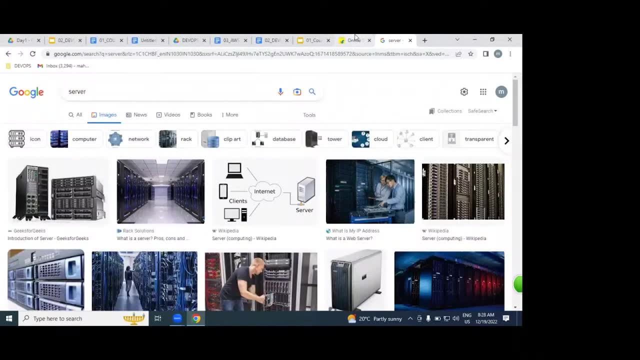 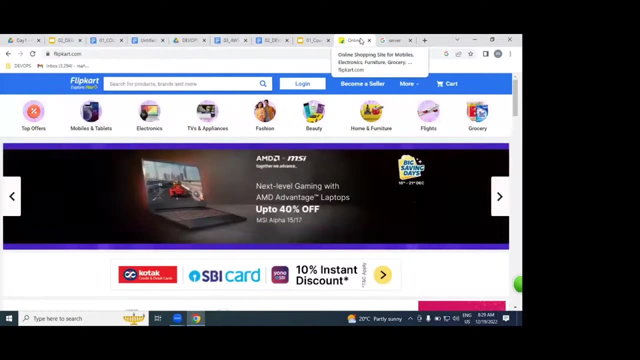 we can able to produce a software. the software we are going to be placed on server side. then we are going to be accessing as what application understood very clearly in SDLC. in SDLC we have a several stages and several phases. 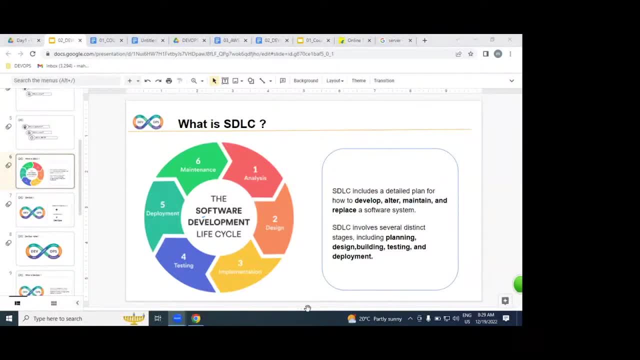 several stages and several phases. in SDLC, we have a analysis, design, implementation, testing, deploy and maintenance. we have a several stages and several phases. several stages and several phases. so let us understand what is this role. let us understand. let us understand what exactly. what is role? the phases and stages. 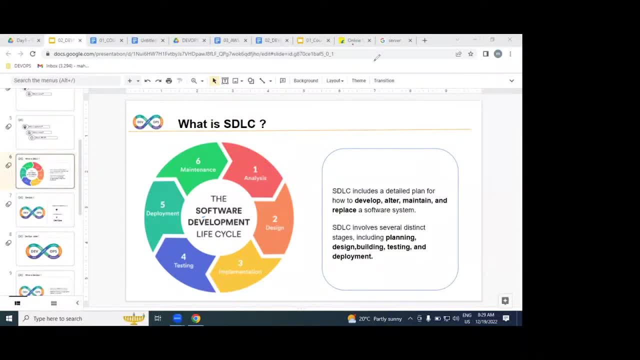 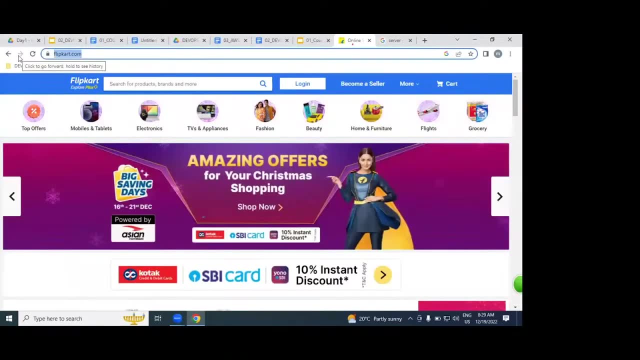 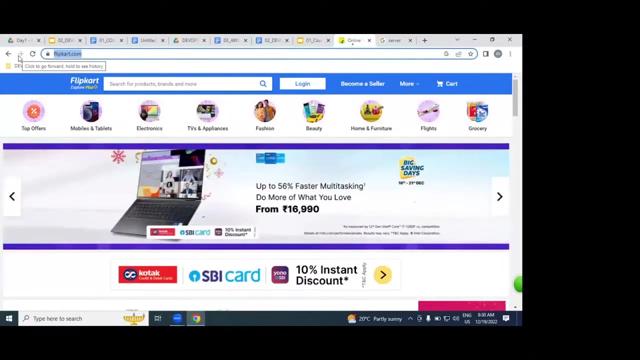 for example, I want to build a flip code kind of applications. I want to build a flip code kind of applications can able to build this overnight, within a day overnight. can able to get this flip code kind of applications? please tell me. 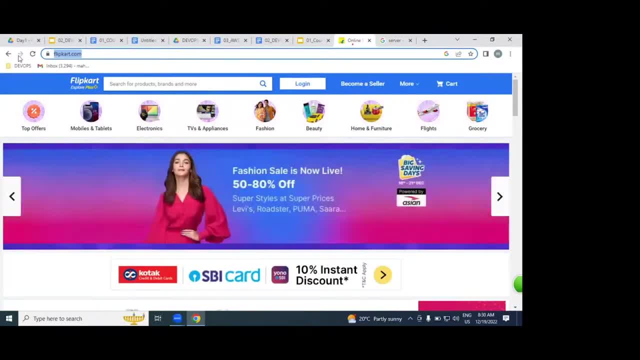 no, we can't build. so I am going to be asking you one more question, please answer to me: can able to build a apartment overnight, within a day? can able to build? no, the same way, we can't able to build our websites also. 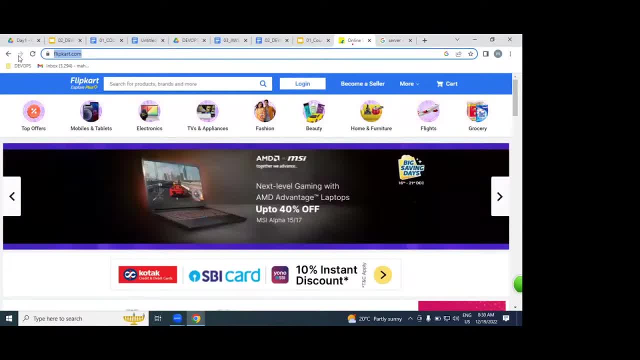 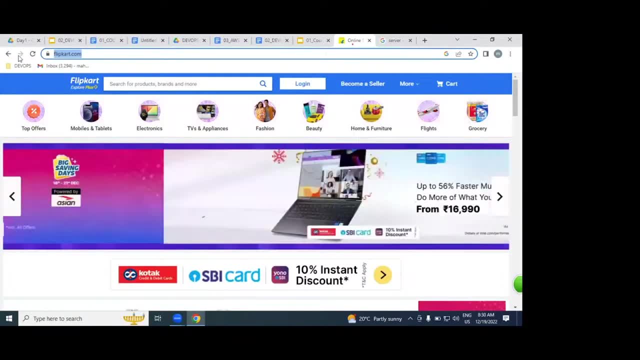 to make an application, you can add a new CRM, you can timestamp and any commissions that you like to short-term. the same way, we can't able to build our websites. also, if you want to construct the house, we need to follow so many stages and it will take six months, sometime one year also, we need to follow. 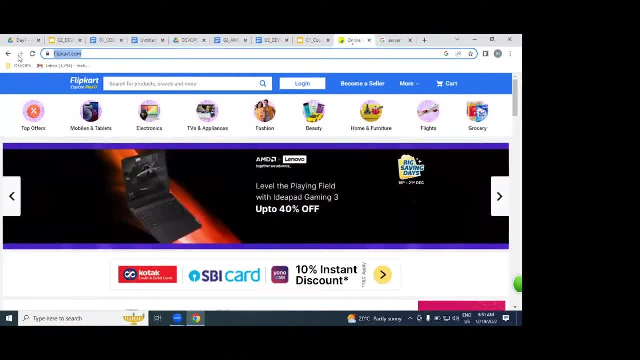 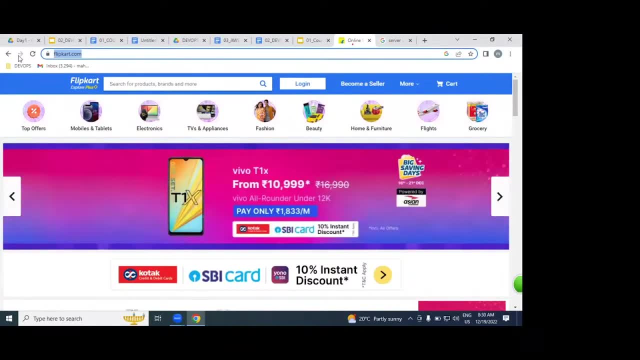 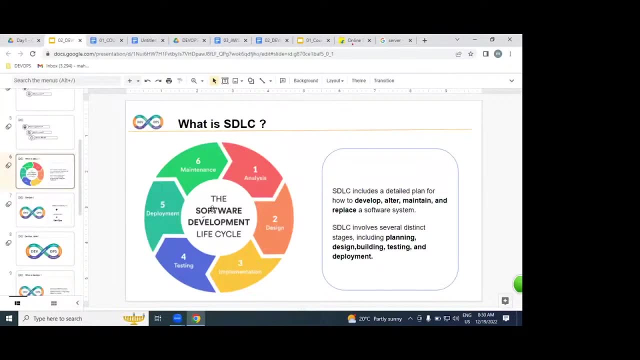 so many stages, then only we can able to complete what our apartment or home, whatever, the same way, our website also, if you want to construct, if you want to build this flipkart kind of applications we need to follow. these are all the stages. what are the first stage, guys, please, analysis, analysis. 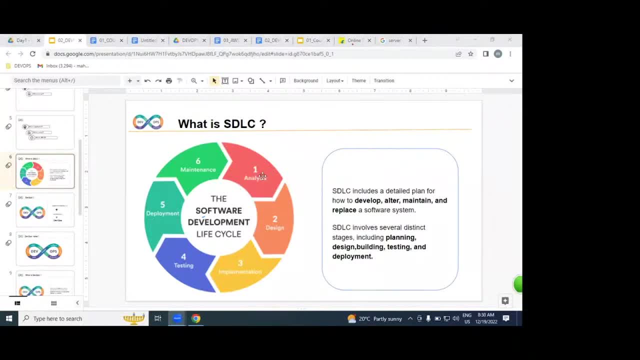 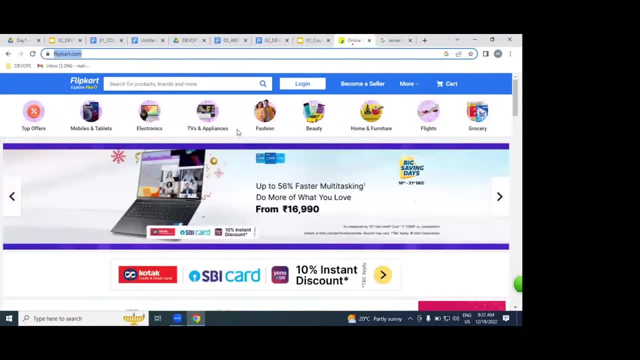 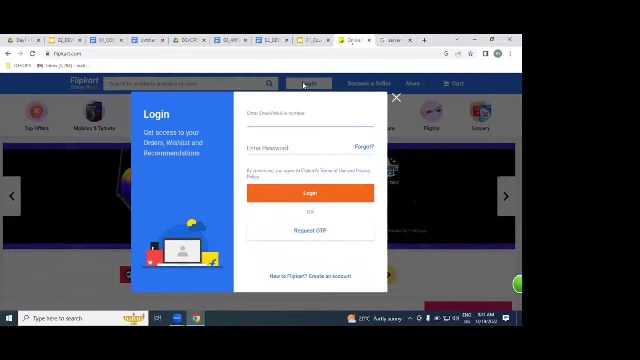 analysis is nothing but what: gathering information from the client. who is the client here? flipkart? what exactly this business? so whether it is required, how exactly login page? how exactly registration page? what is the payment gateway? what are the search page? how exactly tracking customer? each and every information. 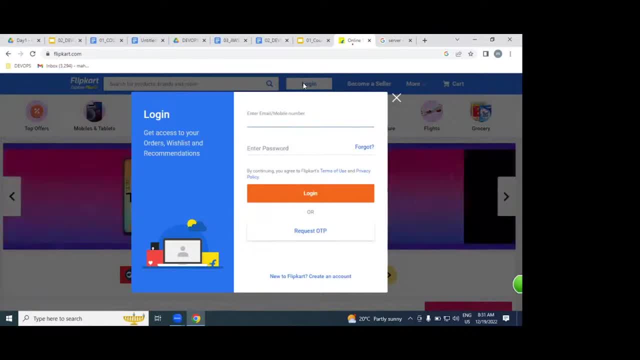 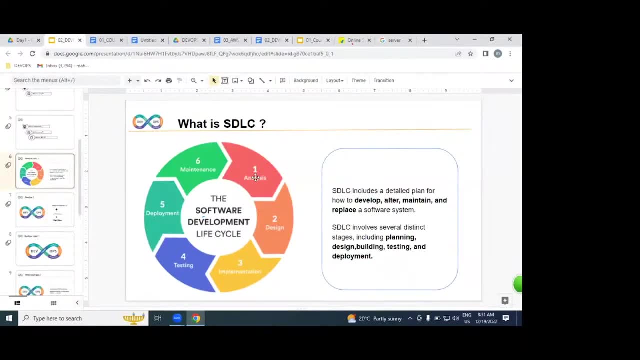 will be gathered from the client based on gathering information, based on gathering information, based on gathering information. so our architects will be designed. design is nothing but what plan? design is nothing but what plan. according into the plan, according into our plan, our developers will write the code. our developers will write the code, either maybe java code or dotnet or python, any programming. 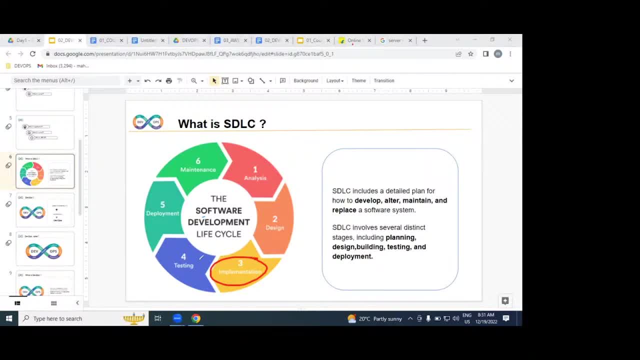 our developers will implement the software. but whether the software is in working condition or not, our testers will be verified by using selenium test cases or automation test cases, performance cases or manual test cases. our tests will be verified once if it is verified. so we are going to be deploying on hundreds of servers. so we are going to be deploying on hundreds of servers. 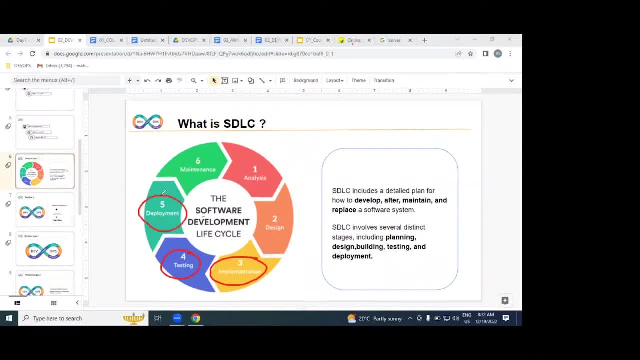 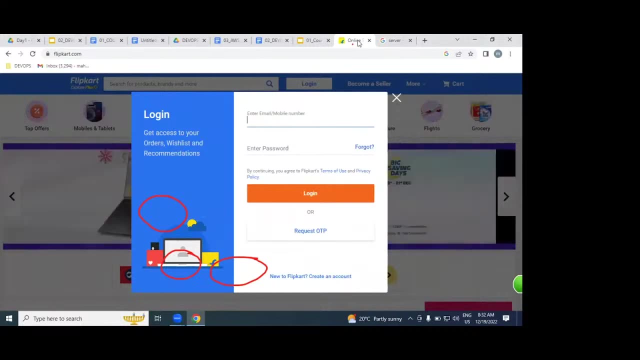 we are going to be deploying on hundreds of servers. Once if it is deploy applications on hundreds of servers, we can able to access our internet as a website. Once if it is. once if it is an access- access, no, whether this application is in working. 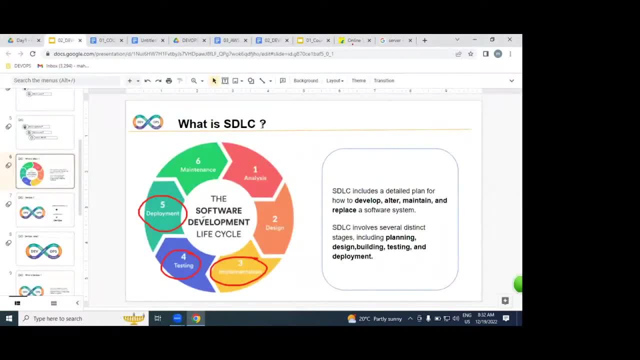 condition or not, we are going to be monitor and maintenance, monitor and maintenance. This entire process we are calling is what? This entire process we are calling as what? SDLC, SDLC, In this total process. so we have a developers, we have a testers, we have AWS administrators. 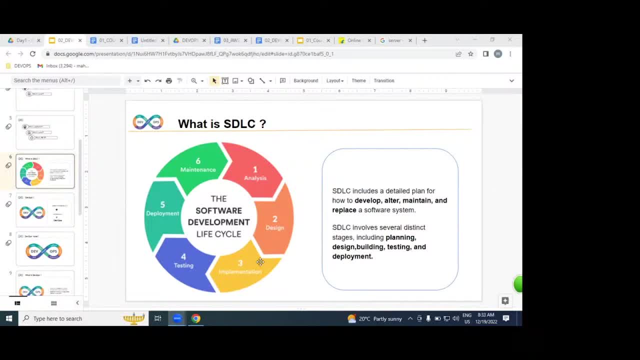 we have a Linux administrators, DB administrators. If you are an IT profile, if you are doing an ID, job or any profile, any platform, you are part of this. SDLs Including DevOps network. If you are working in IT software, you are part of this. 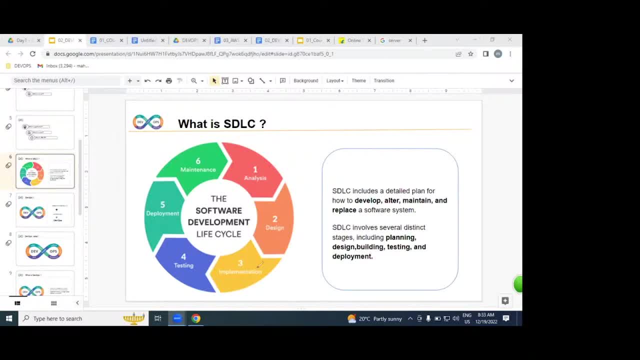 Maybe developers are working on where Developers are working on where exactly In implementation part Testers working on? where Are DB administrators, DevOps engineers, AWS engineers, LRX administrators- all together? we are going to be working in SDLC. 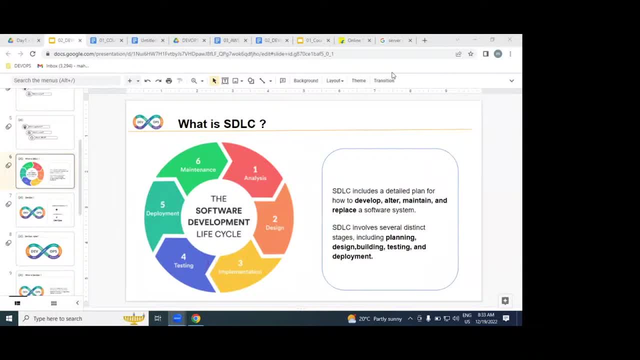 By end of the day. by end of the day, we are all not a DevOps engineer. we are all either developers, including AWS engineers, DevOps engineers, Java developers, NET developers, or we are all together. we are going to be involved in SDLC. by end of the day, we are 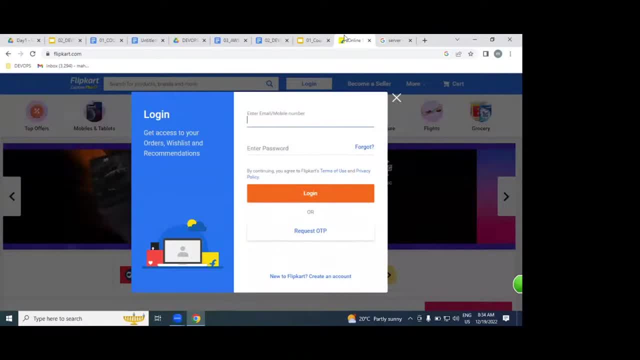 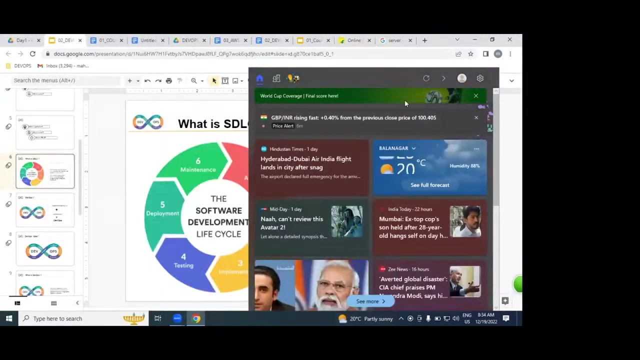 going to be produce a Flipkart kind of application, A Flipkart kind of application, Understood very clearly. I hope you people are understand What is SD, what is SDLC? I hope you people are understand very clearly. On top of SDLC, on top of SDLC, we are going to be implementing DevOps process. 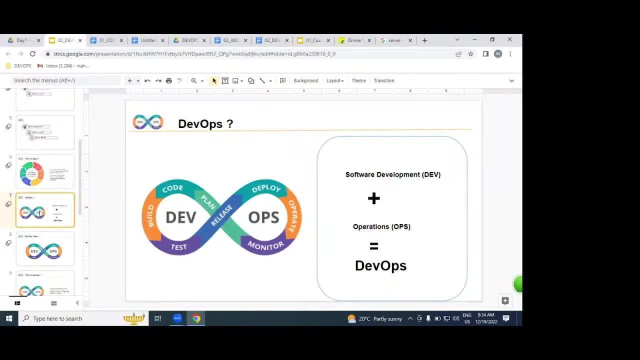 On top of SDLC, we are going to be implementing our DevOps process. What is Dév guys? please Come and talk сейчас. Dév guys representatives, Welcome to FL. Welcome to Dév guys representatives. The dev is nothing, but what development? dev is nothing but what development? OPS is nothing. 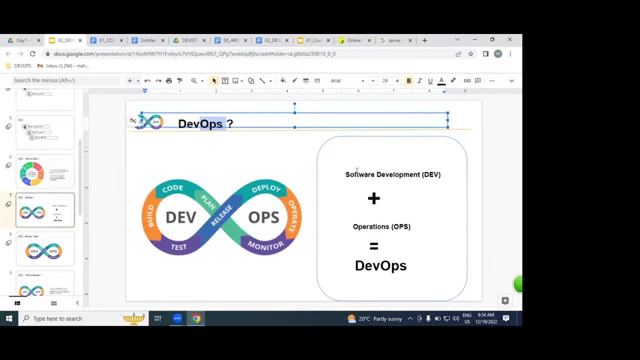 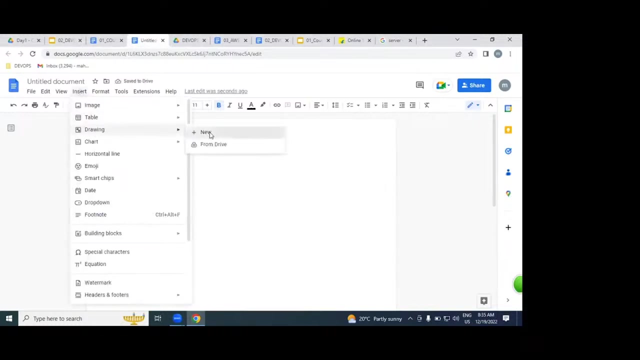 but what operations, the combination of software development plus operation we call as what dev OPS? we call as what dev OPS, guys, please, for example, let's say, let's say, for example, in SDLC we have a several stages and several phases, which you are already discussed am. 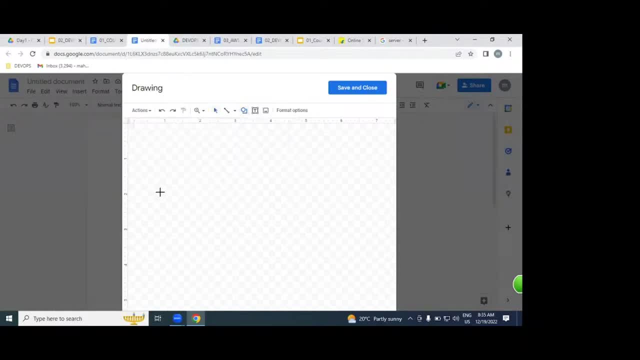 I right? yes, just in assume. so our SDLC, we have a several stages, am I right? so we are writing script if we say it may be developers are working here, maybe testers are working here, maybe it is a production. it is live. this last one is what life it is. 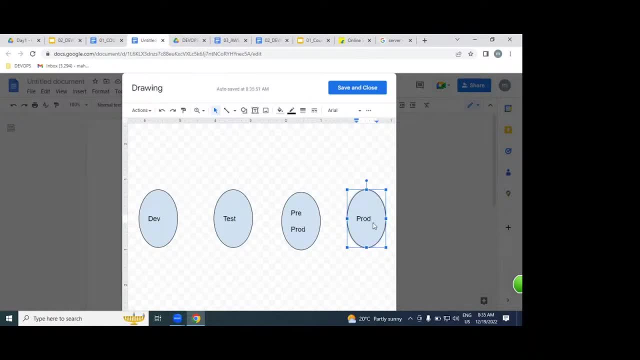 a live project product. so these are all the stages. we have guys, so many we have while writing scripts. so developers are going to be writing from where exactly in dev Meinung it by using java code, then what exactly it is moving into the testing environment. after verifying testers, we're going to be moving into the production: pre-production to the production. 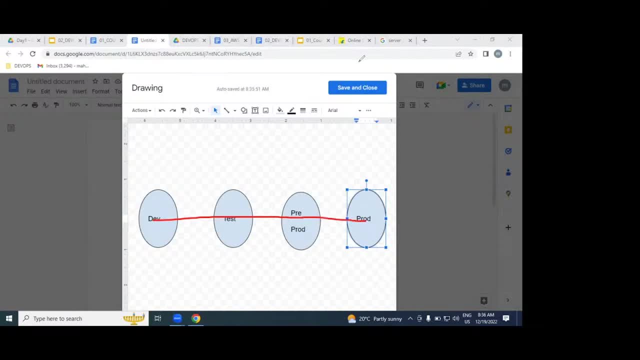 into production to the production. but my point is what exactly i'm going to be discussing with you, guys, please? so, as a devops engineer, our roles and responsibilities start from where dev environment ends with, where exactly production is nothing but operations, guys, please. so as a devops engineer, our roles and responsibilities start from the environment. 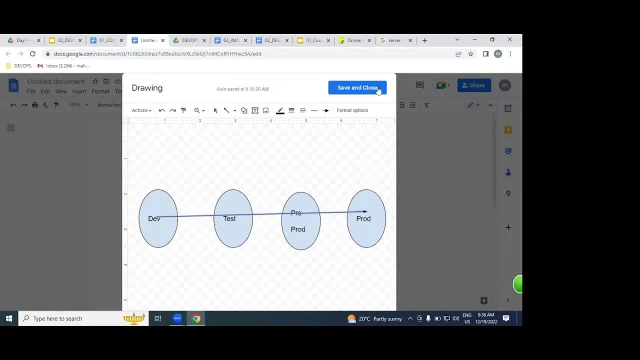 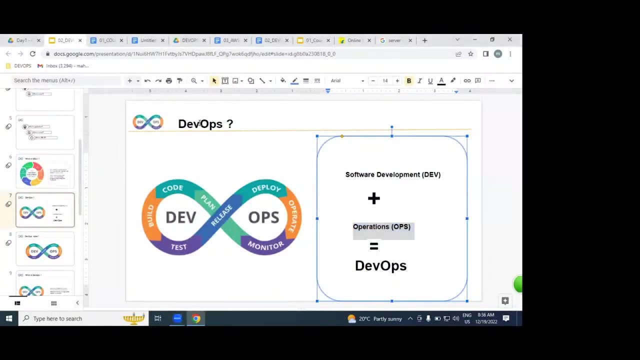 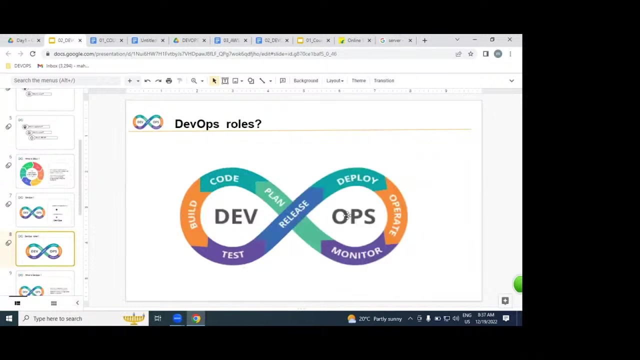 ends with operations. that is what exactly point i want to discuss with you. yes, so div is nothing but what development, ops is nothing but what operation, the combination of software, development, place operation we call as what, the webs we call as what develop. that means our roles and response. 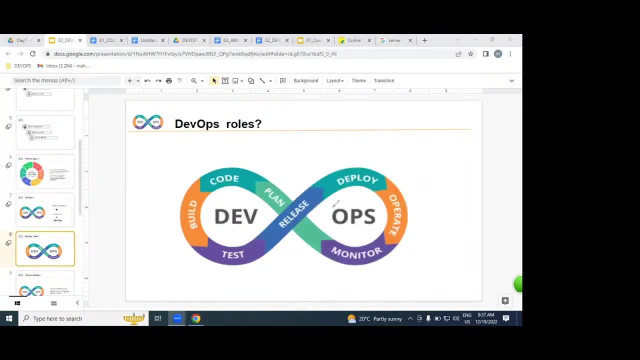 ability start from where exactly dev environment ends with operation. that means we are part of dev environment: build, test, release, deploy operation and monitor. so these are all the stages we are part of, but to be frankly, to be frankly, to be frankly, we are not writing any coding, sorry, 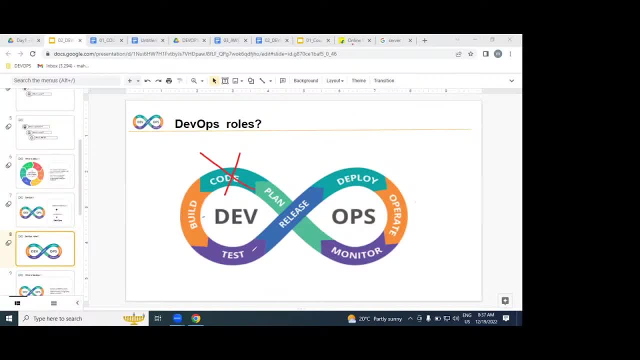 we are not writing any coding, to be frankly, we are not writing any test cases also. so our job is just: we are gonna be implementing here'sSpe, colt boss. so our job is just: we are gonna be implementing, just, we are going to be a implementing devops process from where dev environment to operations. 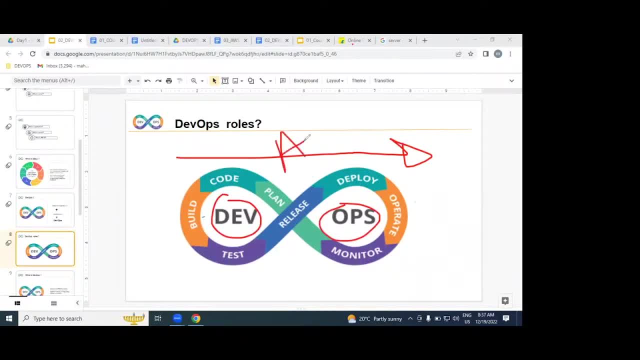 with an automated process. with an automated process. with an automated process is nothing but what device is nothing but project-based. the process is also is nothing but today's program. that's our products. is our cyber security that we are trying to solve. is this private project with us? 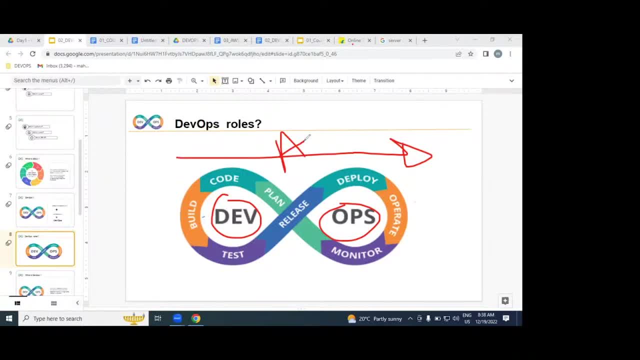 watch the palestineALL application website. the project biji is working in rome, taking the solution to build up a system called firest cope. that was opened at strategy. so, Strawberry, it will be appelied, you go around the, but what devops in? so, for example, developers are writing a code, the line software, the software. 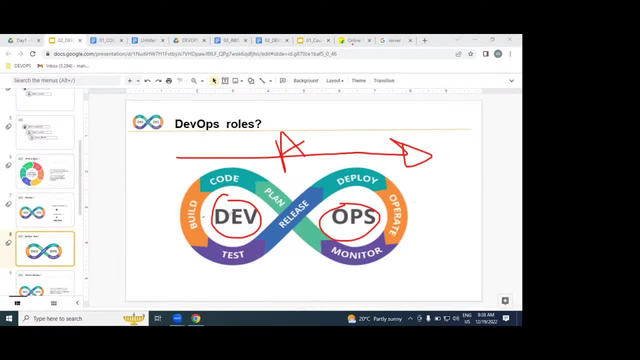 the software is going to be moving into a production environment with an automated process. that automatic process is going to be created by devops. that is only role we are going to play. in sdlc there is developers writing a code, testers are writing test cases. db administrator working in. 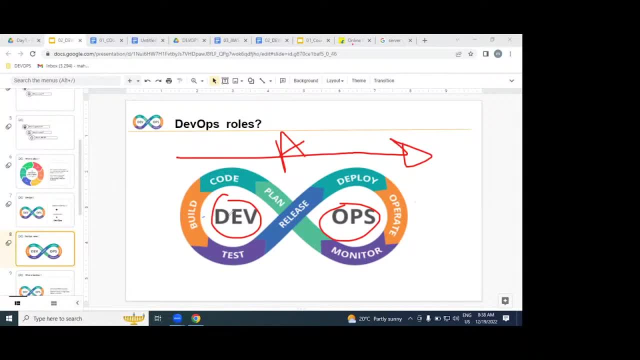 db admin, the aws administrator working on aws- the- all the people will be together. we are going to be complete our sdlc process in top of sdlc process. as a devops engineer, we are going to be implementing a, an automated process. so, if you are implementing an automated process, what will 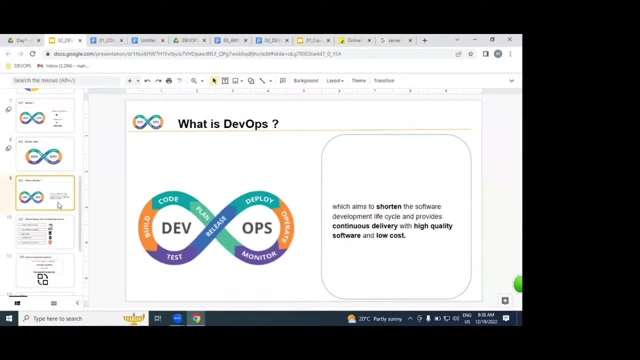 happen. what is in exactly devops? anybody help me? what is the devops? devops is a technology like javanet. no is devops is a technology like a javanet, it is known. devops is not a technology. devops is a process. devops is a process which we are going to be implementing from dev environment to 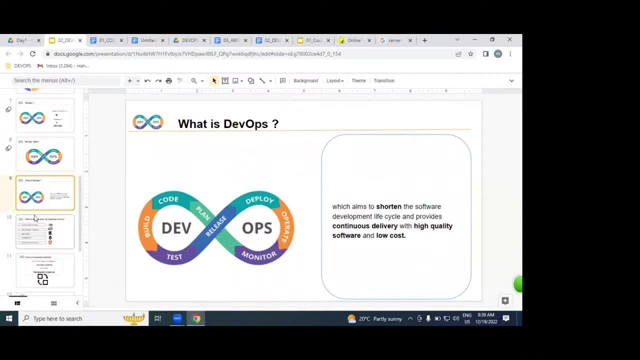 operation with an automated process. if you are implementing an automated process, we can able to deliver the software within a shorter step, as soon as possible. we can deliver our development developer software into the production environment. if you are delivering within a shortest time and the cost is going to be reduced, we can able to reduce the cost and we can able to provide highest. 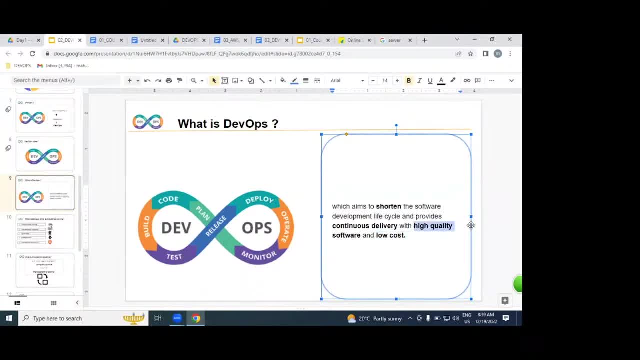 quality, highest quality. understood very clearly what is the devops? let me repeat: devops is a process which we are going to be implementing from where dev environment to operations. while delivering development, developer code into the production environment, we can able to deliver within a shortest time with the high quality, with low cost is nothing but what devops process. 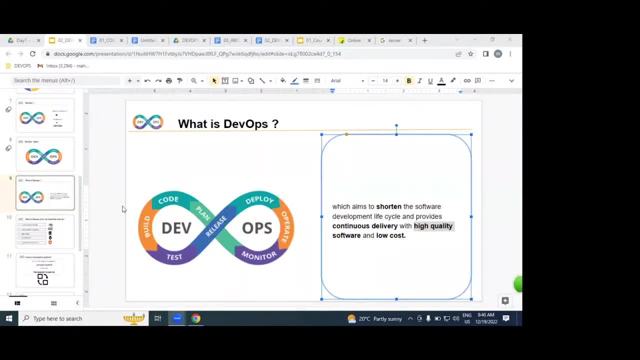 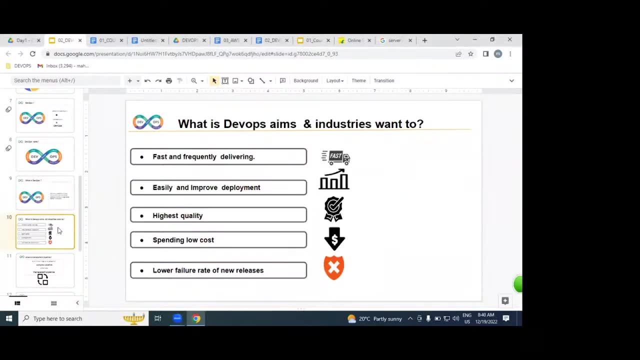 is nothing but what devops process? if we are replacing with our sdlc process with devops process, if you are replacing with the sdlc process with a devops process, what is the auto advantage? exactly, please, exactly DevOps aims, please, So we can able to deliver very fast. We can increase the. 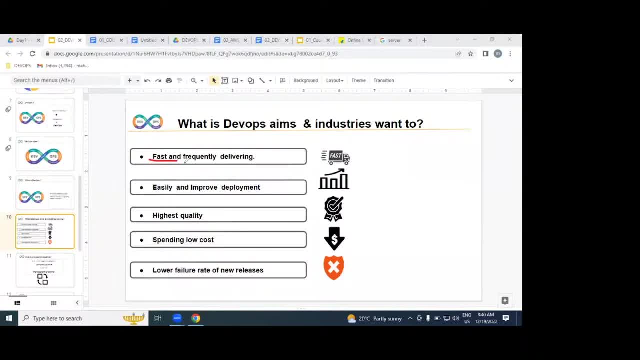 speed. we can increase the speed and frequently, and we can able to improve n number of deployments, and with highest quality, with lowest cost, with lower failure rate. These are all the advantage. These are all the advantage we can able to get it by helping our DevOps process. 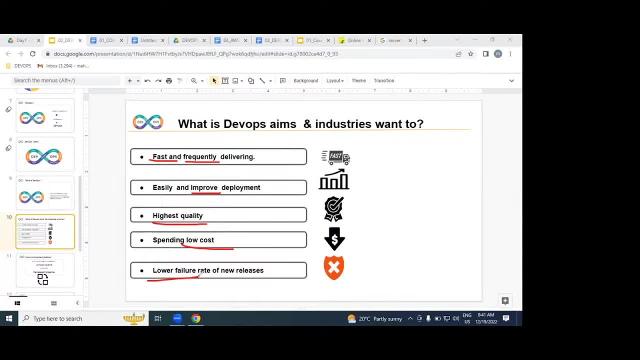 Simply, if you call this speed increase, cost is reduced, Quality is increased, quality is increased and so quality is increased. cost is decreased means who don't want this technology? That is the reason, so more demand in DevOps Understood very clearly, if you. 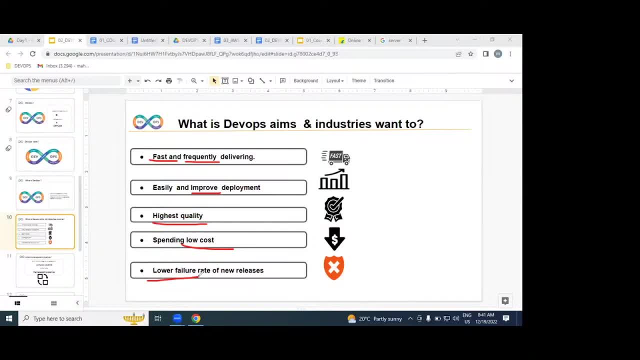 go for any shopping mall, Okay So Pepe Jeans or any Fand and Shoddy buying instead of 2000 rupees. if you getting 200 rupees, you are happy or not. Are you going to be saving our expenses or not? The same. 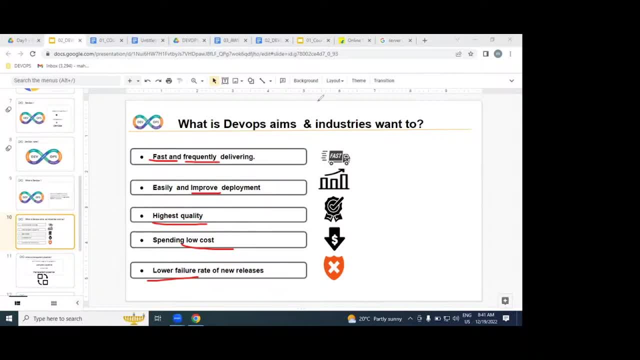 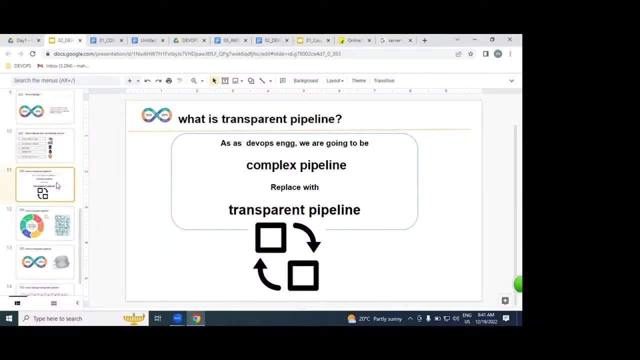 concept. Fine, Fine, please. So, but whenever? after getting a job? if you are, what is an exactly roles and responsibilities Once? if you are getting a job, what is an exactly roles and responsibilities, guys, please. So, as a DevOps engineer, we are going to be replaced. 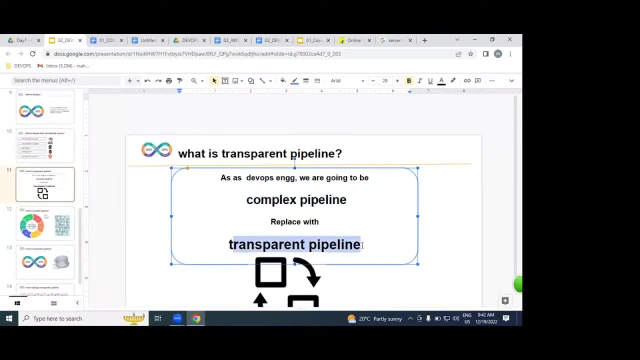 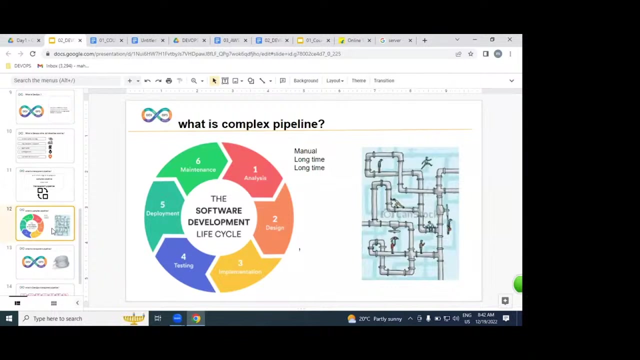 for. but in this process and every level right We are, we have, we are going to function without any optimizer or anything, because so and so just do something, Repeat that. There Is that what I, what's finally got important: in氣z: 250%, so now you understand 200. Oh, by the way, probably we have not heard in this risk is of that we have to invest. So this is the argument Question that should answer. for Well, let's ask the first one, And I think you guys CAN: what are you can get and what exactly? 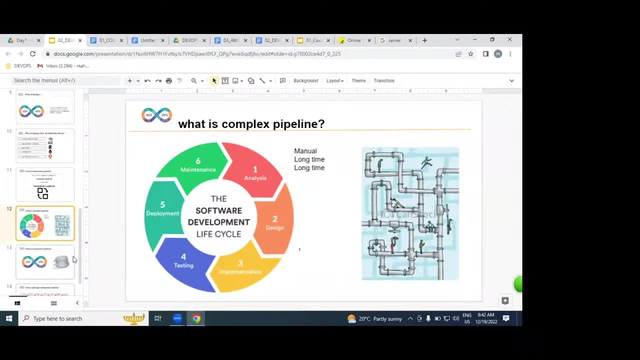 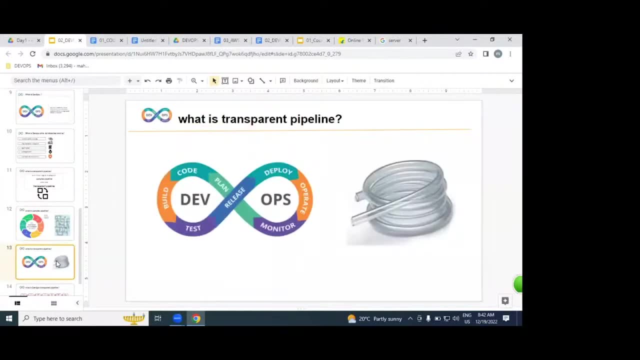 Oh yeah, obviously Say: all right, Determine and so studies, okay, complex pipeline- What is a transparent pipeline? DevOps process: Very simple. So we understood very clearly what is SDLC. We understood very clearly what is DevOps process. 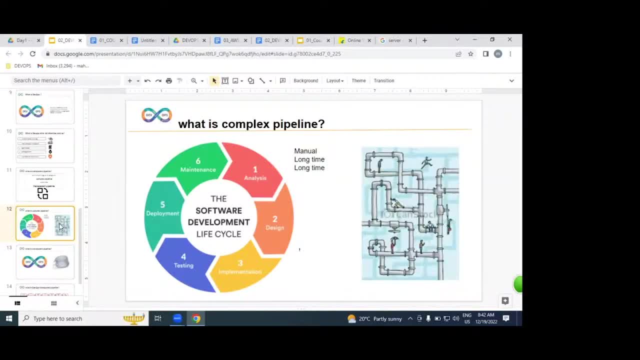 So we are going to be replacing with what Our SDLC process, with what DevOps process. Why we are calling SDLC as a complex? Because if it is a manual process, It is not automatic. SDLC is not a automatic, It is a manual process. So, from analysis to design, design to implementation. 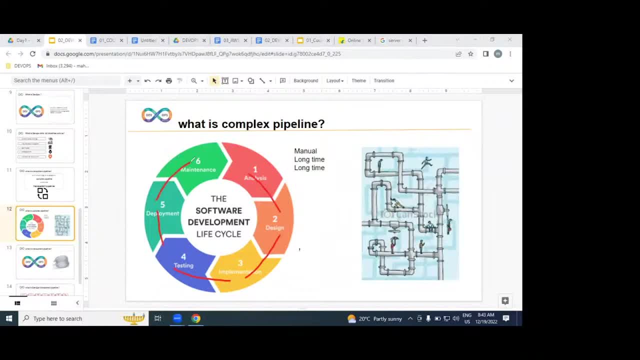 testing to deploy, deploy to maintenance. it is a manual process. If it is a manual process, if it is a manual process, if you got any issue, any problem in the middle, any issue, any problem in the middle. So 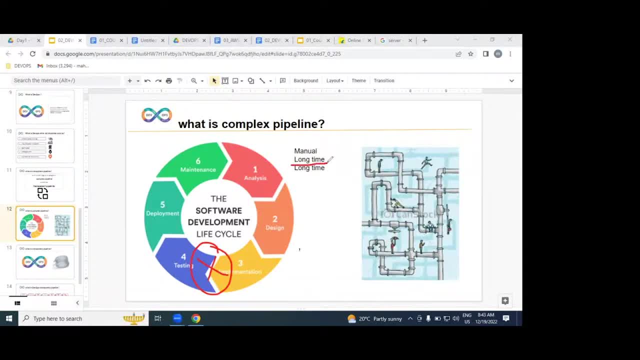 it will take long time for resolving issues, For identification issues. it will take long time because of it is a manual process. Example: a water pipeline. The water pipelines are underground. Example: somewhere else, a blockage. there is no leakage, It is a blockage, So can able to find. 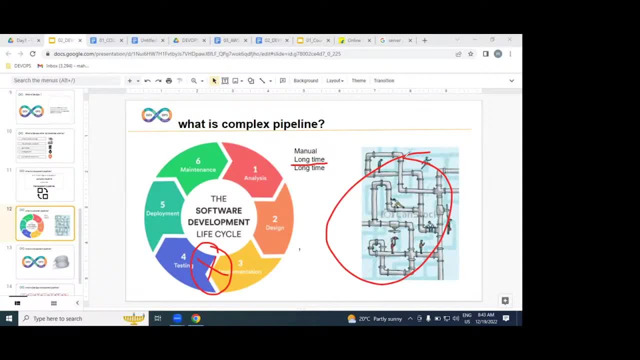 immediately. where is the blockage? Experts are required or not. We need to pay more amount or not. Even experts also can able to resolve within half an hour, within one hour, within a day. No, It will take long time. The same process in SDLC process also. If you are following SDLC process, 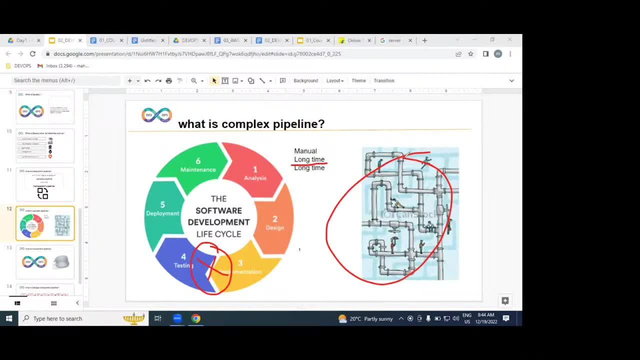 if you got any issue, any problem for identification, it will take long time For resolving issues. it will take long time. That is the reason what we will do. We are going to be replacing with what An automatic? an automatic, transparent pipeline. 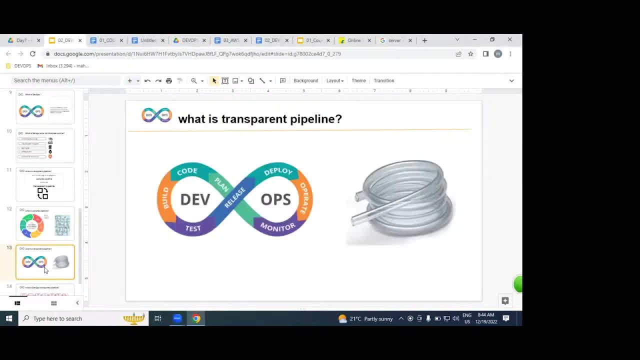 An automatic transparent pipeline. Automatic, transparent pipeline by using what Devalves Same water pipeline, it is a transparent pipeline. Look like this: Same pipeline, same usage, but it is a transparent. it is an automatic. Understood Any issue in this middle. 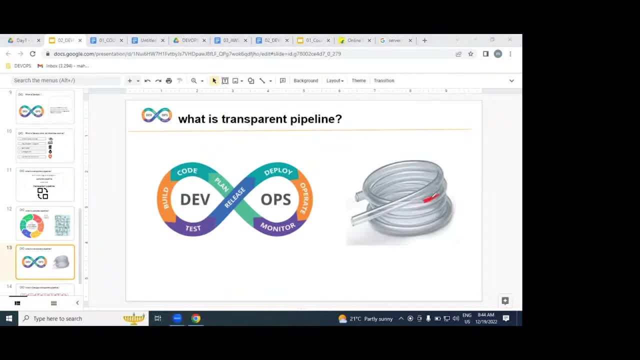 any problem in the middle occur, Any issue, any blockage. So can able to see one look itself or not In this transparent water pipeline. so can able to see one look itself where is an exactly problem and can able to resolve as soon as possible, or not. 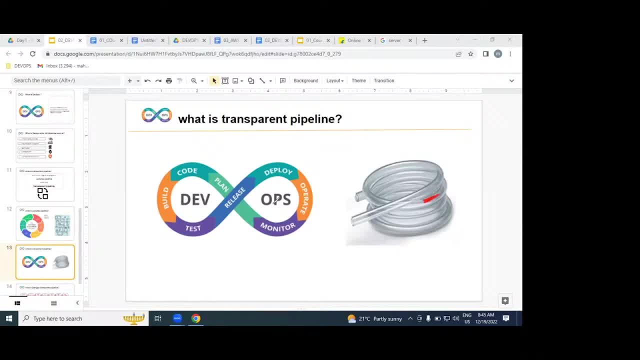 The same with devalves process also, Because if it is devalves, it is an automatic process. Devalves is a transparent process In the middle. if you got any issue, any problem, so can able to resolve as soon as possible in the middle And it is an automatic. 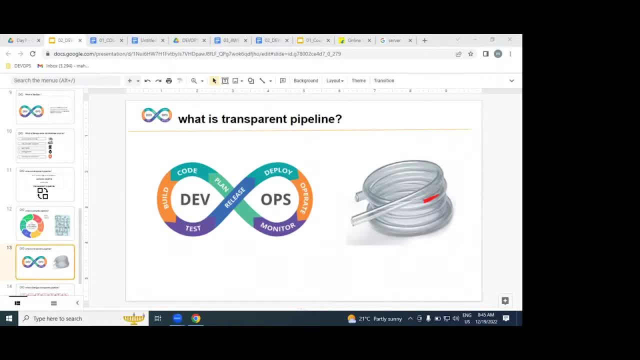 any problem is Once again, Let me continue, please. What is an exactly we are going to be, guys? please, We are going. 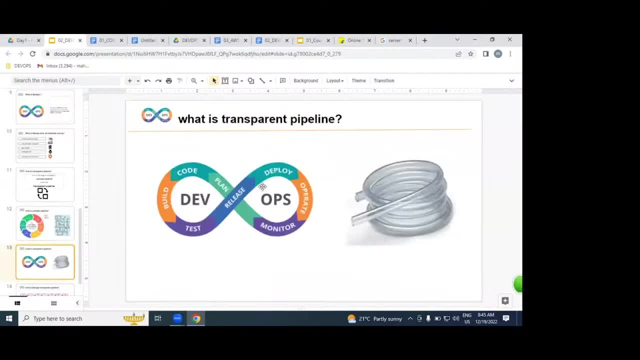 to be replacing with what Complex pipeline with transparent pipeline. Why we are calling DevOps is a transparent pipeline Because if it is a transparent, with an automatic In the middle, if you got any issue, any problem, easily we can able to identify easily. we 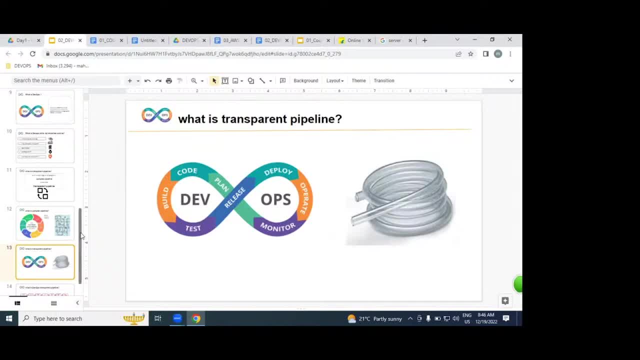 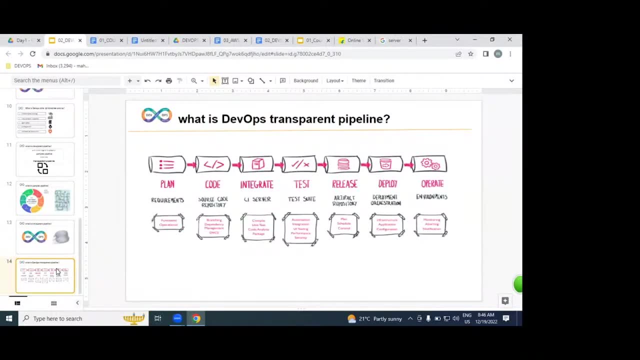 can able to resolve. But actual DevOps process- how exactly? look like this. This is what exactly our actual DevOps process, which we are going to be an implement, Our actual DevOps processes, look like this one: In this DevOps transparent pipeline, we have a several stages in several 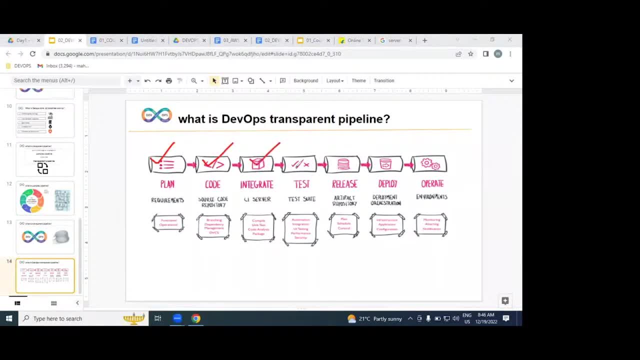 phases like plan code, integration, testing, release, deploy, operation. But in this DevOps process we are going to be, we are going to be our roles and responsibilities start from where: Dev environment- Hence, we are going to be a dev environment. We are going to be a dev environment, Hence. 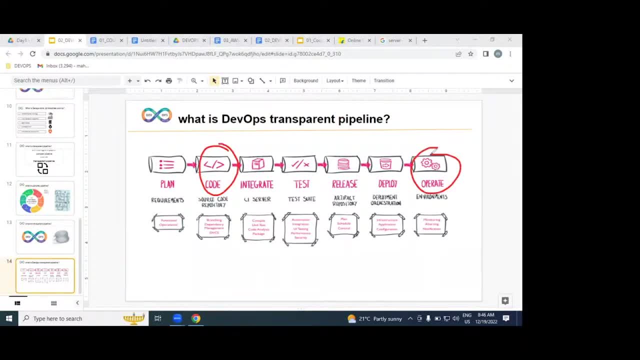 we are going to be a dev environment Hence. we are going to be a dev environment Hence with where Operations Start. with where exactly Dev environment? Hence with where exactly Operations. That means our roles and responsibilities in dev environment, in. 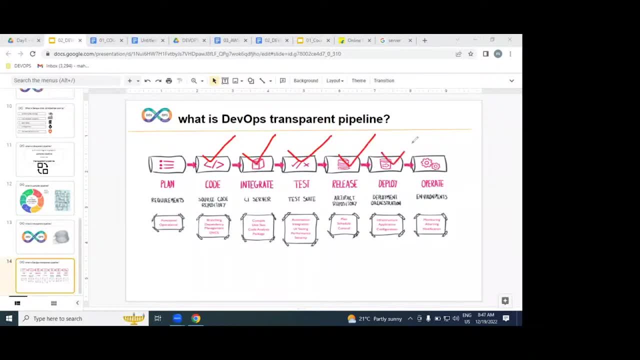 integration part: testing, release, deploy and operations. It is very clear really, To be frank, while implementing this DevOps process, We are not writing any code, We are temp. some are not writing any code, we are not writing any test cases, just we are going to be implementing. 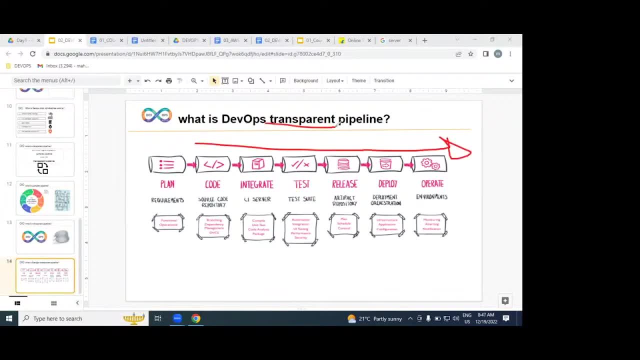 a devops, an automated, a transparent pipeline only. why? to make it speed, to increase the quality, to decrease the cost. so that purpose only. we are going to be implementing our devops process from where exactly? dev environment to operations. so let us understand this devops process in stage by stage. what exactly roles and responsibilities in each and every stage? 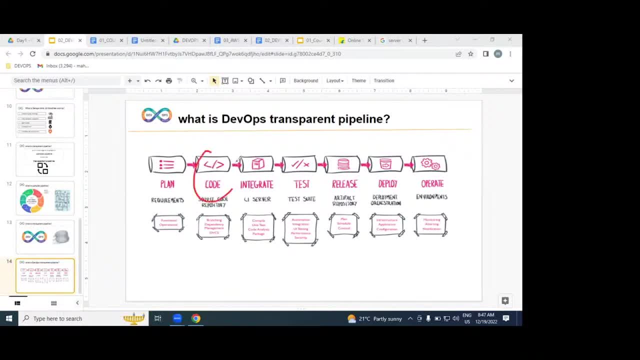 let us understand, guys please: in dev environment, in dev environment, we are not writing any code. we are not writing any code. the writing is responsible by whom? developers, the lines of code is responsible by whom. writing is responsible by whom? guys please, developer after writing by, after writing by developer that code, which? who are all maintaining writing is? 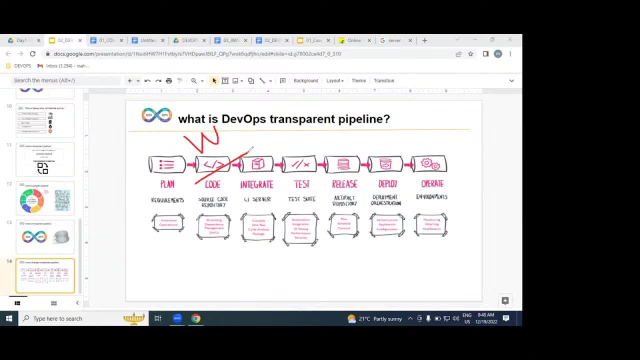 responsible by the developer after writing the code. that code is going to be maintained by devops. that's what we're part of, davenport here, all of you. it's very important point: writing is responsible by the developer after writing. that code is going to be maintaining by. 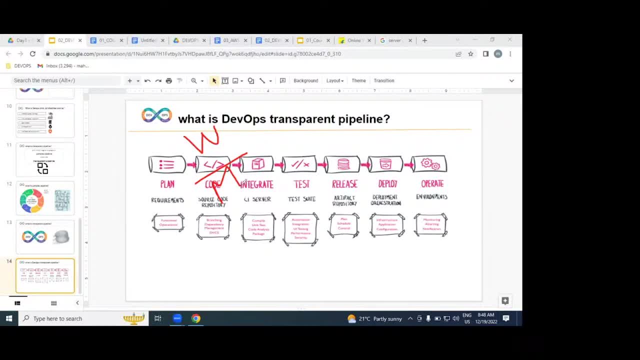 devops, engineer. but how many developers we have? please anybody help me. how many developers? please tell me n number of developers we don't know. so all developers source code. so every day, morning to evening, each and every developer writing n number of code. but all developers source code, we, we. 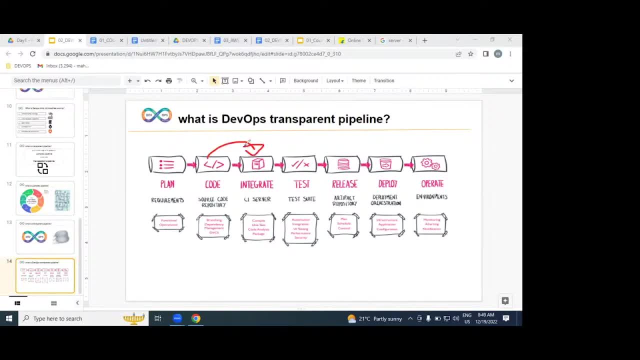 integrate or not? we need to integrate or not. yes, we are going to be integrate. how continuous we're going to be integrate once, if it is integrate, all developers source code, whether the software is in working or not. we need to execute our test cases. these test cases, who is reading? writing devops, engineer or testers? and tests will write, not by you. 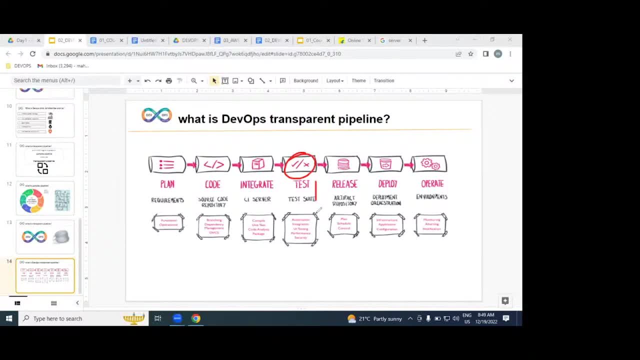 on me. So we are going to be just integrate only test cases. our job is only integrate Which is written by test season Once. if it is, execute test cases if there is no error. if there is no error, or else if you got an error, if you got an error, automatically it is. 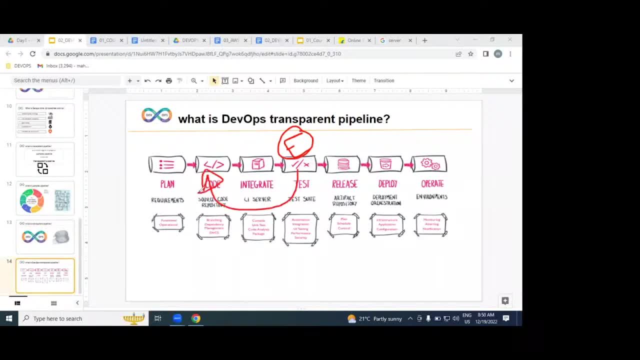 redirecting back to the developer. Developer has to fix the issue again Again. integration again. this error Understood very clearly. So developer code going to be integrate. then it's going to be verified by the test cases Once if you got an error. 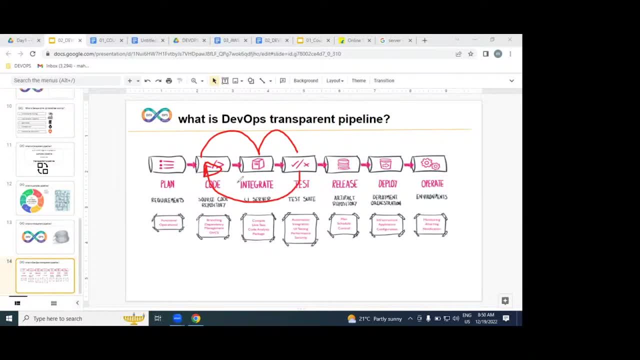 automatically it is going to be redirected back to the developer. This loop will be. this loop will be repeated until what? Zero errors, zero bugs. Once, if it is, everything is fine without any error, without any bug, we calling as what? 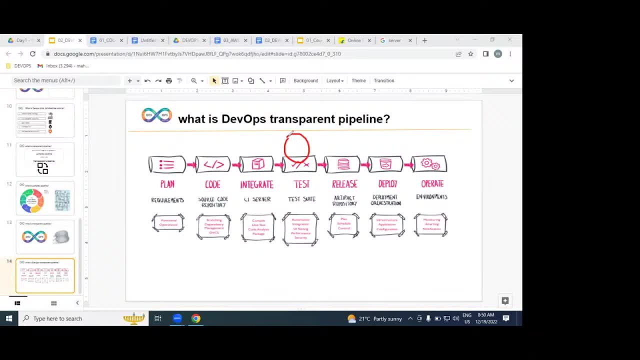 The working software as a application. What is the first question which you ask, please? What is application? What is an application? The working software, without any error. If it is working software is ready, what we will do Directly, we going to be placing on server side. No. 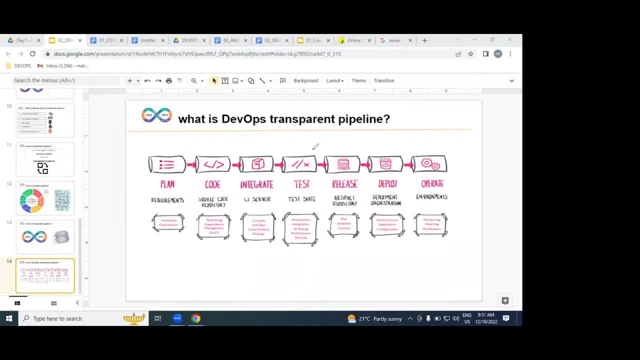 Directly. we are going to be placing on server side. No, We need to hold or halt in a particular period of time, in a release, In a release In a particular maintenance window, a particular schedule date. we are going to be placed on hundreds of servers. 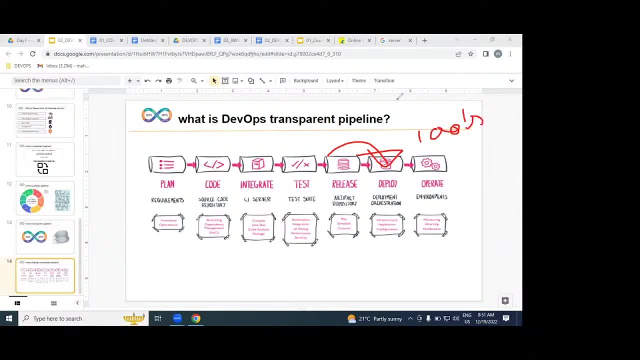 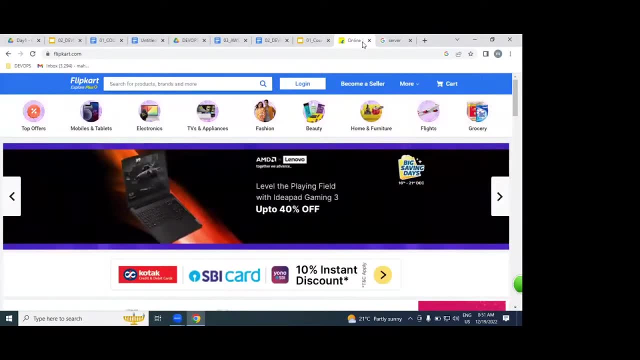 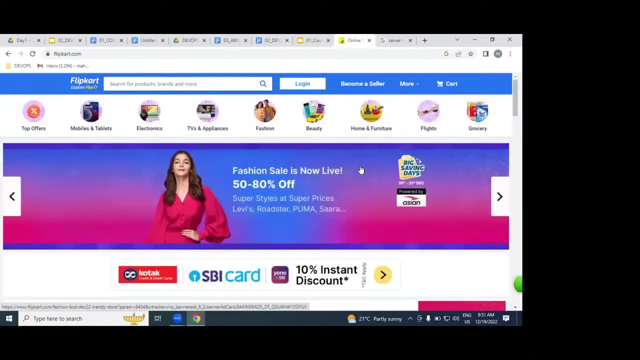 On a hundreds of servers. Once, if it is placed on hundreds of servers, we can able to access our internet as a website. This entire process we are calling as what Devops. Once if it is placed as an application, Once if we are accessing it as a website on our internet, our job is finished. 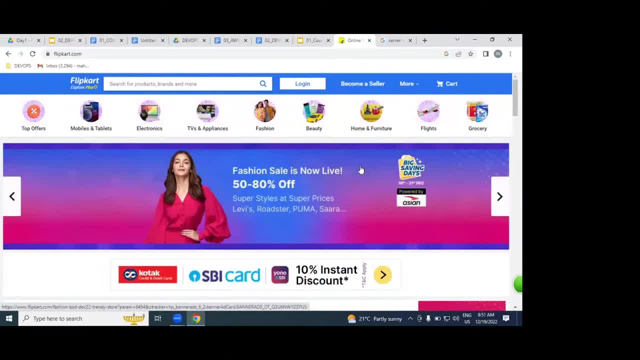 Is our job is finished? No, Whether it is working or not, we need to monitor our maintenance. That is also responsible by the devops in your own Got it very clearly what is a devops process. So devops is a process which we are going to be implementing for 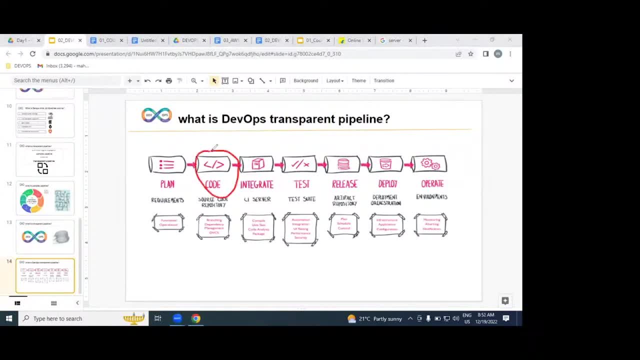 from where exactly Dev environment ends with, where Operation Ends with where Operation. That means we are part of dev environment: integration, testing, release, development and operation. We are going to be implementing DevOps and automated transparent pipeline. while implementing this transparent pipeline, make sure whether you are going to be delivered. 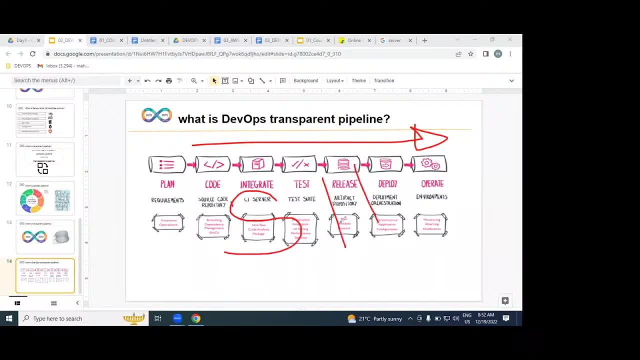 within a shortest time, with the high quality, with low cost. This is an exactly DevOps process. I hope you people understand what is an exactly this DevOps process. What is an exactly this DevOps process, But for implementing this DevOps process, for implementing this DevOps. 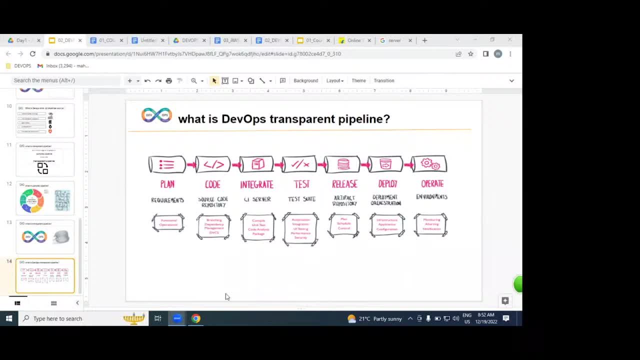 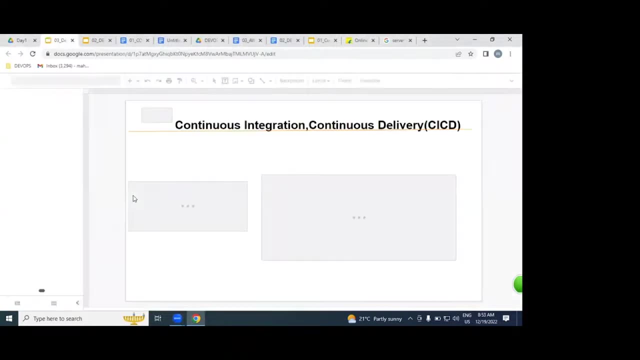 process. which are all the tools we are going to be using. We should learn something. We should learn something. We should learn something. We should learn some tools that are not For implementing this DevOps process. which are all the tools we are going to be guys, please, Liz down, Let us Liz down, Let us Liz down. Which are 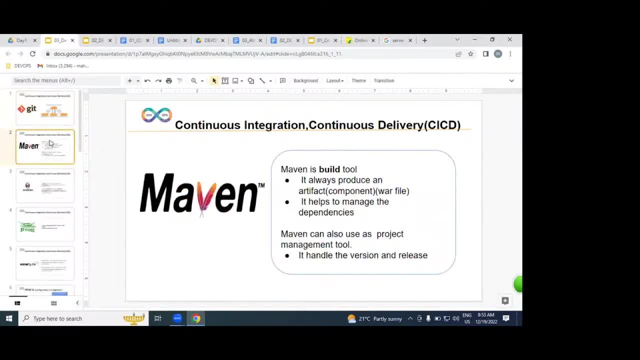 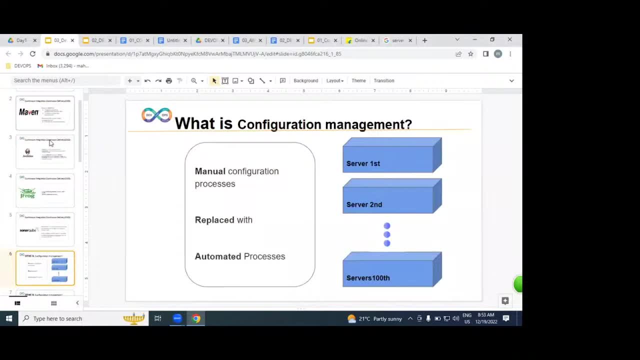 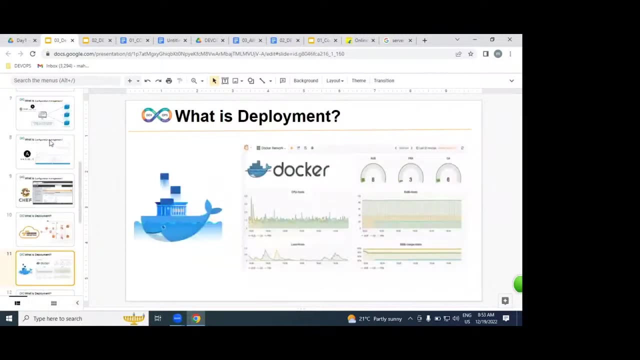 all tools, guys, please Git. we are going to be learning Maven. we're going to be learning Jenkins. We are going to be learning JFrog. We are going to be learning SonarKey. We are ansible chef aws, complete aws, docker. we are going to be learning kubernetes. we are going to be 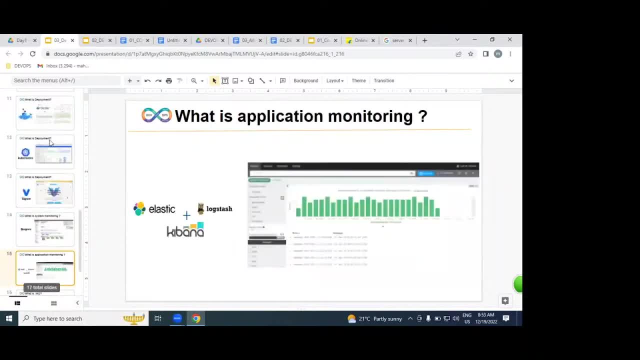 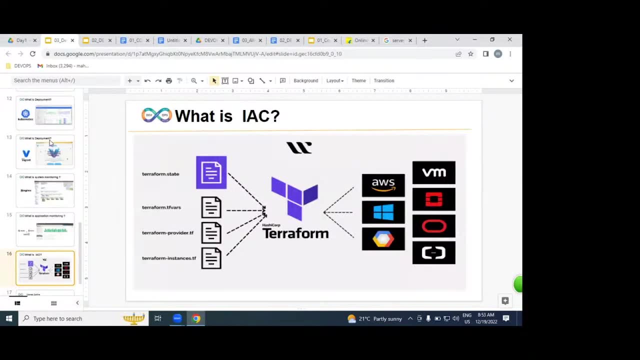 learning vagrant, we are going to be learning negios, we are going to be learning elk. we are going to be learning terraform. so these are all the tools we are going to be learning. for learning these tools, it will take more time, so by using these are all the tools we are going to be. 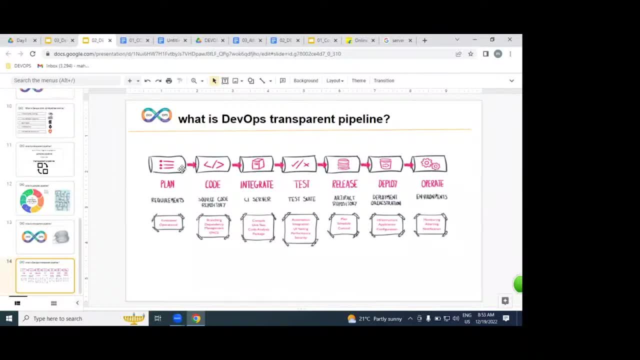 implementing this devops process, how exactly these tools are fitting into this diagram. let us understand so. firstly, so n number are developers writing code. that code is going to be maintaining by whom? maintaining by whom? and devops engineer, but devops engineer is going to be maintaining. 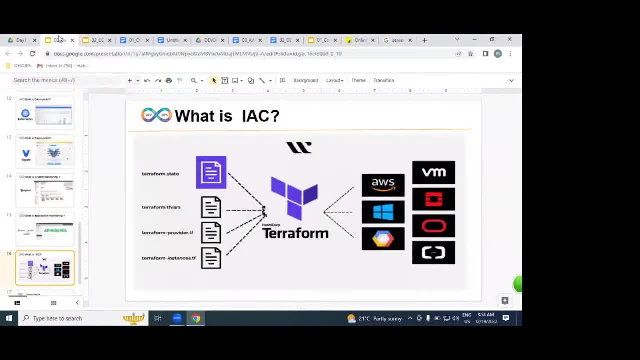 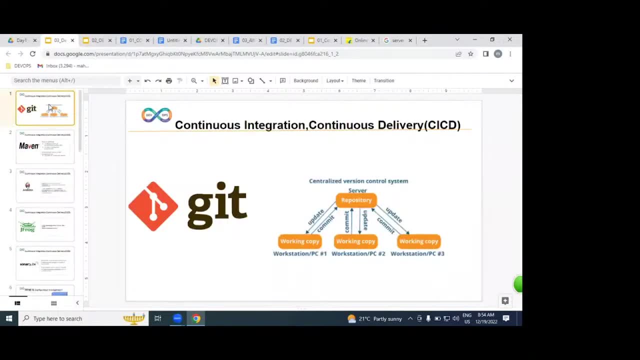 it? by using which tool? which tool? by using git. git is a version control, all developer source code. as a devops engineer, we are maintaining in a git version from git version control. but all dollar per source code we should be executed or not. we need to build or not by using maven, but this entire process we are going to be automated or not? 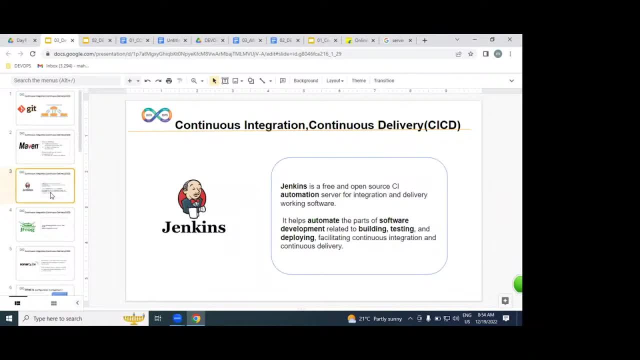 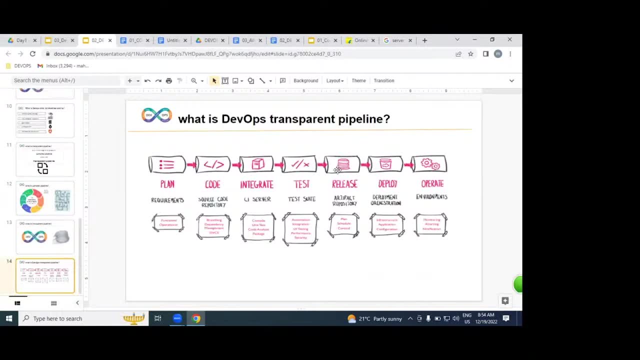 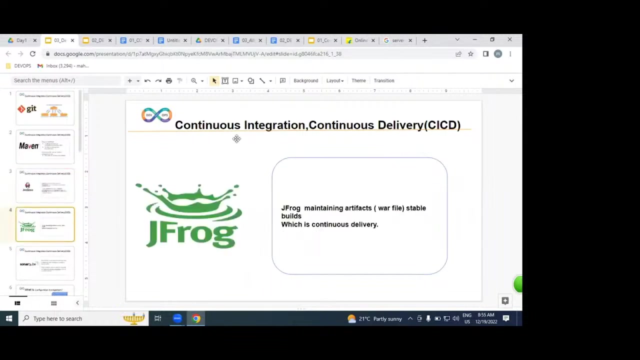 by helping of jenkins. jenkins is a an automation tool in automation tool. this entire devops process is going to be automated with jenkins once if it is once if it is an automatic, and we are going to be field our working software in release or not the release. 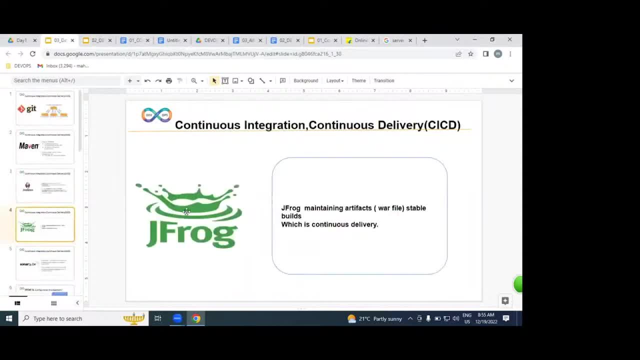 is nothing but what by using j frog. j frog is nothing but what- release and we are going to be learning sonarq. SonarQube is what exactly? Code analyzer. It is an optional tool, but we are going to be discussing, By using SonarQube, whether developers are following standards or not. it will verify and give statistics and reports. 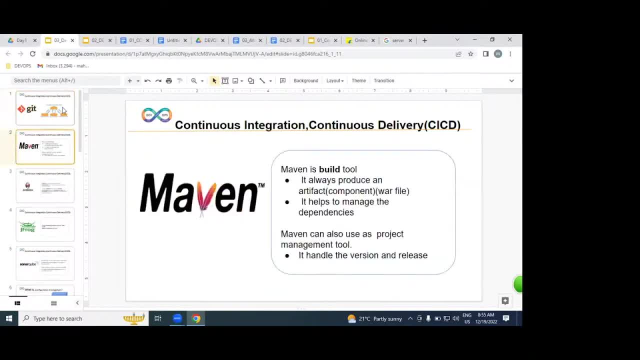 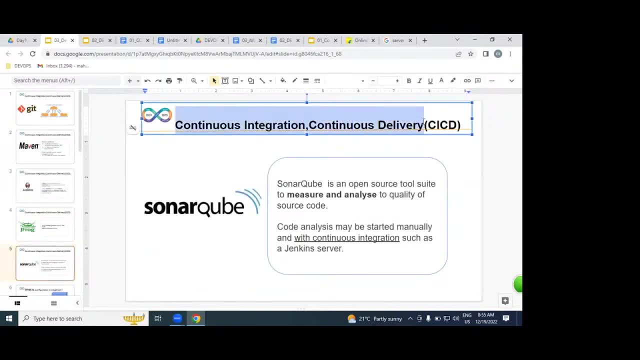 By using. these are all the tools. Which are all the tools, please ListDoc, GIT, Maven Jenkins, JFrog SonarQube. We are going to be implementing CI CD process: Continuous integration, continuous delivery. one modular. 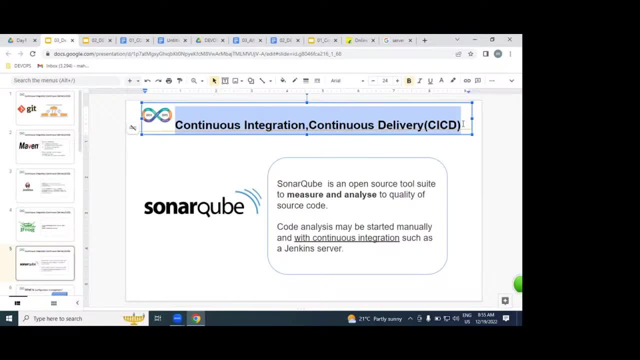 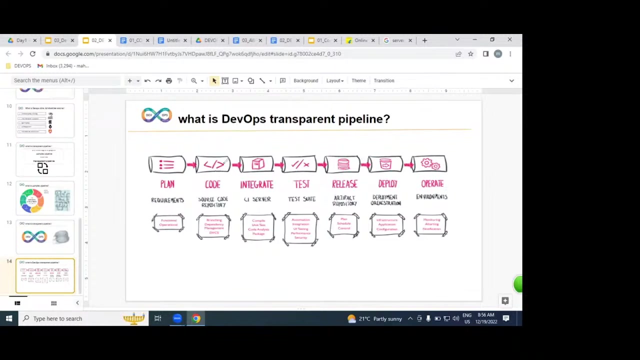 These are all the tools We call as what One model. it will take three weeks, Example, Or four weeks sometime. All of you understood very clearly, So where exactly CI CD goes. CI CD is nothing but what? Continuous integrating, continuous delivery, Continuous integrating, making working software. 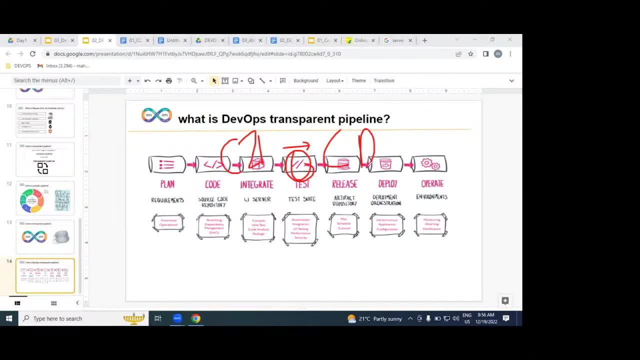 We are going to be continuous, Continuously deliver. I'll repeat this diagram, Let me So, after writing by developer, all developer source code continuously. we have to integrate. Am I right or wrong? Then, making working software by executing task space Once. if it is making working software, we are going to be deliver. 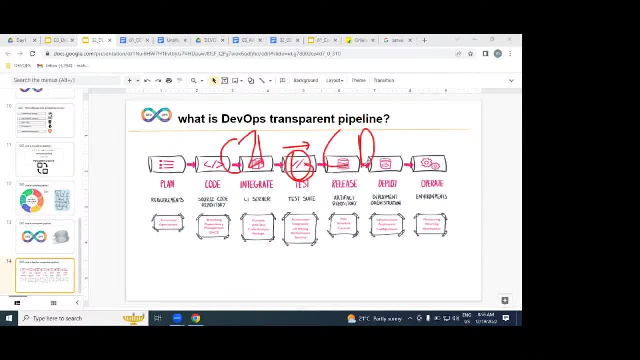 Continuously deliver. Once, if it is deliver, we are going to be placed. We are going to be placed on how many servers guys? please, If it is one server, not be here. You not be, sit here, not required. 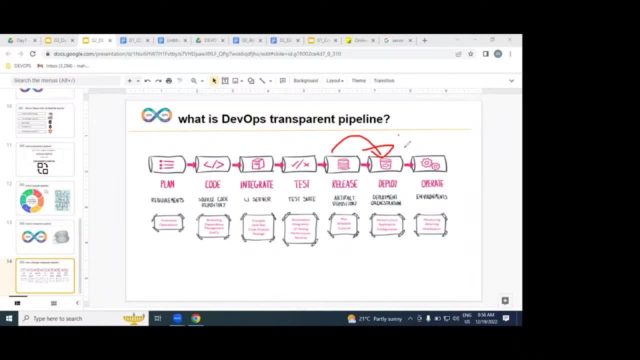 Understood very clearly. So we are going to be handling, we are going to be placed our applications on hundreds of servers. That is the reason we are be here. We are using DevOps, Understood. So after completion of CI, CD, after delivering working software, we are going to be placing on where Hundreds of servers. 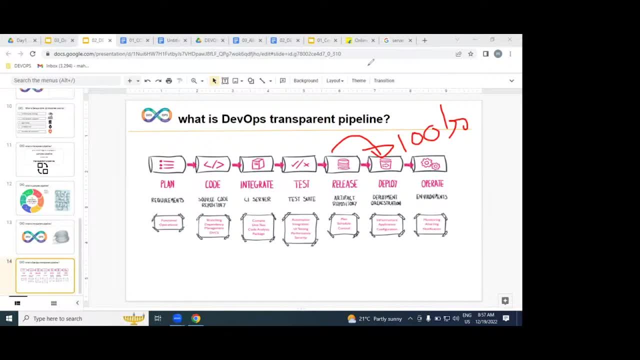 But these hundreds of servers. if you want to configure, sir, what is the configuration? Configure means what. If you buy a new laptop, what will you do, Configuration or not? You buy a new laptop one day You are going to be configured at, maybe network settings, maybe installing some software like Microsoft. 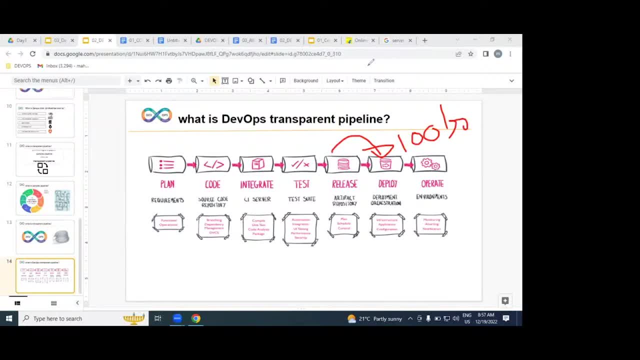 Maybe PDF, You are going to be configuring something X, Y, Z or not, according to your requirement or not. That we are calling. We are calling as a configuration, But here is how many servers we have: Hundreds of servers And each and every server. we need to install the software, We need to create a file, We need to change the files. All of you are now. But if you want to do manually, server by server, how much time? Just think about it. For laptop it will take minimum one hour and I hope maybe. But server It will take more than two days, three days also for server. 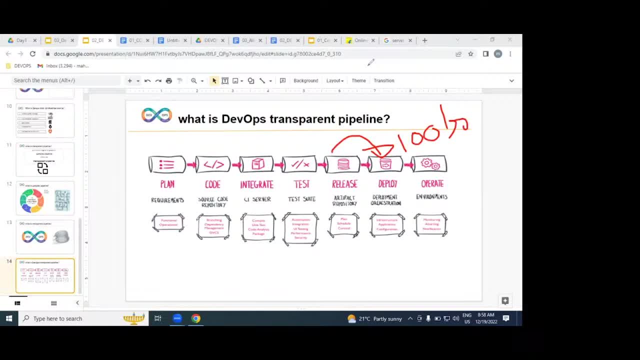 But hundreds of servers. it will be completed. how many days It will take, how many months Can able to complete within end of the day? No, but if you want to do that, we require an automation process. That automation process we are going to be implementing, by using what? 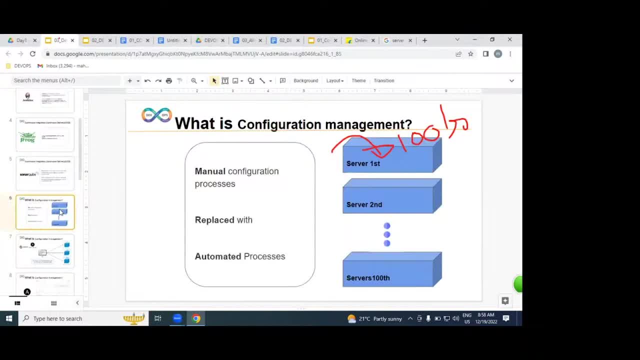 Configuration management systems. Configuration management. So what is an exactly configuration management? Please anybody help me. You know that answer: Manual process replaced with an automation process And hundreds of servers. it is nothing but a configuration. So our job is what exactly? Creating files, installing softwares and hundreds of servers. 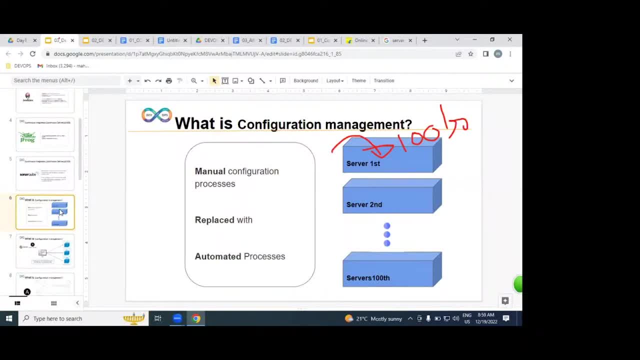 How? With manual or without manual, Without automation, Manual or automated? Automated For that? we are using what Configuration management? By using configuration management, hundreds of servers, We can automate. We are going to be replaced with what Manual process? with what Automation process? 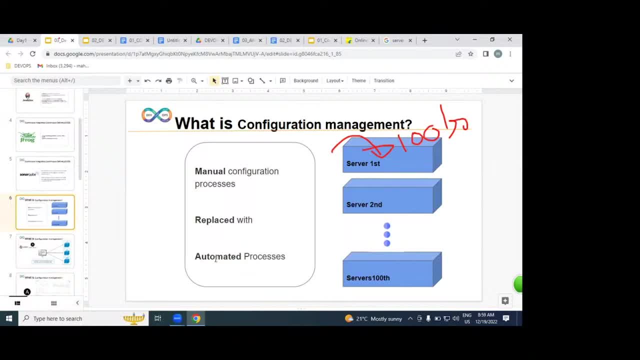 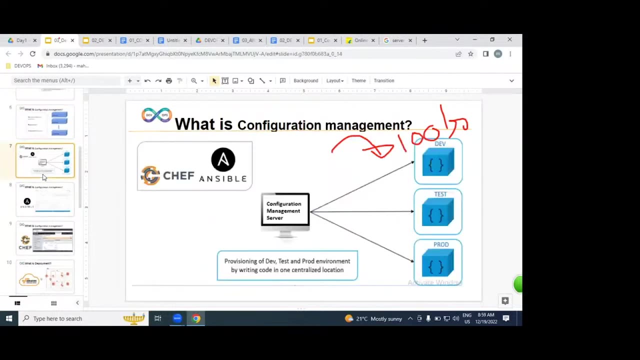 Automatically, we can able to create hundreds of servers, Automatically creating files on hundreds of servers, Automatically installing softwares on hundreds of servers. Clear, all of you. But for this, which are all the tools supporting us, please? So it's going to be supporting Ansible and Chef. 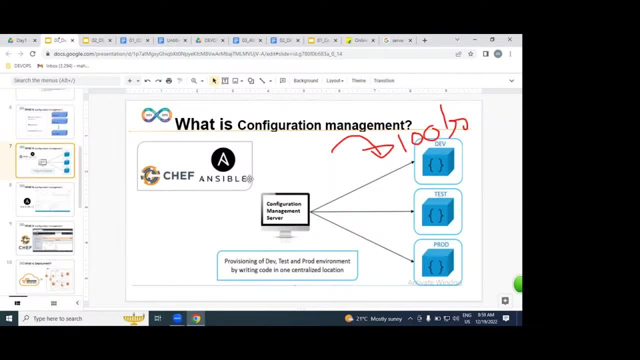 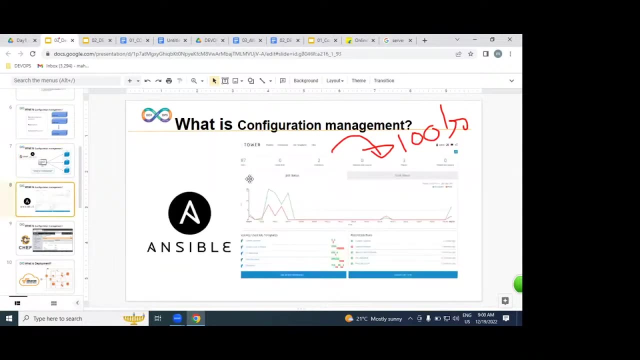 Ansible and Chef. By helping of configuration management, we can automate n number of dev environment. we can automate testing environment. we can automate production environment. we can automate. But we are going to be learning one push model: Ansible is a push model, Chef is a pull model. 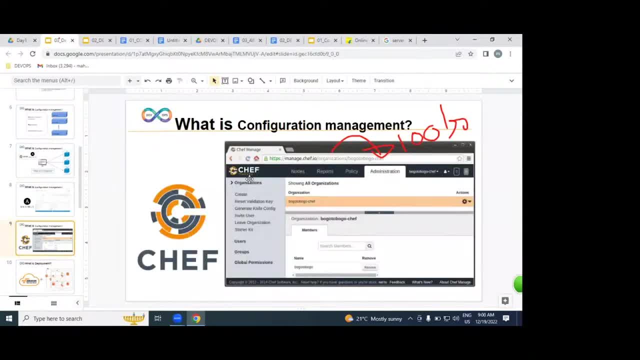 One push model. we are going to be learning one pull model. we are going to be learning. Clear all of you: What is a pull, What is a push? Don't ask me. We'll discuss in the regular session. It will take one hour. 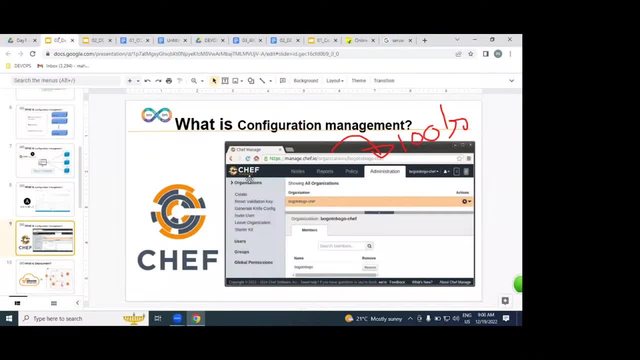 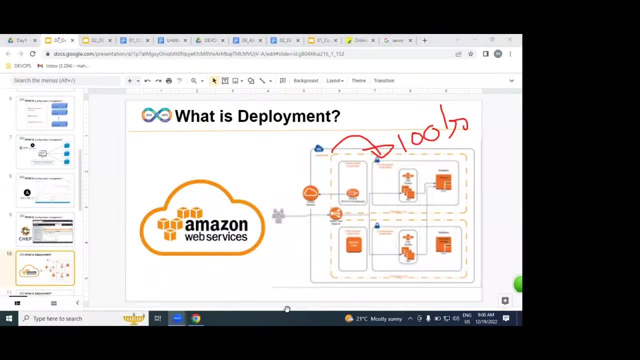 For the statement. if you want to clarify it, it will take one hour, Not for today. Okay, I will discuss deep discussion, not for today, And then we are going to be, please. We are going to be discussing what exactly? 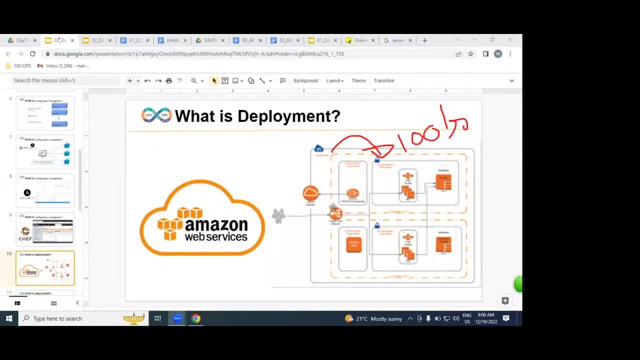 AWS. AWS is a complete course. We are going to be discussing AWS as a complete course, But here is what we are going to understand. So, as we express, As we discussed, you know, we are configuring how many servers. only 100 servers, from where? 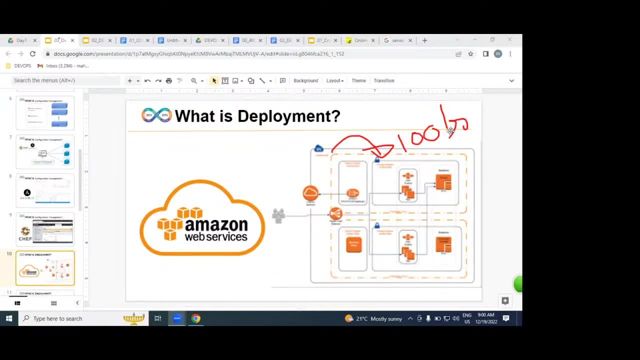 we are getting hundreds of servers. If you have a laptop, we can configure. if you don't have a laptop, from where you can able to get it done, Question is that: where, from where, how many times, how many ways we can able to get a? 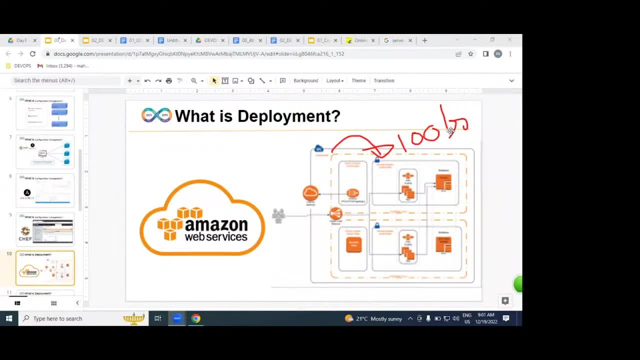 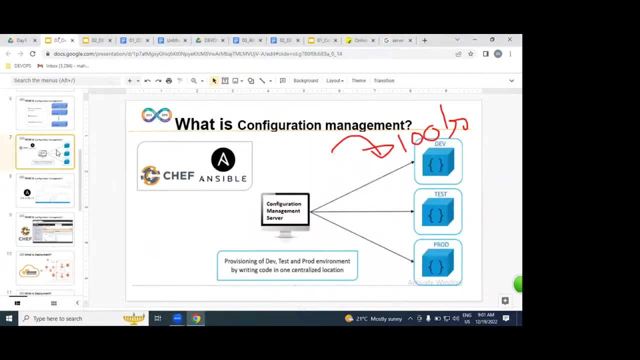 servers, and physically, like your laptop, virtually, and cloud which cloud, which cloud. we are going to be getting, as please, hundreds of servers. We are going to be getting from where AWS, on top of hundreds of servers, we can able to implementing automated process by helping of Ansible and Chef. 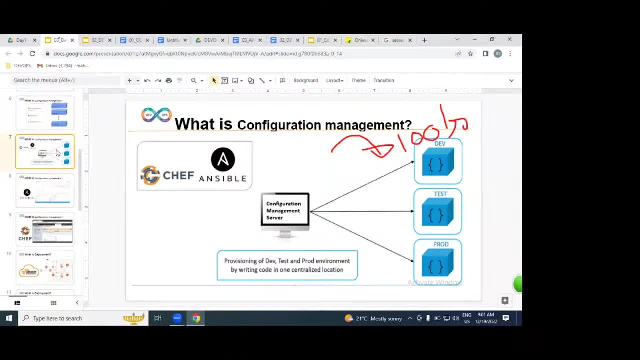 I'll repeat this point, Very important point: getting servers from AWS. after getting servers, we are going to be implementing an automated process by helping of Chef and Ansible. Chef and Ansible- that's very simple, Am I right? But so we are going to be deploying servers on where AWS servers, am I right? 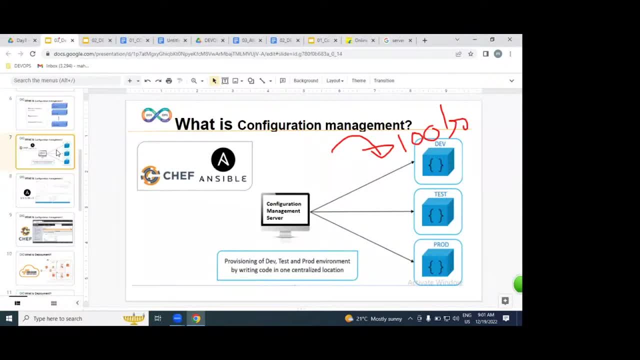 By using Ansible, by using Chef, we are going to be deploying our applications on a hundreds of AWS servers. That is the point we are discussing from starting up, the session Application. what is an application? Am I right? The first question is: that or no? 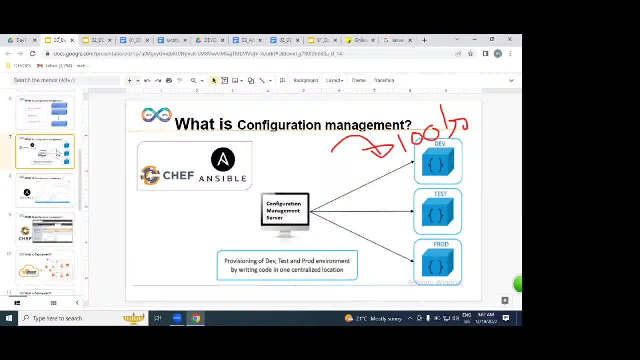 But I've shown you only one server, but right now 100 servers. but the servers are from where exactly? we are getting AWS, Am I right? Yes, That is the point, But are we deploying our applications on only AWS servers? 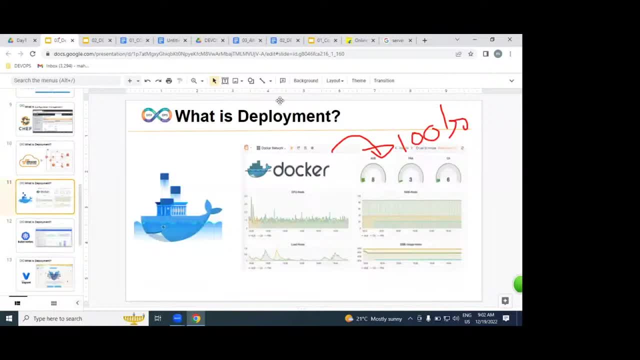 Are we deploying our applications on only AWS servers? No, We can deploy our applications on Docker. also, We can deploy our applications on Docker container. understood very clearly. If anybody asks you what is a Docker, What is the statement? Docker is a container. 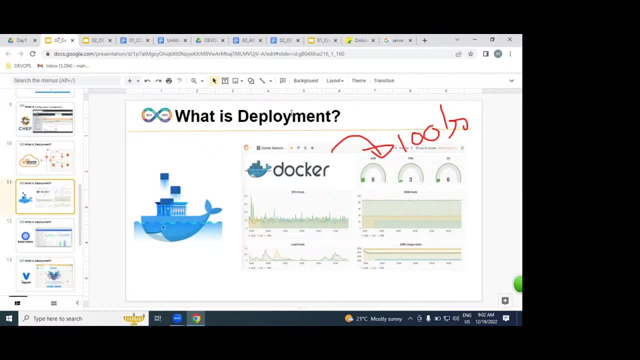 Docker is a container. Docker is for only websites. deployment Understood very clearly. What is a Docker For placing our websites? Very simple word. What is a Docker For placing our websites very easily, with the high performance, with low cost? 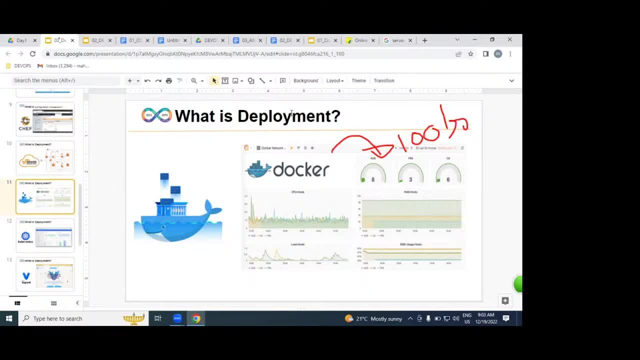 Understood very clearly. You know, for example, PIP engine. you want to buy it for 10 rupees. Is it cheap or not? Same quality, same fan, but 10 rupees, Same thing here. So for getting servers, instead of spending crores of rupees. 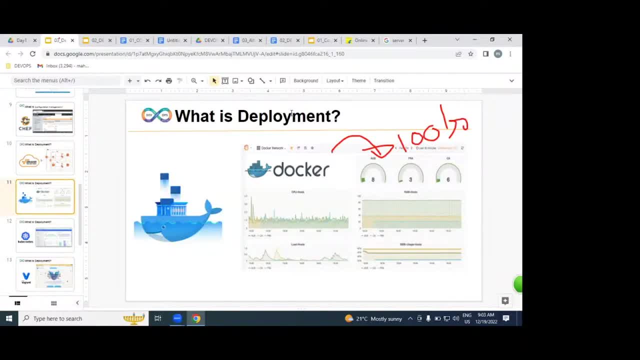 we can able to deploy our application with a minimal cost by using Docker. What is a Docker? Docker is an isolated area which is specifically deploying our application. That is a definition, But easy way for deploying our websites. Simple, one Definition point of view. 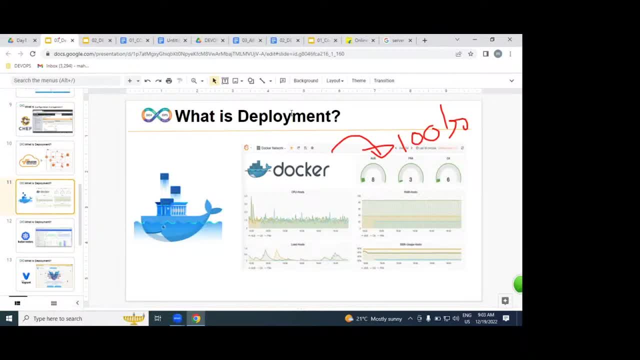 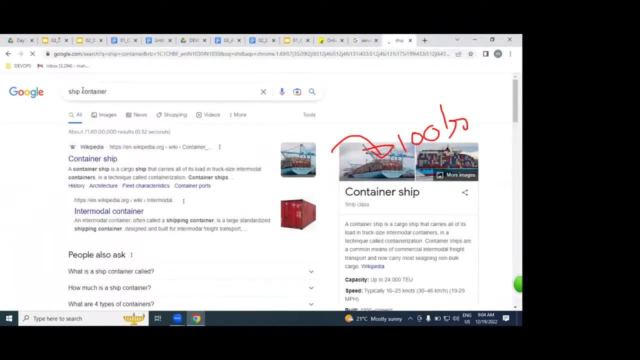 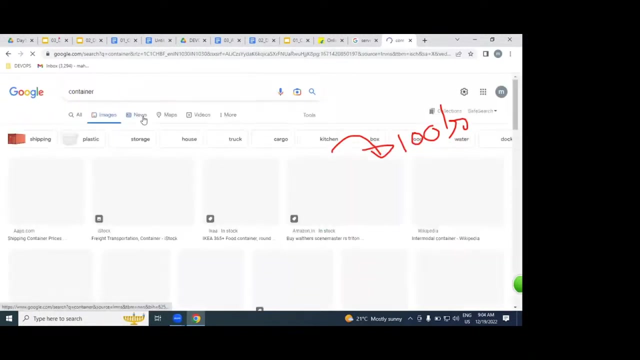 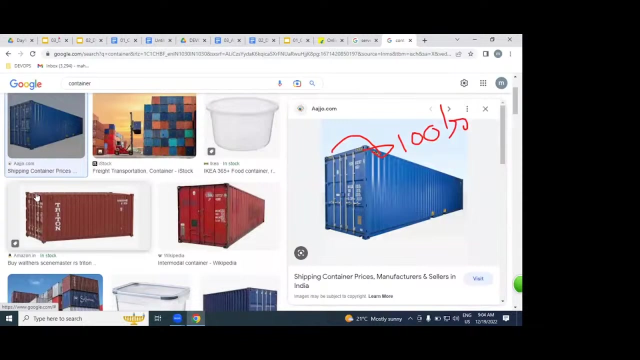 Docker is an isolated area which is specifically deploying our applications. Understood very clearly. Example, Example. So container. Have you seen this container in a lifetime? Have you seen this? Have you seen this container space? I think you would have seen this physically somewhere else, on roads. 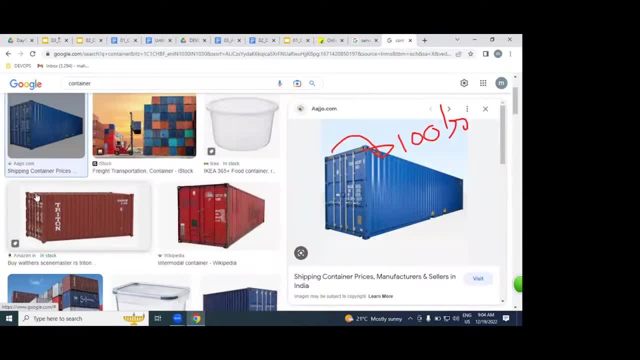 You can see this type of containers, How exactly this container works. Same as Docker container source, But by using this container we can able to transport in the YSC. But by using our container we can deploy our applications, Means, websites. 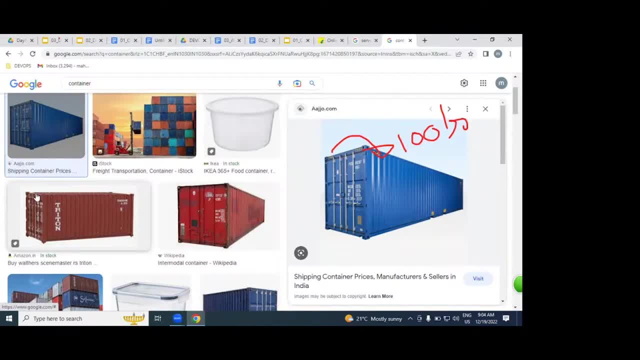 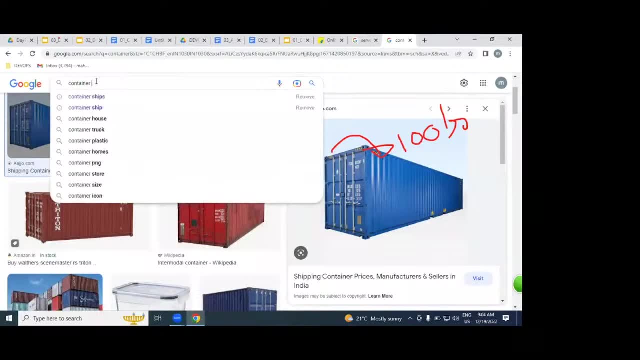 That is only difference, The same as it is No difference, Understood very clearly. But this container, we can deploy our applications. But this container, we can deploy our applications, But this container, we can manage by who. This container can manage by whom? 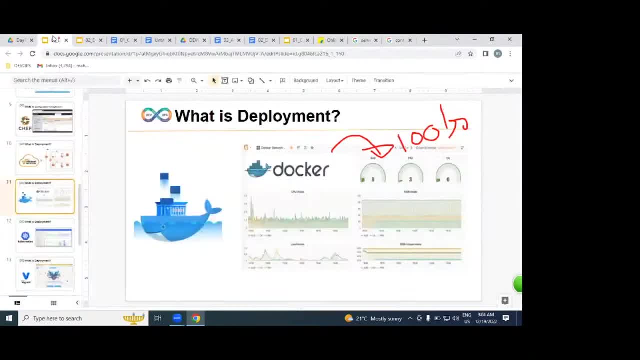 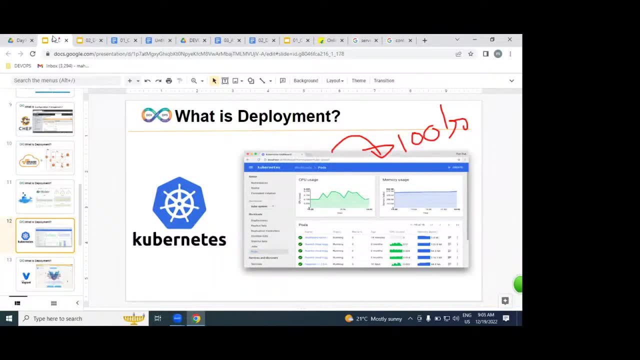 Ship. But where is the ship here? Kubernetes, So Docker. by using Docker we can able to deploy n number of applications on n number of containers. Those containers can managed by control by Kubernetes Steering up The Shipper. Understood very clearly. 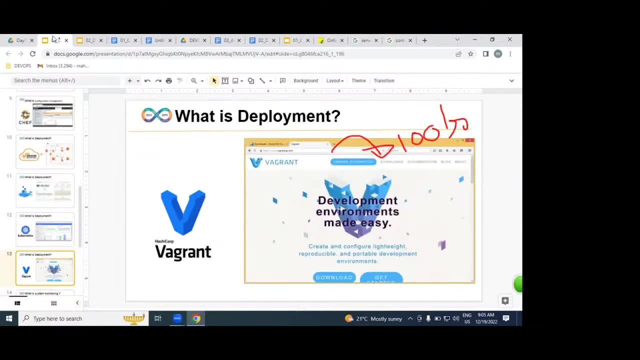 So, not only deploying applications on Docker, not only deploying applications on Kubernetes, We are going to be deploying our application by using Vagrant. Vagrant is a virtual provisioning tool. We can able to create a virtual machines in your laptop or not, a production environment. 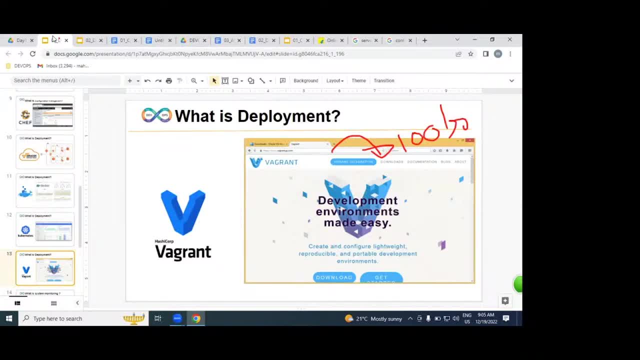 On top of we can deploy applications also. Vagrant is a virtual provisioning tool for only laptops, Not for production, But AWS is a production environment. Kubernetes is a production environment. Docker is a Kubernetes production, But Vagrant is only for Davenport. 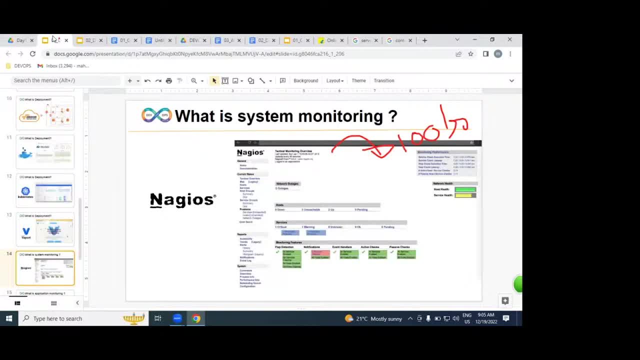 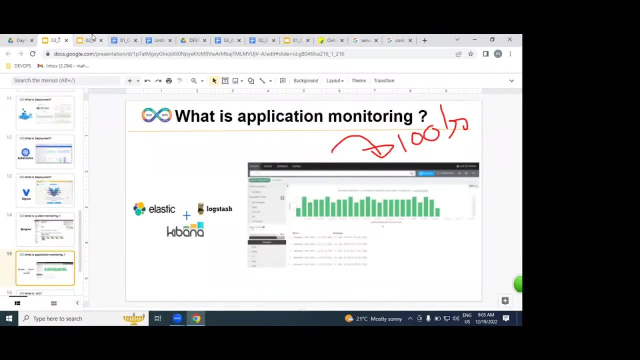 And we are going to be using Nagios. Nagios is a system. monitoring Means RAM. What is the RAM size CPU We can able to monitor? We are going to be learning Elk. Elk is a Elastic Locks, as Kibana. 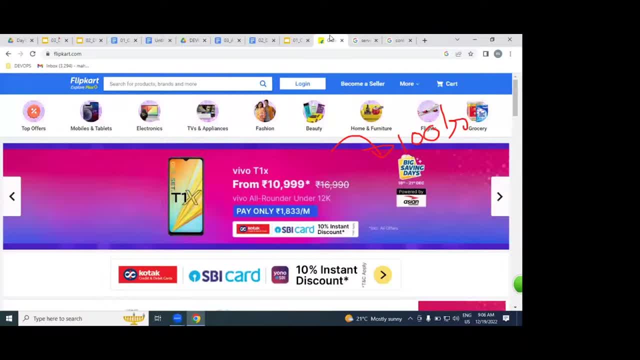 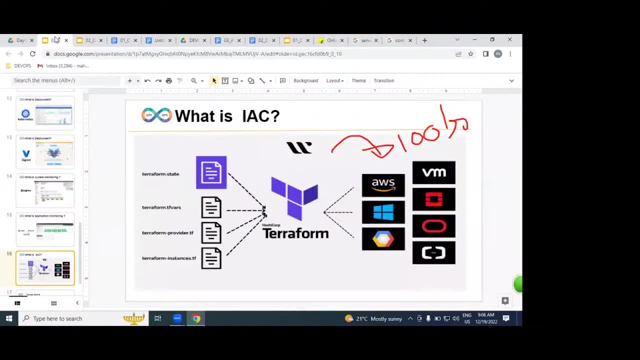 We are going to be monitor applications, How exactly this website is performing, And we are going to be learning Terraform. Terraform is a cross-cloud platform. By using Terraform, we can able to create a service in cross-cloud Means- AWS, Azure, Google, any cloud. 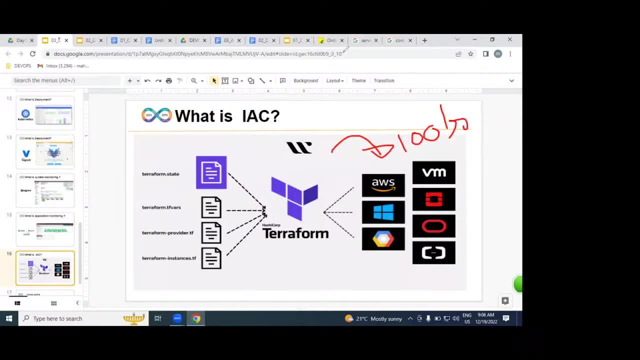 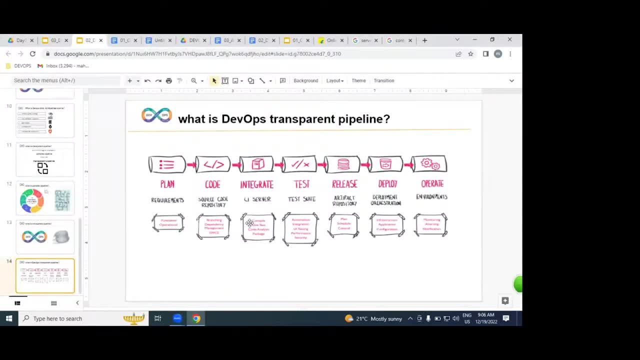 By using these are all the tools, By using these are all the tools, By using these are all the tools, we are going to be implementing our DevOps process. Clear all of you. So what is the DevOps we understood? Which are all the tools we are going to be understood? 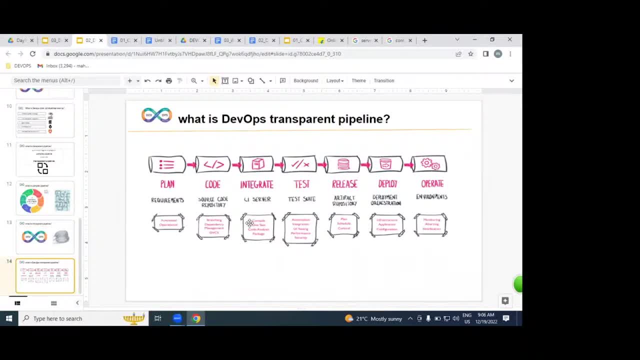 And which tool is where exactly? We are understood very clearly, Clear or no? What is the DevOps? If anybody ask you what is the single line answer: DevOps is an automatic process Implementing from the environment of operation To make it speed. 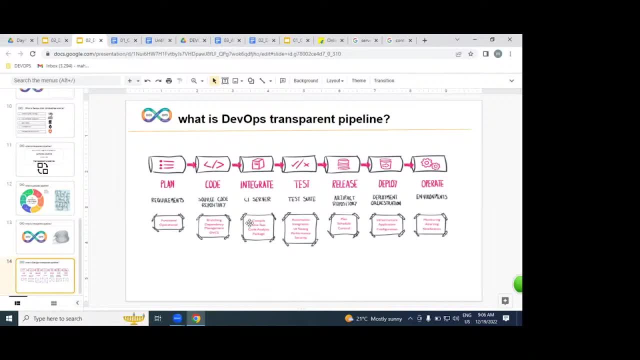 Means shortest time, Increase the quality, decrease the cost. This is only one sentence. Please write down, and we can leave Only one sentence. I will repeat: What is the DevOps? DevOps is a process, So for implementing an automated process. 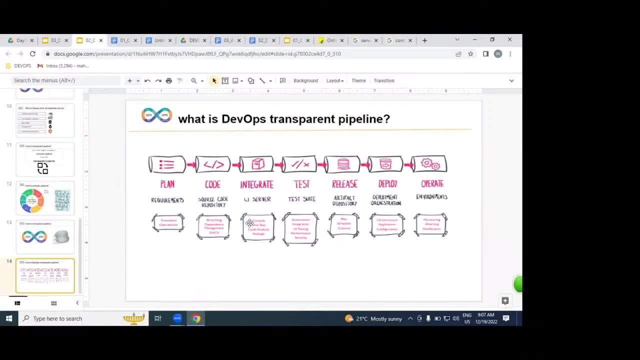 From DevOps, From the environment to production environment or operation. While implementing this process or working software which is written by developer, Making very speedily, within a shortest time, We can deploy on production server with high quality, with low cost. It is nothing but DevOps process. 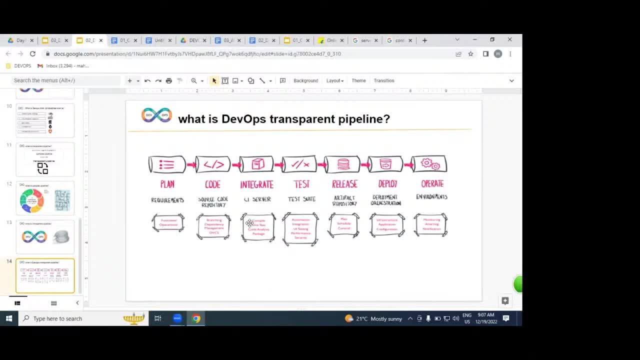 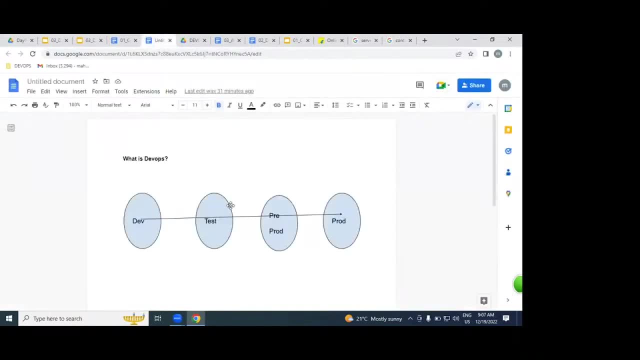 This is only one point we learned for today. This is only one line sentence. we learned for today. only the whole story. Okay, Tomorrow we are going to be discussing about What is AWS and what is the difference between AWS and DevOps. 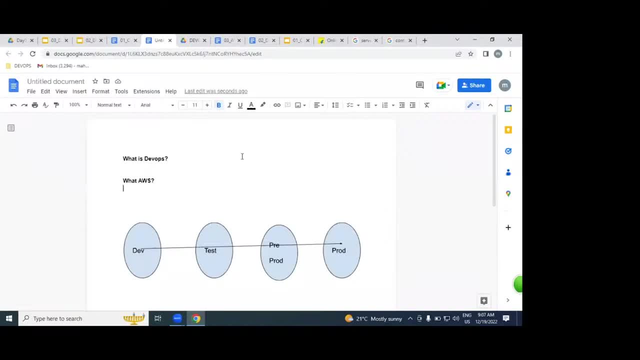 That is a class for tomorrow. I hope you people are understand what is DevOps? enough for today. I don't want to get you brained more for today. Tomorrow we'll discuss about what is it. Then we can come back Understood. 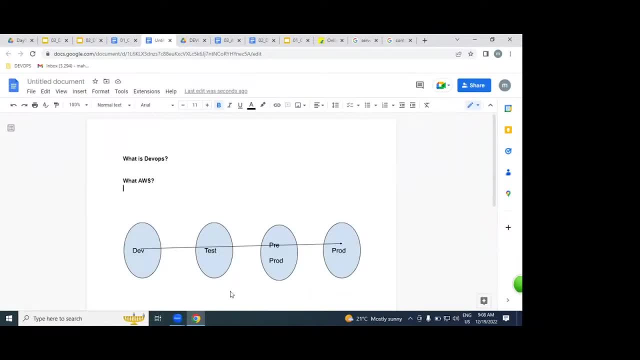 Very clear. That is a class for you. Do you have any questions? please First Let me take an Online students question, Then I'll take offline. Okay, First let me clarify online students. So before taking the questions, please let us revise. 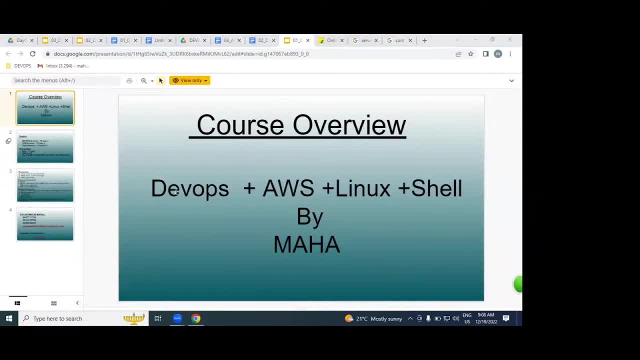 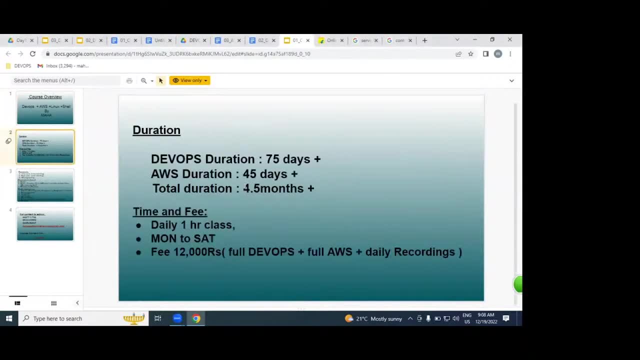 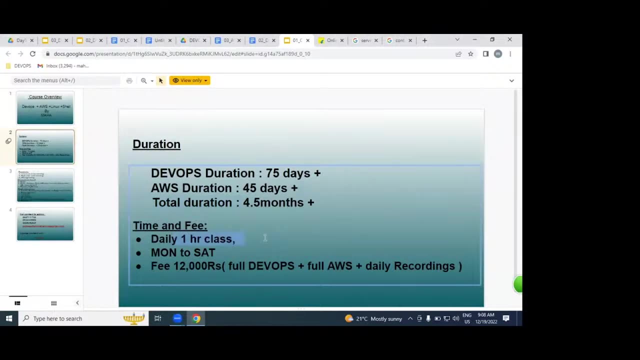 So this is, as we discussed, the vast place AWS plan, especially by me, maha. So. so total duration is four and a half months daily, One hour class, eight AM to nine AM, one hour session only. before nine AM I'll close the session. 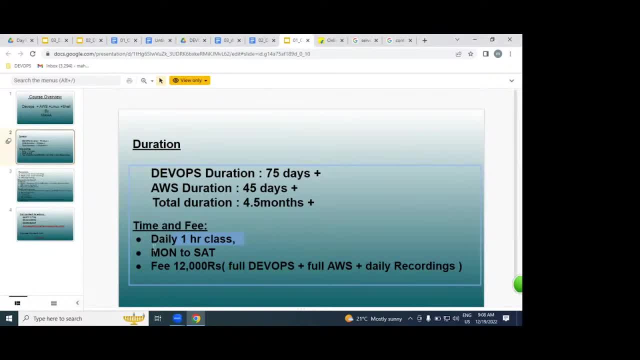 Don't be exceeded because of you need to practice Monday to Saturday, sometimes Sundays. Also, you're going to be paying 12,000 rupees fee for what? full AWS, full DevOps, but daily recordings? We don't recordings, We can't be practice. 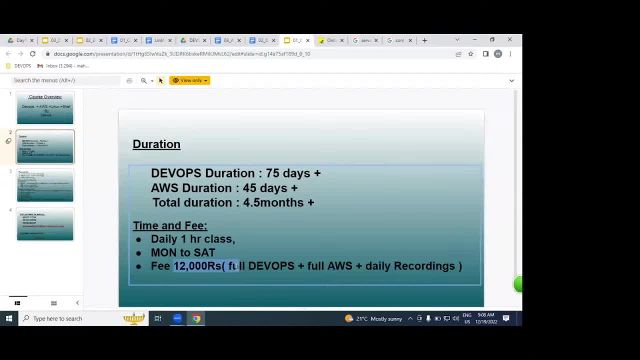 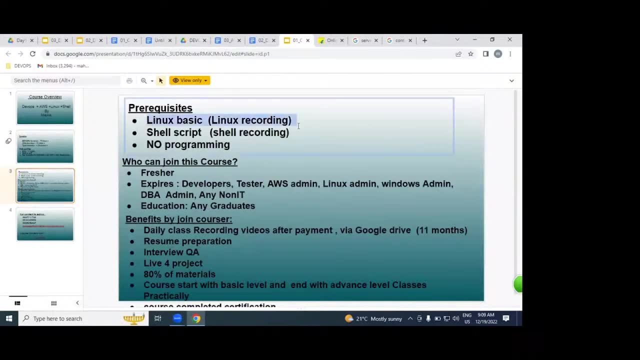 Sorry, It is inbuilt. no separate videos included Nothing, And it is a combo package, single time. So Linux basics shell script I'm going to be covering. No programming is required. Yeah, Yeah, Yeah Yeah. 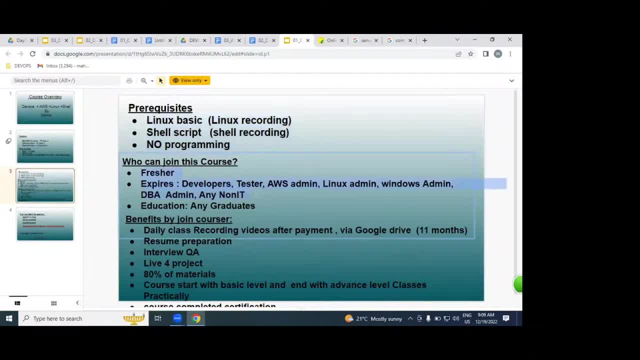 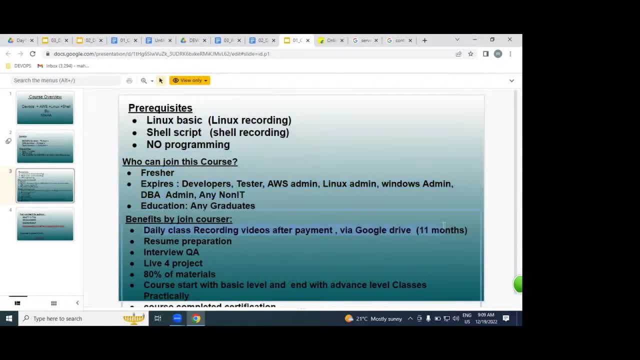 Daily recordings will be received by after payment via Google drive. The 11 months of access from date of registration you're going to have been accessed. 11 months are only 11 months, No, and the lifetime: unofficially: officially: 11 months. unofficially, lifetime. 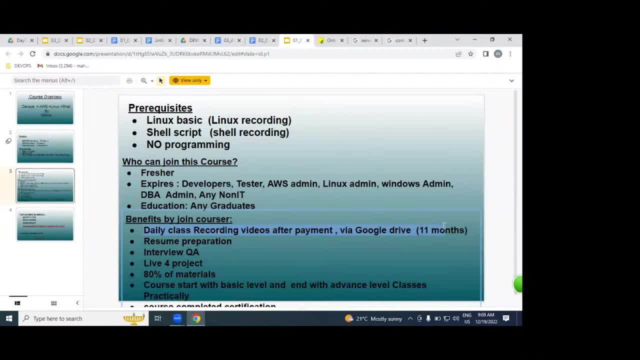 But the namesake. we need to take a. we need to give an expiry date or not. That's what level and resume preparation interview question and answers: yeah, live, four live projects. these four live projects inbuilt the course, not a separate 80 percent of the soft material. our course starts. 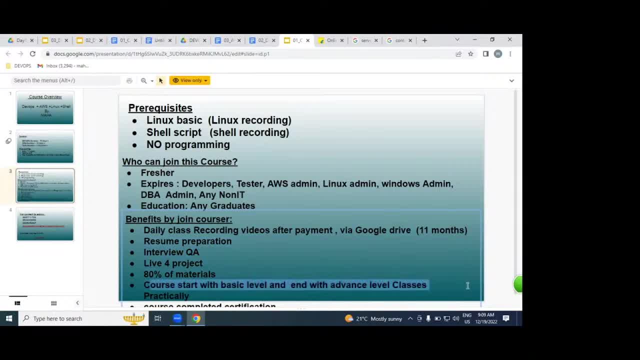 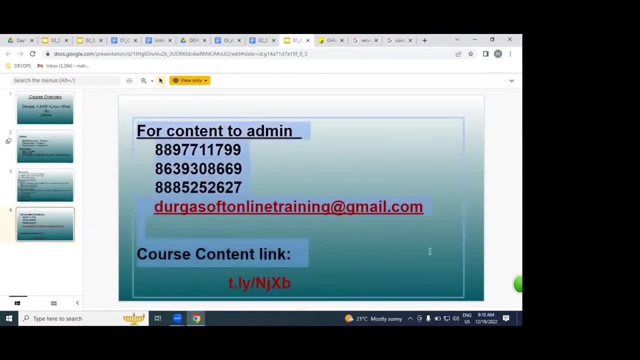 with what exactly? very basic level, finished with an advanced level, and each and every session is a practically oriented session. this is my admin information. it is my course content rate. I'm going to be share one more time in the chat box. please be, get it all of you. 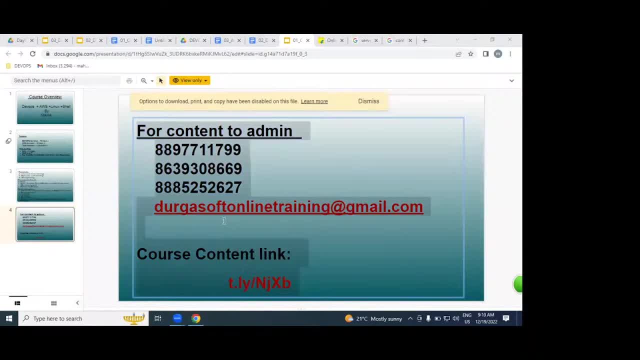 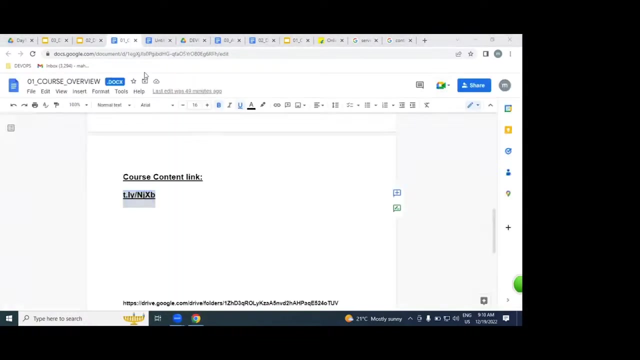 you, oh excellent, so please be get it so before taking our questions, please, before taking our questions, please for offline students, please be make it notice like a photo or note it spelling is: n is a calculator, whatever. so please make it. p dot, l, y, forward slash: n, j, x, b. n is a calculator, x is a calculator. 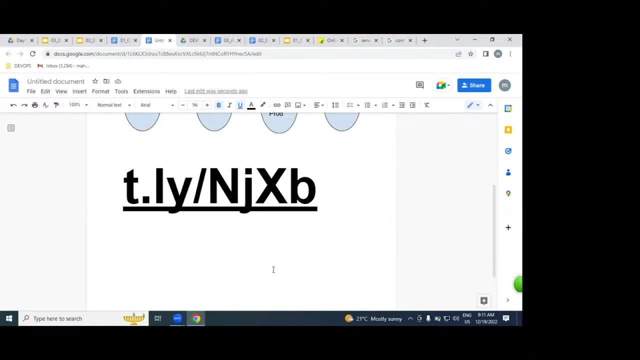 remaining, all are small: n calculator, x calculator remaining- all are small. so try to view and we'll meet them by tomorrow. so any questions, please, online students, please. Kumar have this question. so yeah, you can. so even telecom background also you can able to shift to to it, don't worry. so our class is very easy to understand, very slow, everybody can understand. 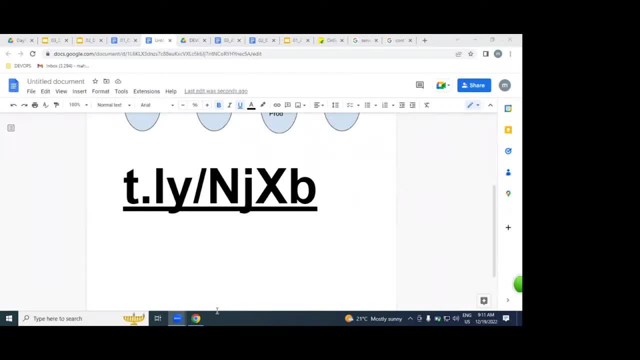 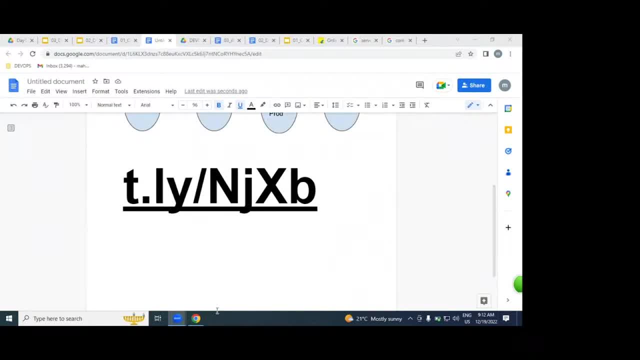 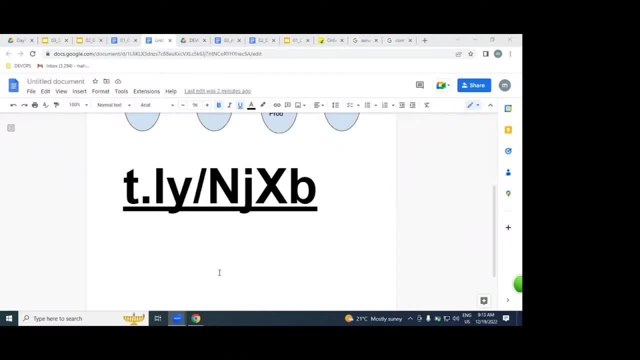 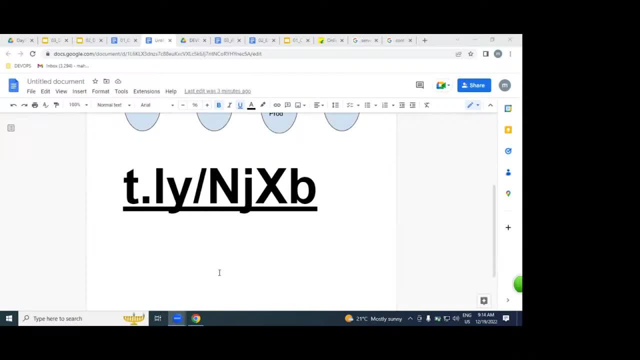 basket? definitely, yeah. is there any other questions please? all of you. is there any other questions please? so is two years of experience. guys got an interview calls so 2.5. i'm recommend 2.5. 2.5 to 3 more openings as of right two place also we have. but 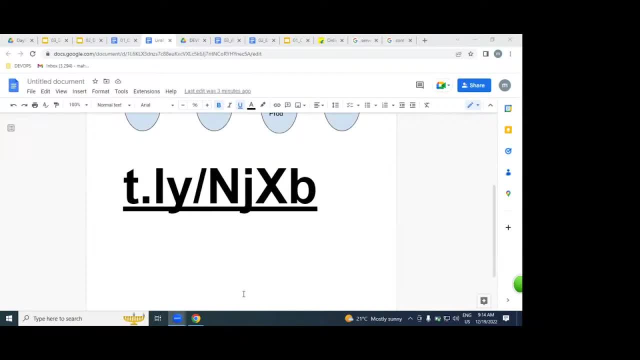 compared to three. less pressures also get a calls, but you know the ratio is. one example: experienced guy getting 10 calls for an example. maybe freshers can get four calls. four to five clubs, maybe after january- i'm talking about, not december- this month, soon, yeah, is there any other question please? online students. 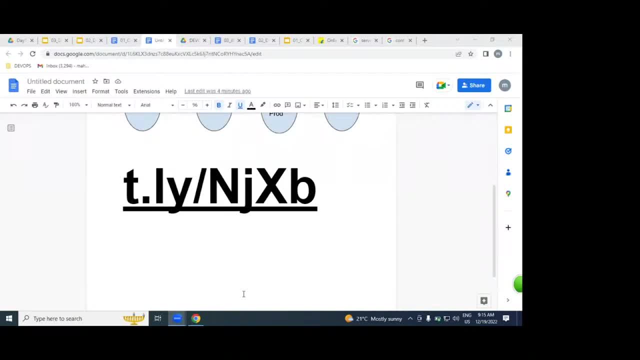 can you move to the offline? yeah, is there any questions? offline students, so you can practically explain. huh, hands-on means what exactly, for example, i will show you here only so, for example, on cancer, because i will show you in the live itself. i will show in the live example. 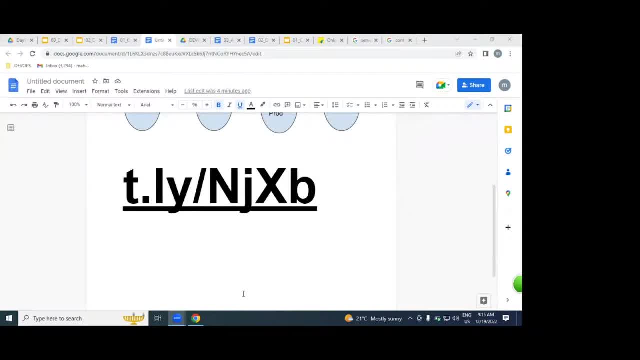 that is only simple example. for example, ansible how to write a playbook, how to execute the playbook, how to configure servers practically. i will show you slowly, class by class. that's what ansible it's three weeks will distance: ansible itself three weeks, chef itself three weeks, ci3 weeks and aws six weeks, so eight weeks again. 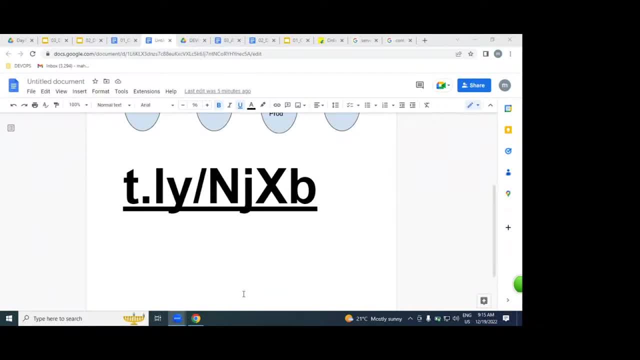 eight weeks or seven weeks, we're going to be discussing adbs. i don't exactly plus or minus one docker component one month, okay, why? because of practical things. i don't exactly plus or minus more docker component one month, why? because of practical things. so we will discuss it by then. i'll definitely do that as well. 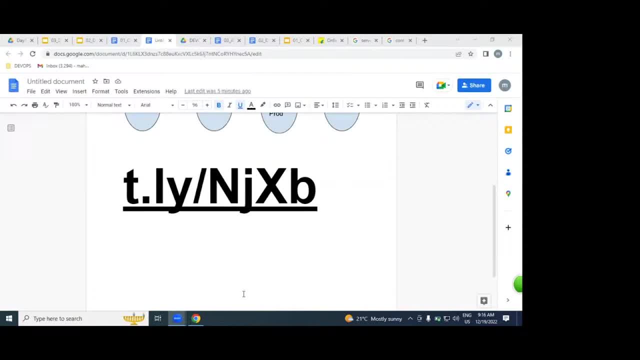 okay, so i'm going to be doing also. i should say after this video that if you wish to do because of practical things, each and every session is a theoretical explanation- we should understand the concept. then only if you show practically you can understand directly. go for practical nothing and that is a blur hands-on. so project also example answer. what is answer? 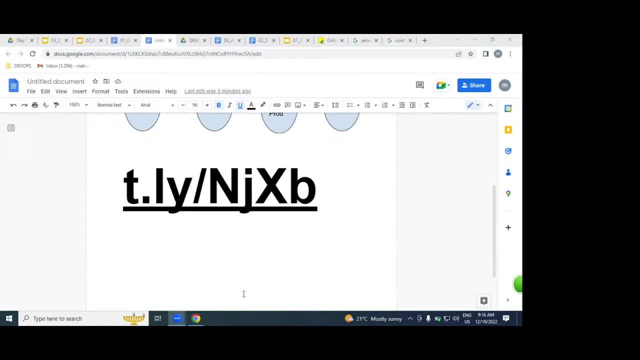 why we're answering. we should understand. so, day by day, slowly, we are going to increase each and every concept through all the functionality. what are the features? in answer, we're going to be discussing practically every day, practical by end of the session, by end of the model. we'll do. 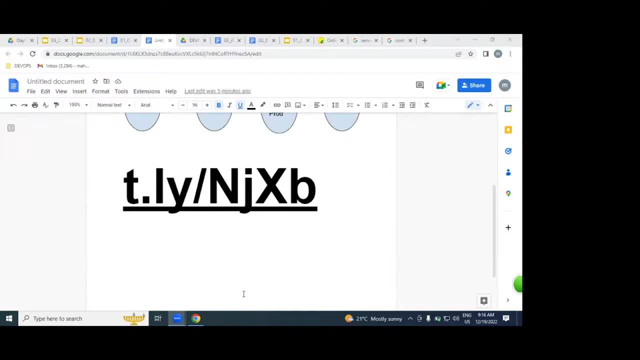 one real-time project on a model in aws, in devops. four modules there. that means four projects ansible. one project cacd, one project docker and kuban, one project chef. one project so complete, one cacd pipeline. this is the reason. that's what it will take. 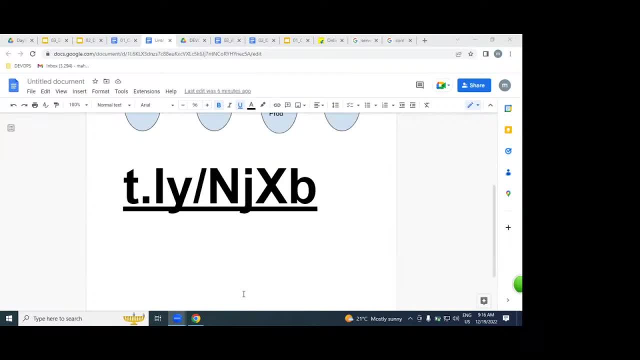 time. so if you want to complete this course, one month is enough, theoretically, but it is not. that's what it will take: four and a half months to five months, we know. four and a half month- that's what classes mean- means it may take one class or month. so time is not concerned. for me, time is not a concern, but we need to. we need. 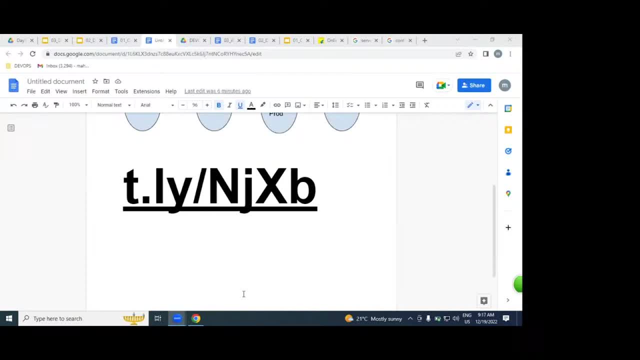 to complete and practice what we are given content. that is my answer, but i am not too good, but also comfortable. one second: How much experience can I have after this course? You can show up to 4 years. You can show up to 4 years by this course. 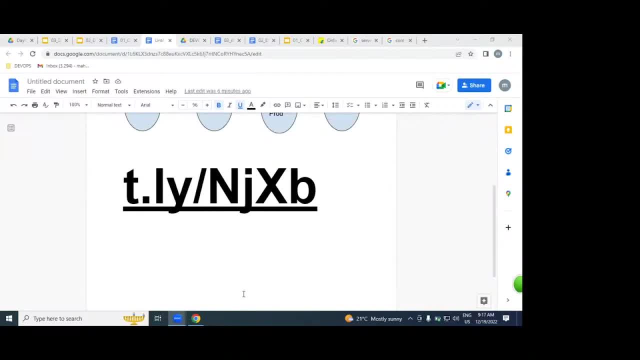 What is the question, please? Okay, For example, your name, please Rajesh. So Rajesh had this question. So I have a 10 years of experience, 11 years of experience, 11 years of experience. I have already Okay. 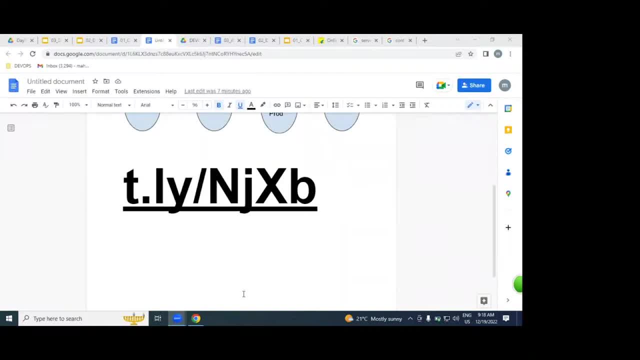 How exactly we can able to show this, please, How exactly we can able to show I have a totally 11 years of experience on IT In resume. From last 3 or 3 and a half years onwards I am working as a developer. 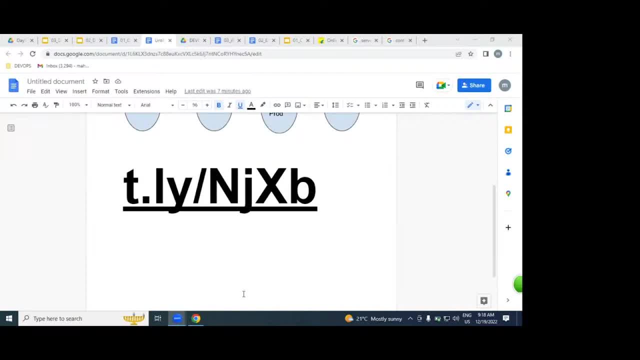 You can show like that, But how exactly convince I am working as a, for example, XO is a technology like NET or Java or whatever Internally. so my project, my project, in the project we got, we got an opportunity to work as a dev option. 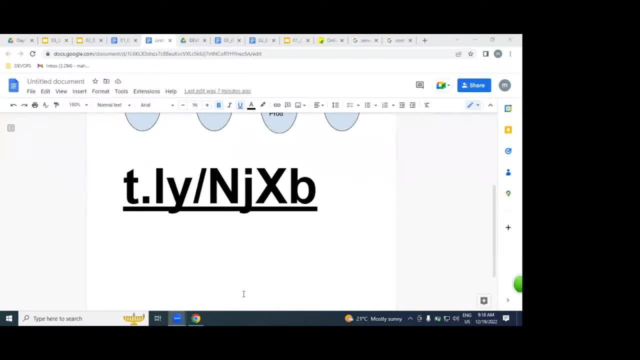 That's what I transfer Depends. We can convince It is possible. So this course is not only for freshers, not only for experts in both- Even 15 years of experience or 20 years of experience Java architect should learn this course. 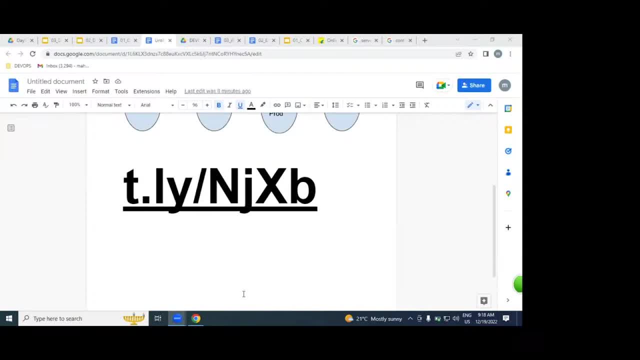 There is no exceptional for that Option, not optional and should be learned. Even VP, vice presidents of the company or a senior manager or senior architect, who are all working in top position as software. There is no option for them. They should learn DevOps. 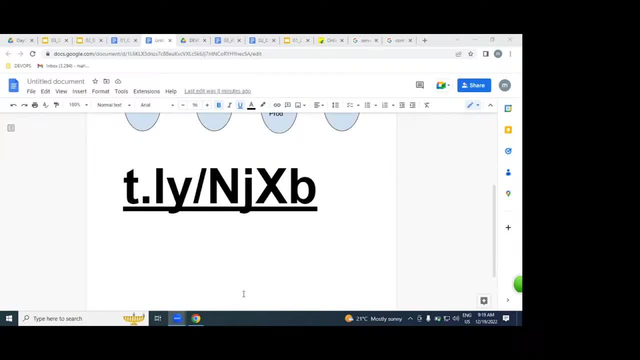 Even freshers also Understood very clearly. Anybody should learn. Even testers should learn this Developer, for example. you join as a developer- Java developer. Last maybe 2 or 3 years and work there. You join as a developer. last maybe 2 or 3 years and work there. You join as a developer last maybe 2 or 3 years and work there. You join as a developer last maybe 2 or 3 years and work there For him also. 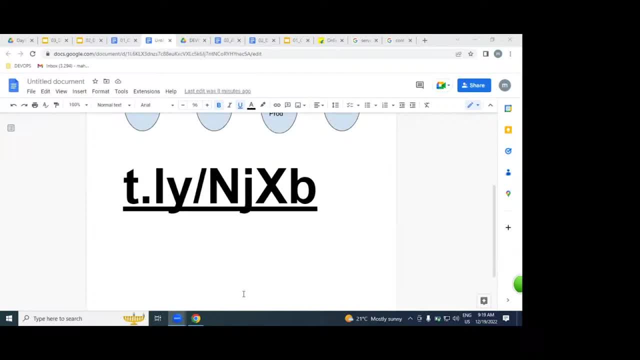 there is no option to learn it. You should learn DevOps. If you are a developer, there is no option for you. You should learn this course, Whether you want to continue as a developer. whether you want to continue as a developer. 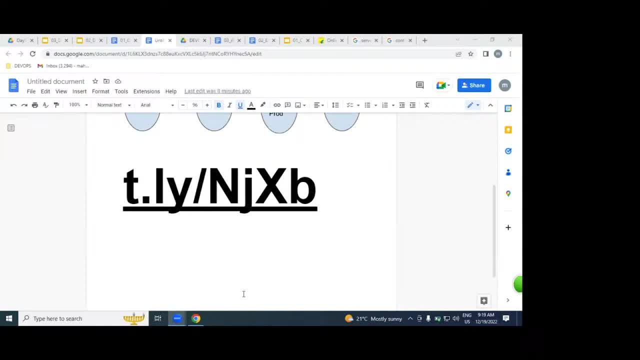 that is the second thing, Even testers also, Even if you are an admin, an infra-type side. So, no question about it, You should learn this course. Fine, All of you understood very clearly. So one more thing: compare to developers. 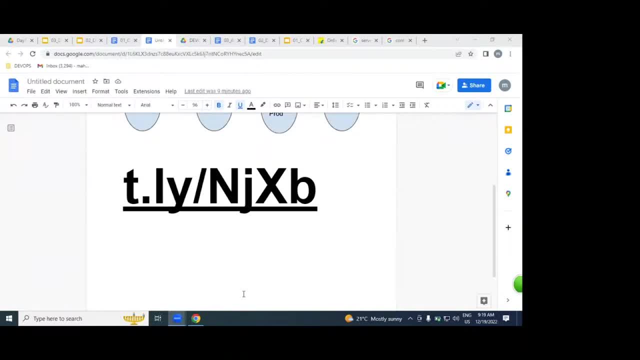 more package is here. Compare to developer. more package is here. If you are getting a more package, more work. If you are getting a more salary. that means we need to affect more, We need to mentally, we need to prepare for that. 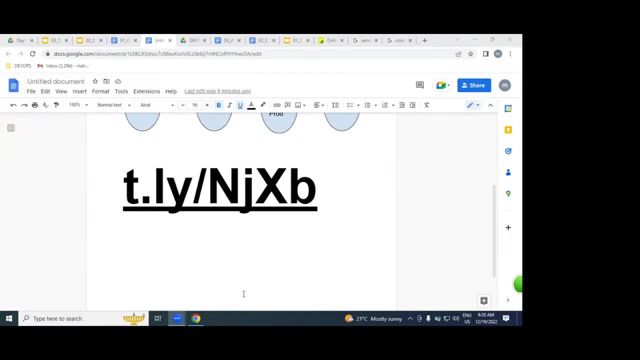 Mentally ready for that. We are working for money. Okay, please, please, keep on the mind. So we need to hard work. We need to hard work If you do practical what I am delivering in the class, if you do the same class. 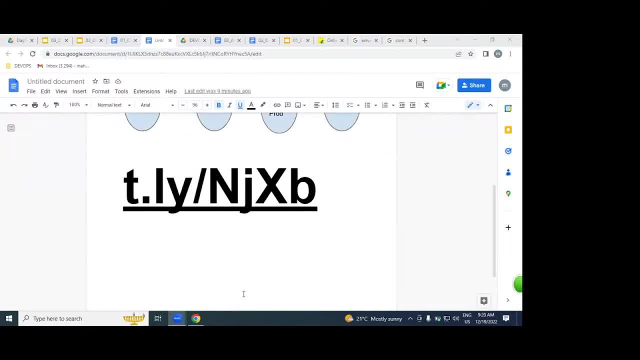 same. if you practice, it is more than enough for getting a job. So you have to promise before joining in this course: practice One hour class, two hours minimum practice per day. It is more than enough. So that's it for today. 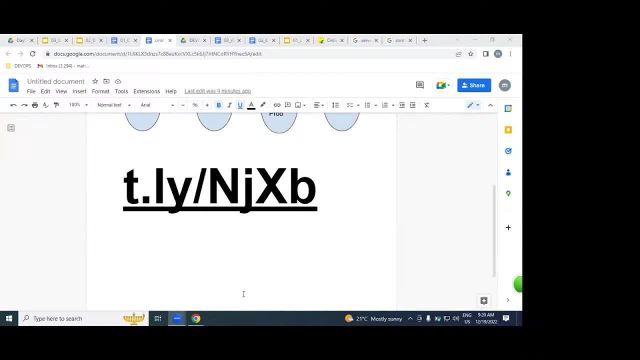 So we'll be continuing by tomorrow, Please, Sir. this course will not depend on coding, sir. It's depending on coding, But we're not learning coding. We're handling Java, but we're not learning Java After writing code. 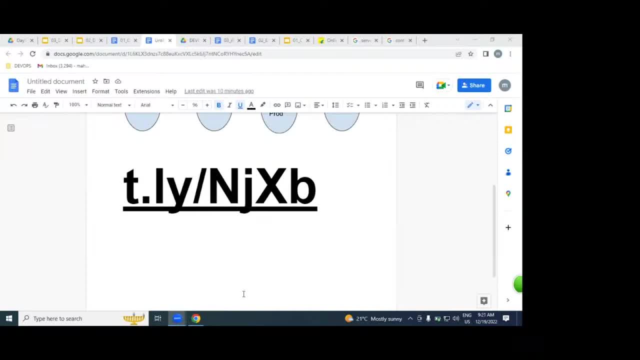 we need to handle the coding, We need to handle the code. That means we're not writing any code Understood very clearly. Some scripts are required, Formats are required. I tell you, I will teach you guys. Maybe I'm a Ruby. 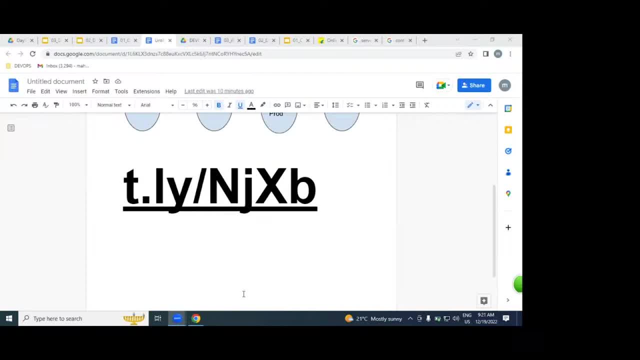 Maybe maximum we are going to be using if condition, If you know very well, If Maximum, Maximum, Yes, Nothing, See, see nothing. If else, data stacks are nothing again. No data types in no variable. 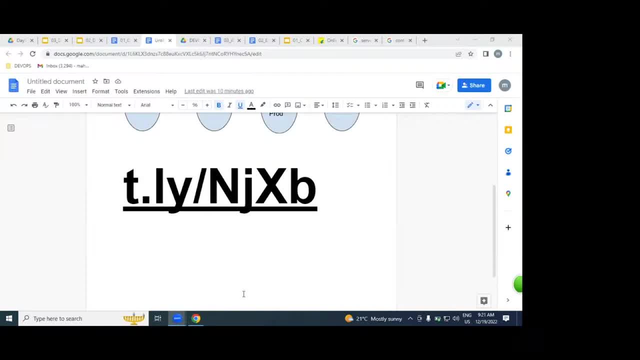 Variables we are going to be using. That is also string type only. No, not required. Python is not mandatory, but it's if you want? yeah, If you want? yes, But what's the problem? You know if you are keeping Python on. 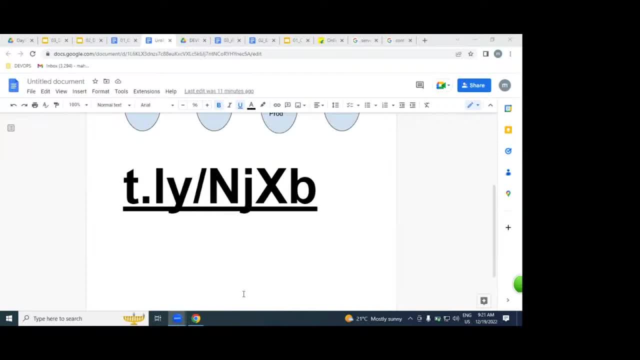 Python with DevOps, you know more of it is We can't handle after getting it. That's the reason. So, as a beginner, as a fresher, as a, so getting a job, as you're looking for a job. Python is not not including you, But after getting a job after three years. one year, if you sit down as a DevOps, then looking for Python, Python with DevOps After getting a job after three years. That's very clear. 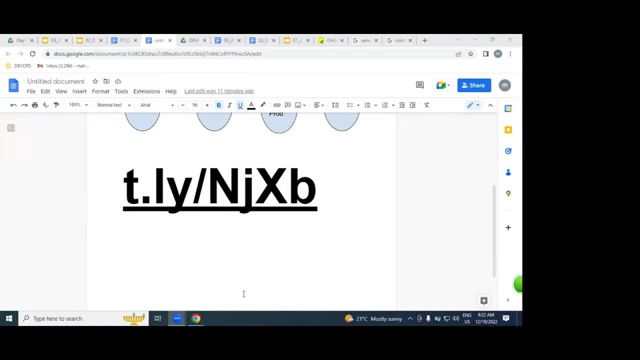 With this combo, what will happen? you know. after getting a job, You become a scientist. Understood very clearly Means what: There is no time for your family. You are dedicated to the company, Dedicated to the project, No personal life. 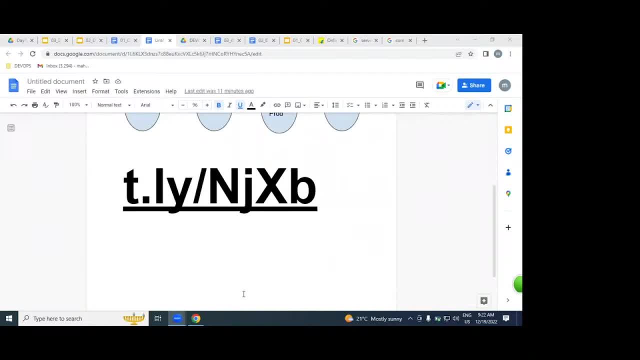 That's what I'm not recovering. Without Python also, we can happily get a job. We can continue. There is no problem. It is an option, Thank you, Thanks, guys, Please. We'll be continued tomorrow. If any questions any doubt, don't worry. 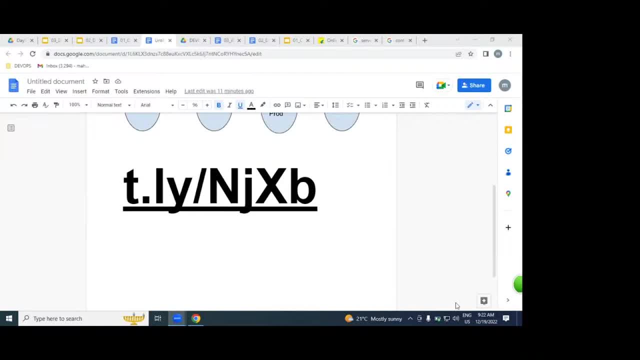 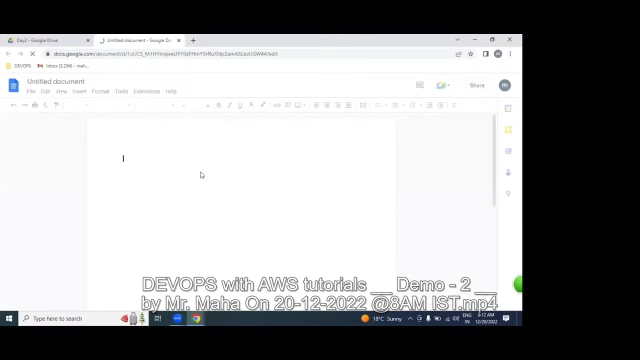 We'll meet tomorrow again We can discuss. Thank you, Thanks, guys, Please Thanks. We'll be continued. Bye. what is aws? that is in exactly our agenda. okay, but in std we have discussed. what is devops? okay from new students? we have. that is the reason. so what we are going to be guys first. 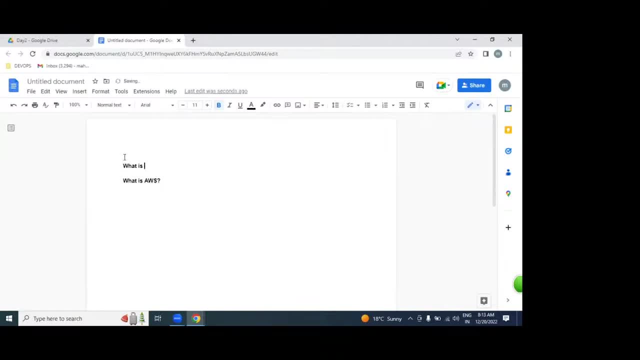 so we are going to be discussing about first- just worry of what we have discussed in the last session: what is devops. then we will discuss about what is aws and by, and we can conclude, we can understand. so what is the difference between aws versus devops? this is in exactly. 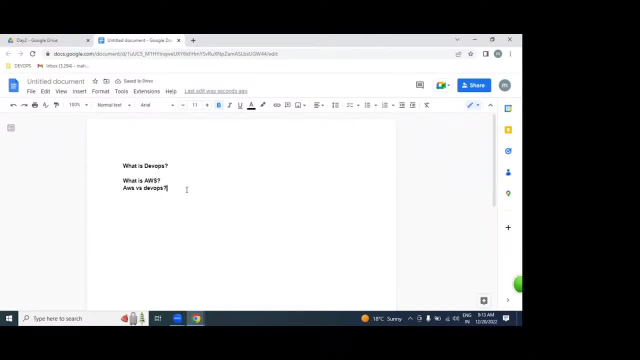 our agenda for today. understood very clearly, right you? so, before starting our session, before our starting our session, guys, please, before starting our session, please. so online students audio video: everything is perfect. can you confirm in the chat box once all of you audio audio is clear, can you confirm in this chat box, please? 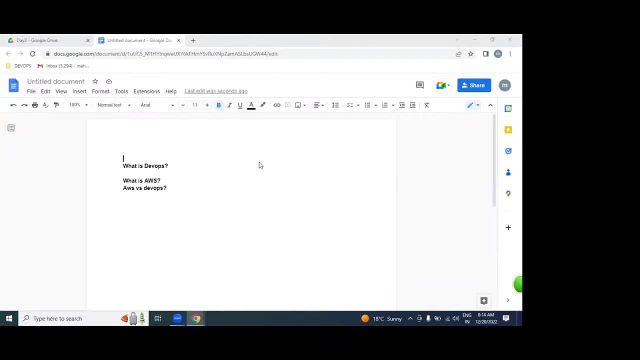 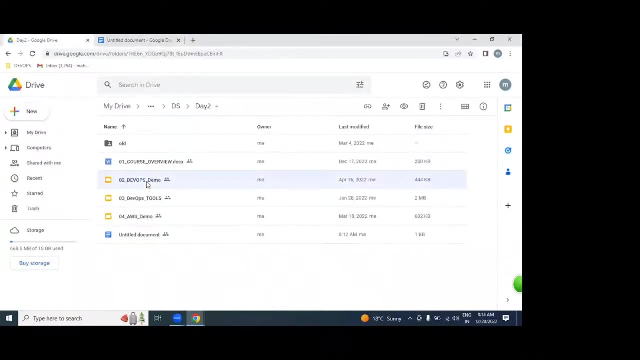 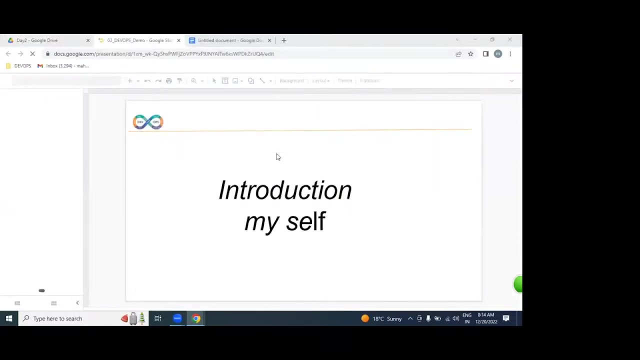 all of you please once. thank you. yeah, if any problem, please let me know in the chat box. okay, in the middle also. fine, fine, thank you. thanks for replying, all of you. let it be content, okay, so first. so let me introduce myself. so my name is maha. i have a totally. 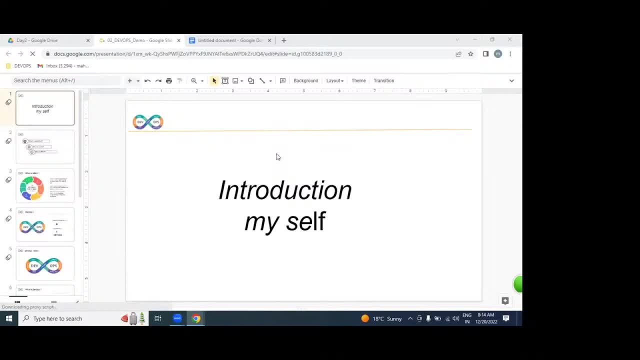 15 years of experience in IT. My career starts as what Java developer. My career starts as what Java developer. From last five years onwards, I'm working as a senior DevOps engineer. Senior DevOps engineer as well as AWS and Azure also. 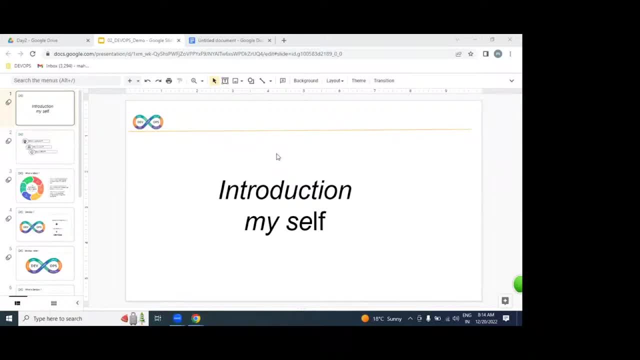 This is exactly my profile, So before starting this session. so I'm going to be asking you three questions, please. What are these three questions, please? What is the first question? Anybody help me? What is application? What is the second question? 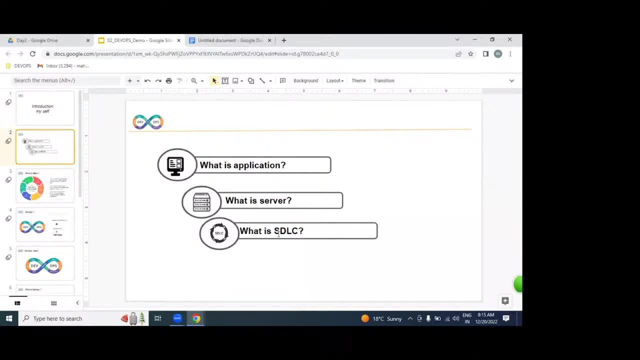 What is a server? Third question is: what exactly? What is SDLC? Is anybody help me? What is an application, please? What is an application, please? Anybody help me please? The working software which is written, any programming language. 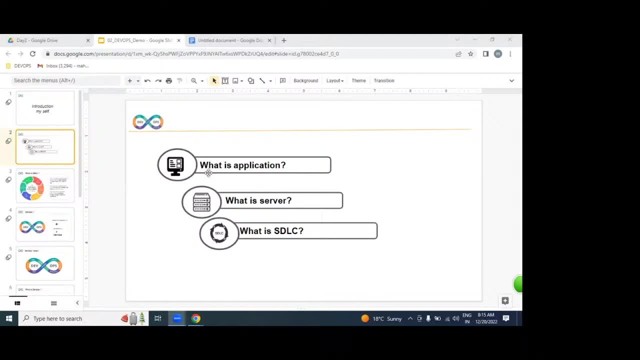 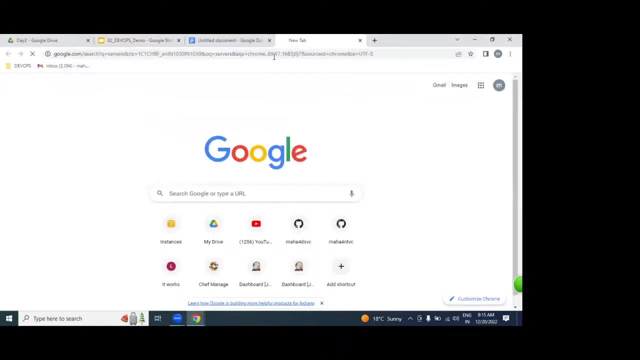 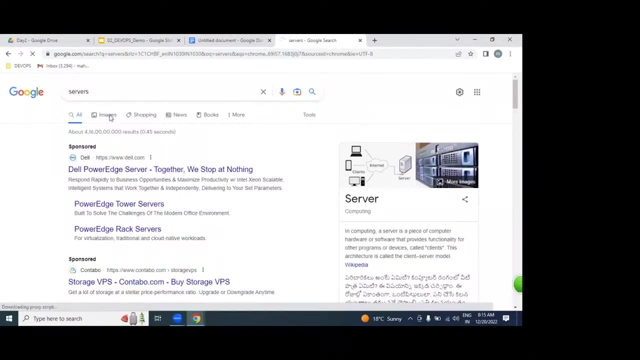 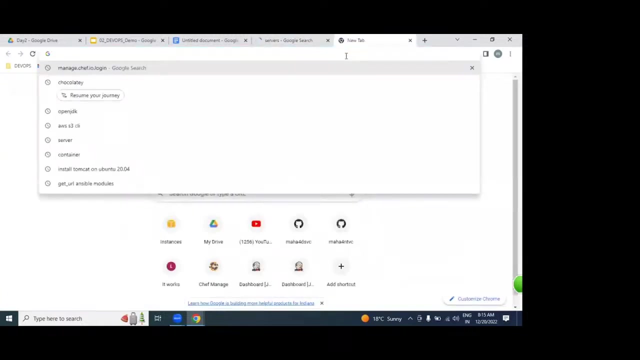 Like Java, NET, Python. we call as. what Application? That application we are going to be placed on server side. Once if it is placed on server side, once if it is placed on server side, you are going to be accessing as a website. 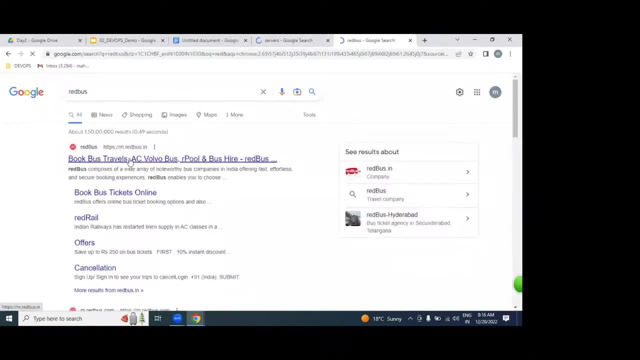 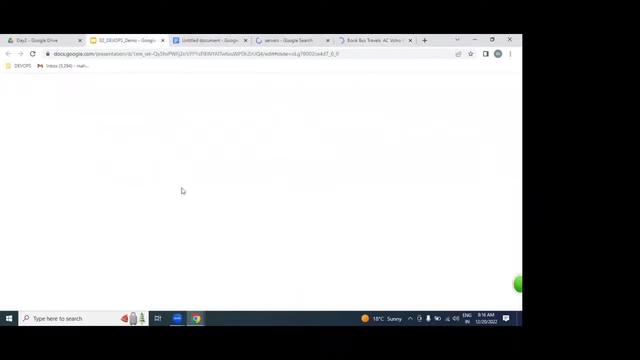 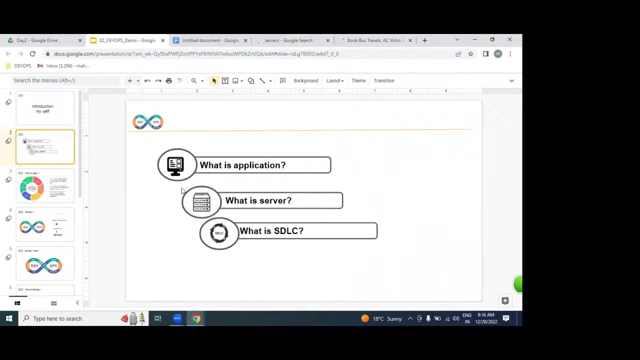 like a RedBuzz, BookMyShow, IRCTC, Flipkart, any website. What is an application? Anybody help me? What is an application? Anybody help me? Application is nothing but a website. Simple answer: Application is nothing but a website. 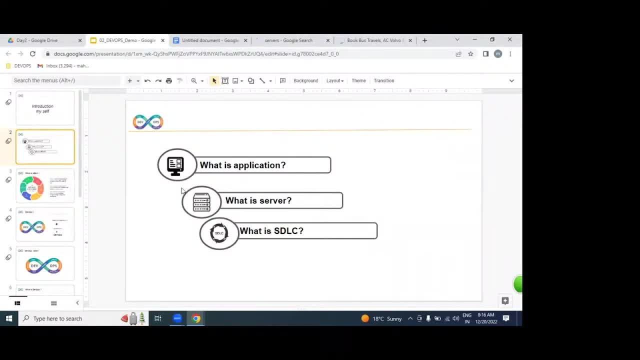 That is simple answer. You always remember when I call application, please, please remember, is a website. If it is called a definition point of view, application is nothing but a website, The working software which is written any programming language like Java, NET, Python. 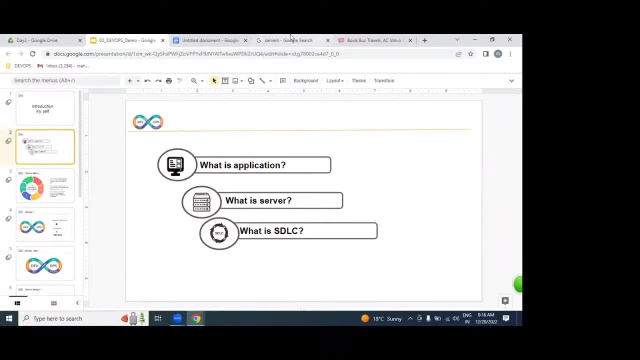 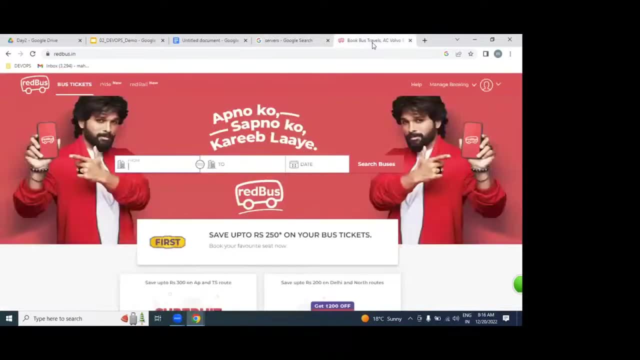 we call as an application That application. we are going to be placed on hundreds of servers. Once, if it is placed on hundreds of servers, we are going to be accessing our internet, our internet as a website. This is we calling as what. 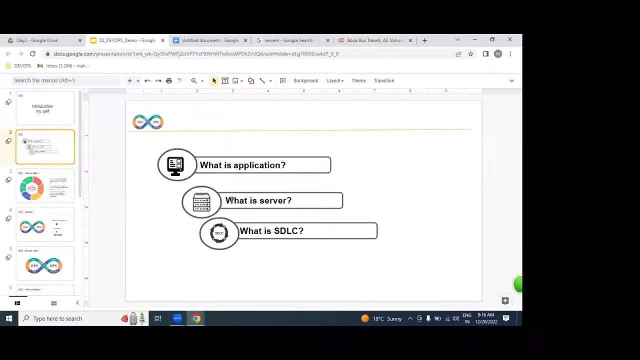 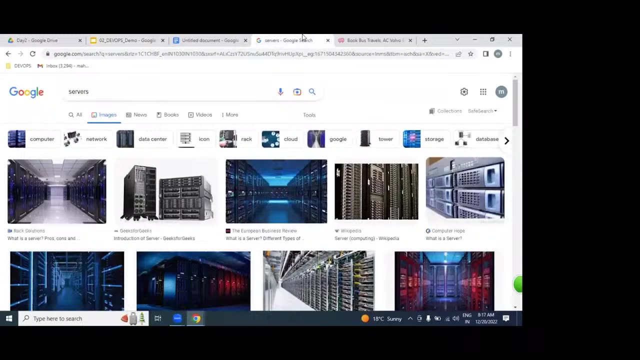 Application. But what are the server? What are the purpose of server, How many ways we can able to get a service. So we can able to get a service, either physical environment or a virtual environment or a cloud environment, But so any server for deploying our applications. 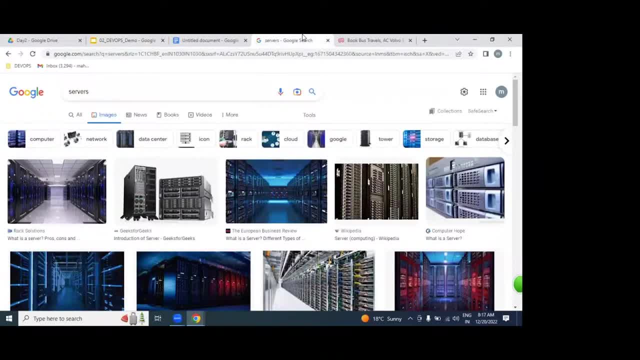 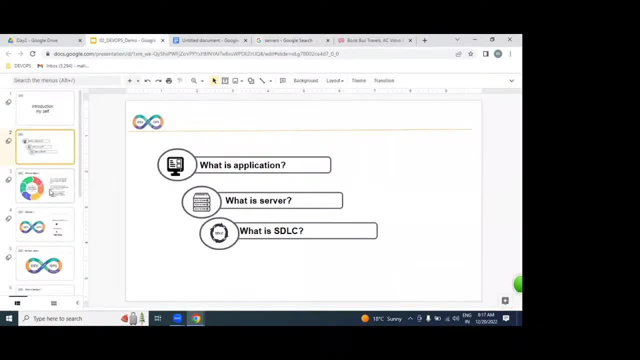 to maintain our applications 24 hours for a long time without any shutdown. So this kind of service we're going to be having. And what is an SDLC? Anybody help me? What is an SDLC? What is an SDLC? 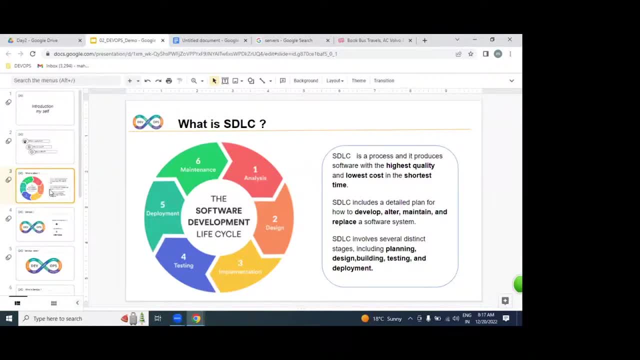 Software Development Lifecycle By using SDLC, what we can able to do it. Anybody help me? We can produce websites By end of this SDLC. we are going to produce what Applications? That application we are going to be placed on server side. 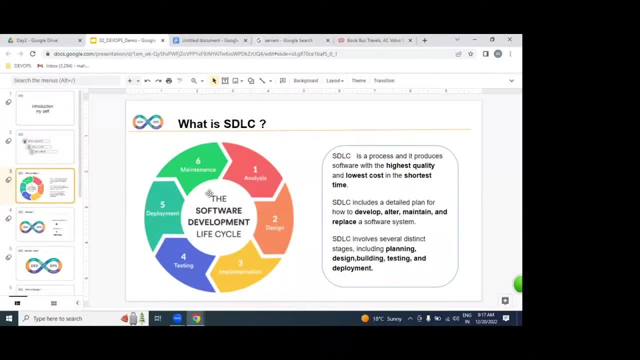 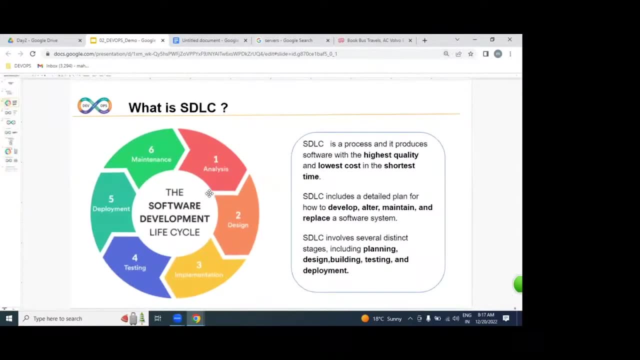 and we can able to access. But in SDLC we have several stages and several phases, Several stages and several phases. Which are all the stages, guys, Please? analysis, design, implementation, testing, deploy and maintenance. So these are all the stages. 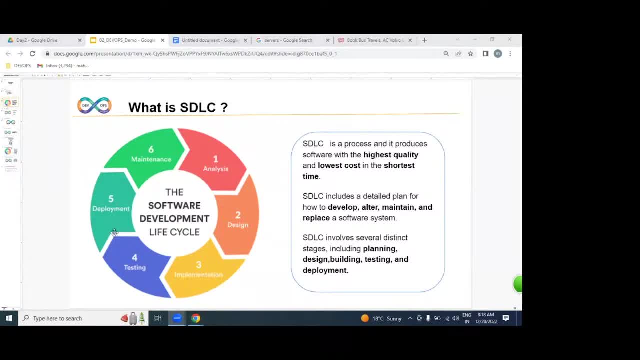 By following these are all the stages- we can able to produce a website means application. How exactly, guys, Please, how exactly we are going to be? Analysis is nothing but what. Gathering information from the client, For example, if you want to construct the house. 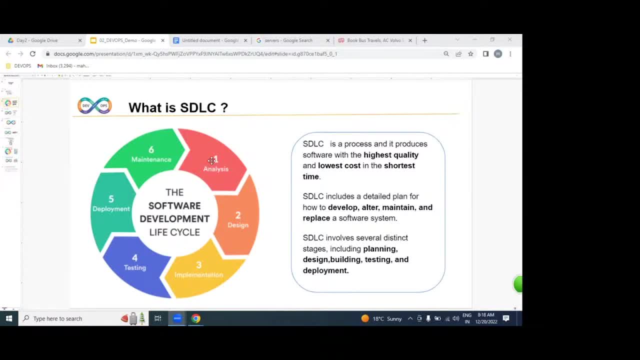 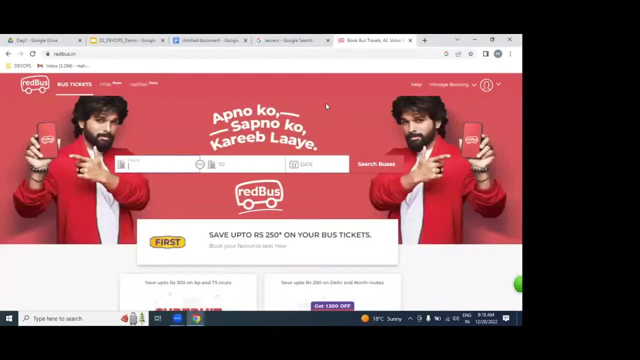 we need to gather the information or not? Iron cost, cement cost, land cost, how much required? what is everything we need to gather information or not? The same way. so how exactly this business? it is a travel business. How exactly this business? what kind of business? 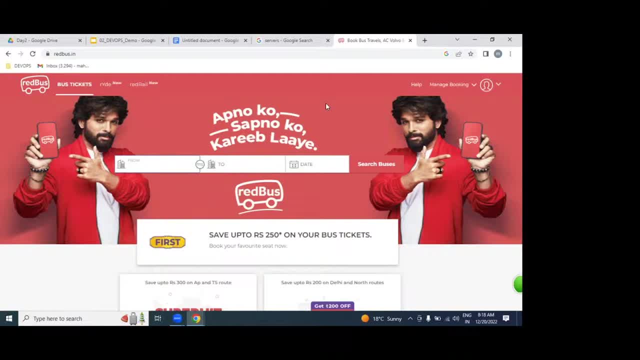 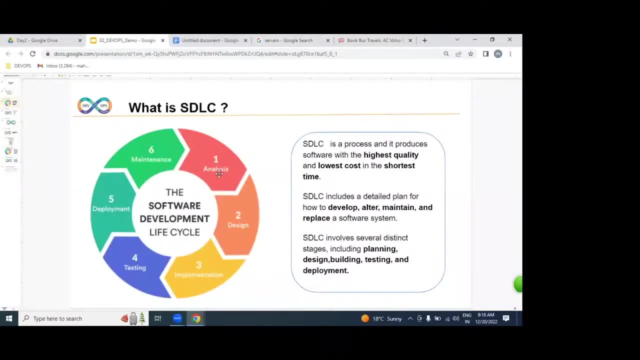 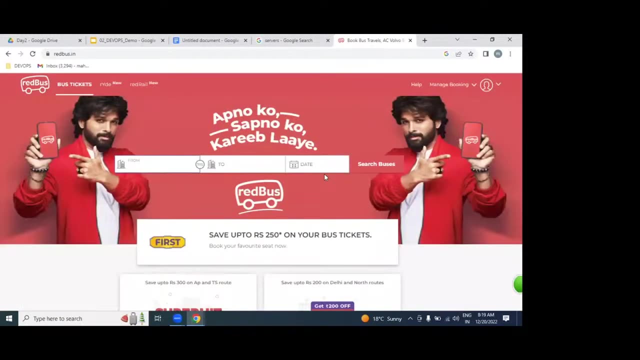 what exactly client the business owner is expecting. So, as a BA business analyst, we are going to be gathering information from the business owner is nothing but a client. How exactly it's going to be login page. how exactly it is registration page. 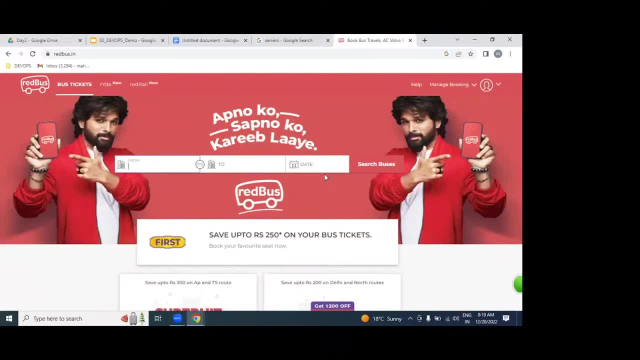 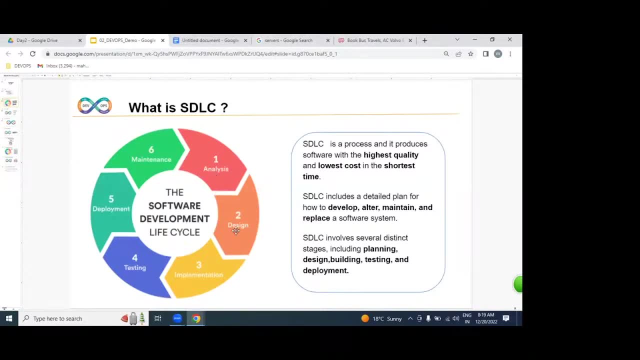 how exactly it is dashboard, which technology. Each and every information will be gathered. After successfully gathering information, our architects will be designed. Our architects will be designed. Architect is going to be planning. design is nothing, but what Plan? So to construct the house, we required a planner. 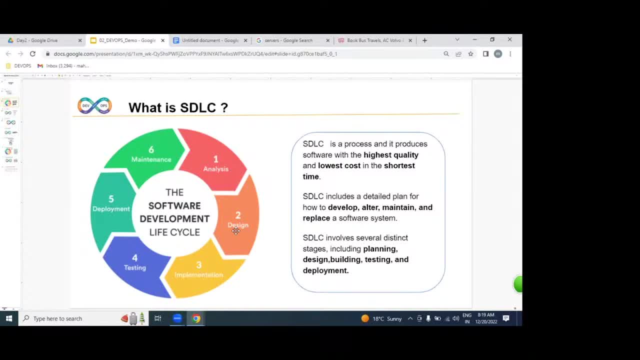 Double bedroom, triple bedroom apartment. Without plan, we can't be construct the house Same way. according to the plan, our developers will implement. Our developers will be implement software by using Java or NET or Python, whatever. After successfully implementing, after successfully implementing software. 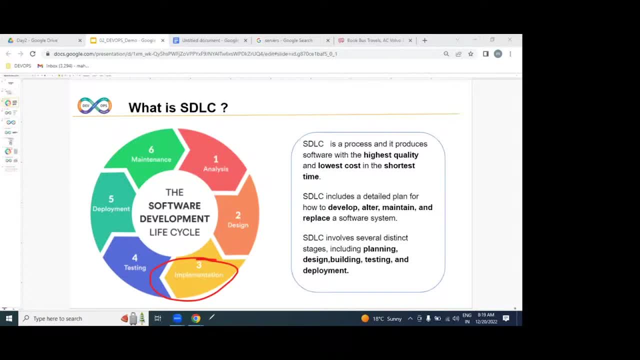 whether the software is good or not, whether the software is going to be working, whether the software is going to be, whether the software is going to be working or not. our testers will be verified by using an automation test cases, manual test cases or performance test cases. whatever, 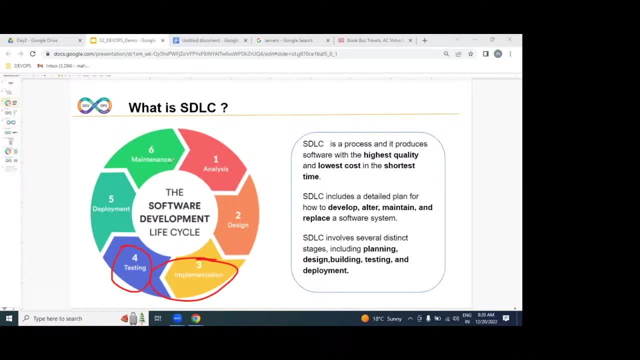 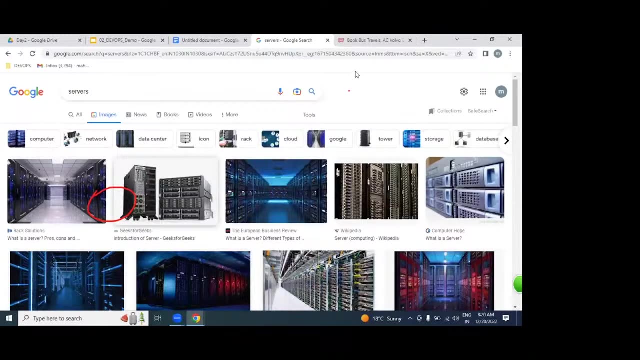 Once if it is verified, we are going to be deploying on hundreds of production sets. Once if it is placed on hundreds of production sets, production servers, we can able to once if it is placed on access over internet and website. That's it, no. 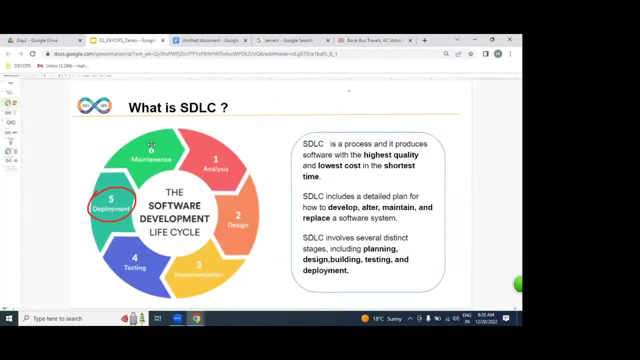 So, whether it is working or not, we are going to be monitor and maintenance This entire process. we calling as what SDLC, SDLC. In SDLC, each and every IT employee involved, not only DevOps engineer, it is AWS Linux administrator, developers, testers. 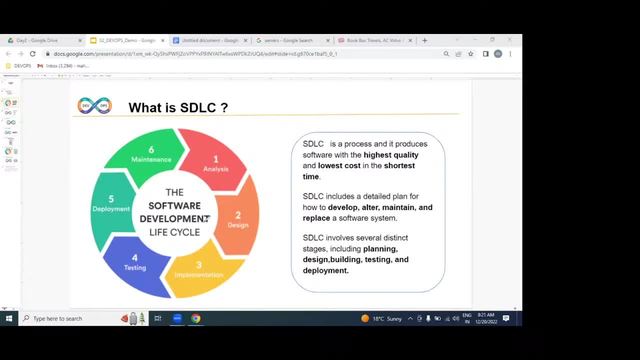 We are all together as a team. We are all together. We as a team. we are producing a website, Like our cricket team, like a movie makers. all together, All together If you want to make a movie, So actress required. 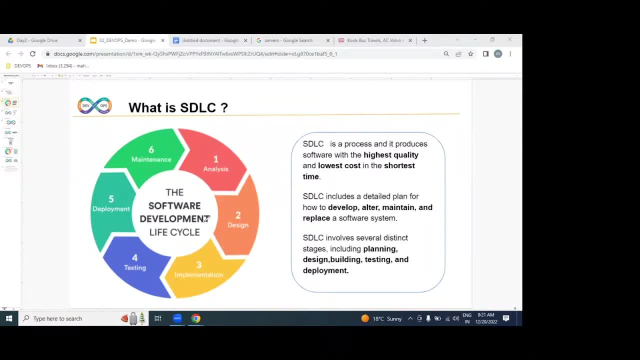 Heroes, actress, editors, Actors required, understood very clearly. and so many 24 crafts we have, i'm right, but here is actors are what developers, but director is devops engineer. understood very simple, we understood here. but by end of the day, any it employee, the developer or the tester or devops engineer, 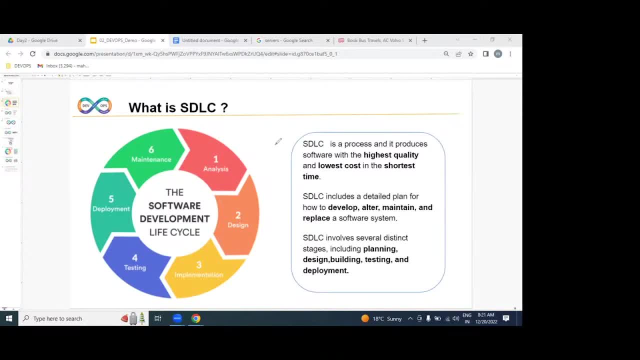 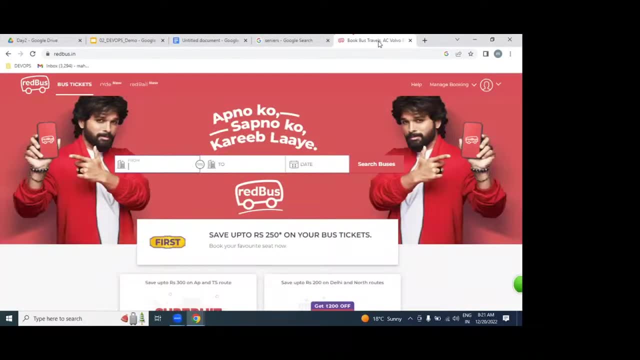 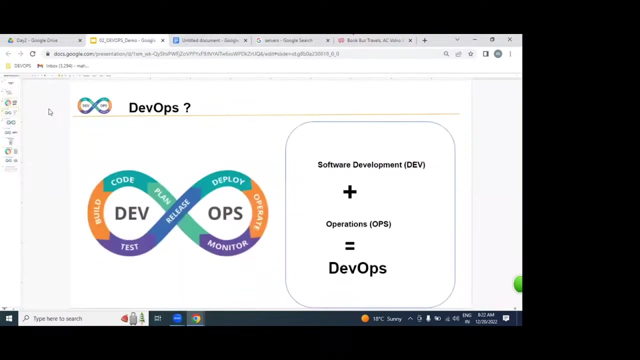 we have to produce an application to do business in online. by end of the day, any it employee, his goal is for what? produce a working software as an application so to doing a business in internet. that is what exactly, sdlc in sdlc, we are going to be. 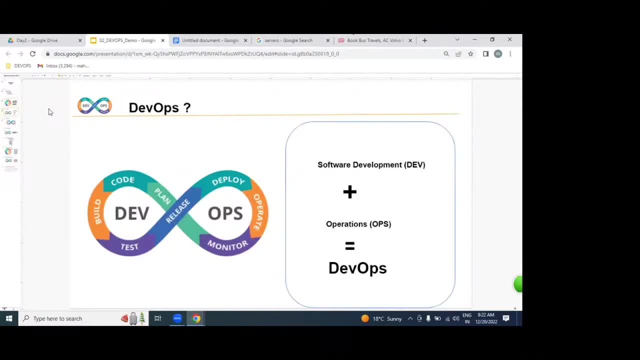 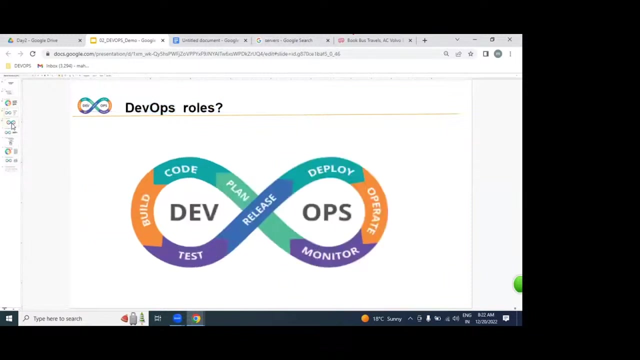 implementing our devops process on sdlc. we are going to be implementing our devops process. what is the dev is nothing but what. development ops is nothing but what. the combination of development plus operation we call as what the web scene. that means what? exactly? what we have understood? that means what we understand. guys, please, our roles and 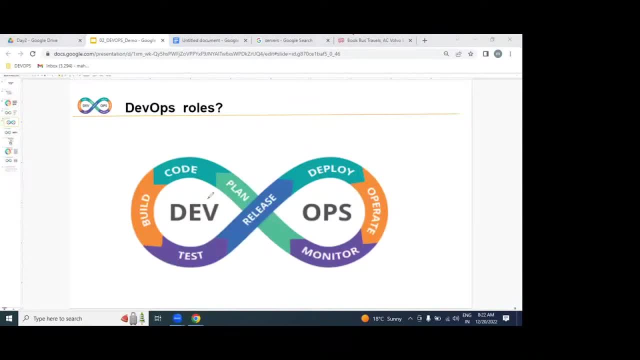 responsibilities start from where devin brawn ends with where operations- that means we are part of coding- build, test, release, deployments, apply, operation. so our roles and responsibilities from coding to production environment. that means: are we going to be writing any coding? that means: are we writing any test cases? no, we are not. 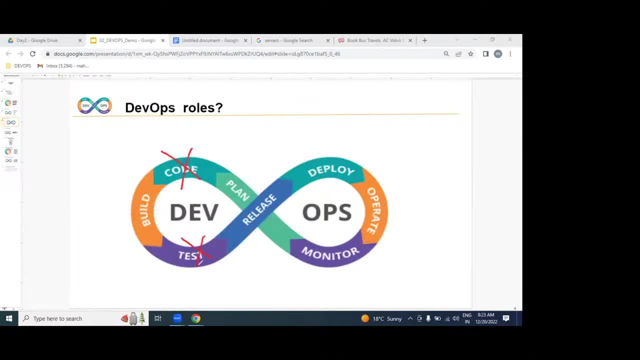 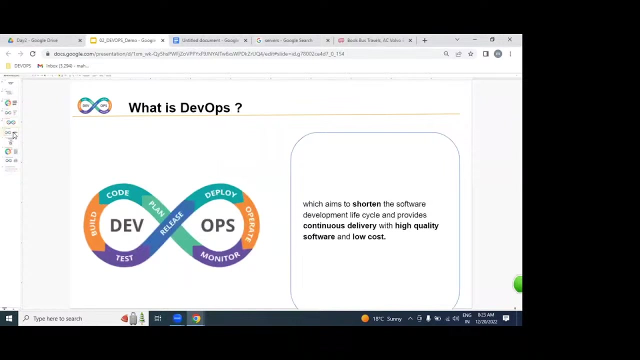 writing any coding. we are not writing any test cases, just we are going to be in implementing an automated devops process from dev environment to production environment. that is exactly our roles and responsibilities. what is it? what is it? devops is devops. is the technology? no, like javanet python: no, devops is a process. the verbs is a process which is going to be. 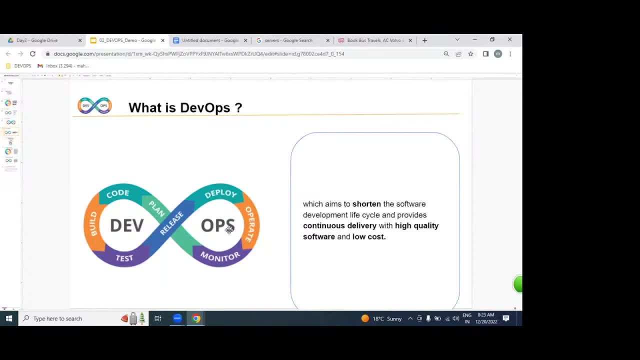 implementing from the environment to operation. but what exactly it will happen? developers writing a software or not, lines of code by using javanet, python or not, that code we are going to be the devs we are going to be placing in from the environment to production environment, while we